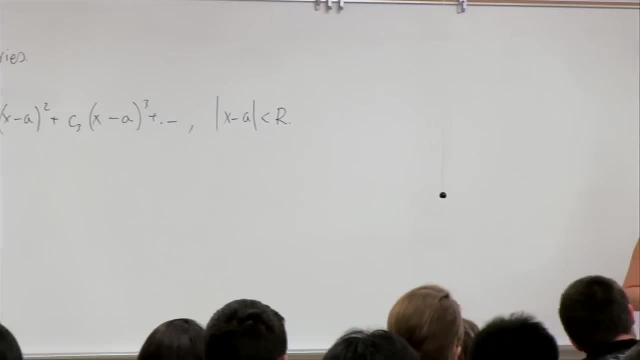 number of terms. So we have a radius of convergence. And we have a radius of convergence, So we have a number of examples of functions that can be represented as power series. Remember the first one that we kept coming back to? It was 1 over 1 minus x. 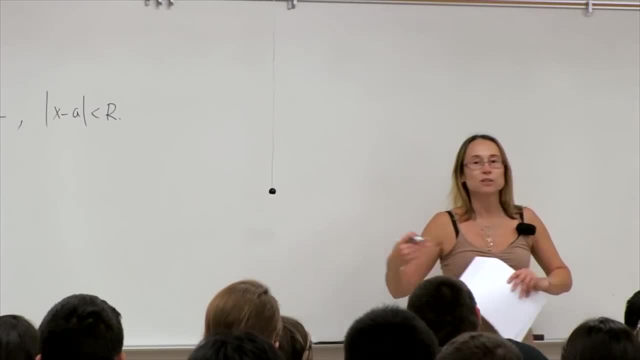 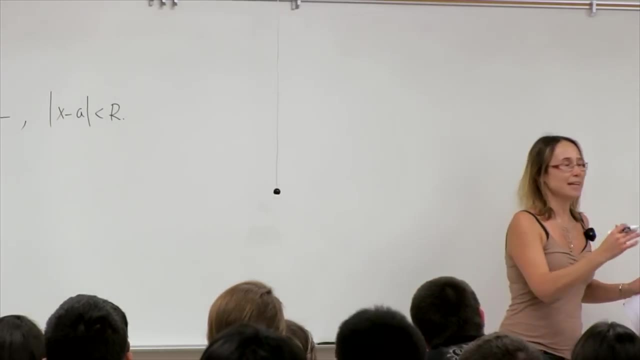 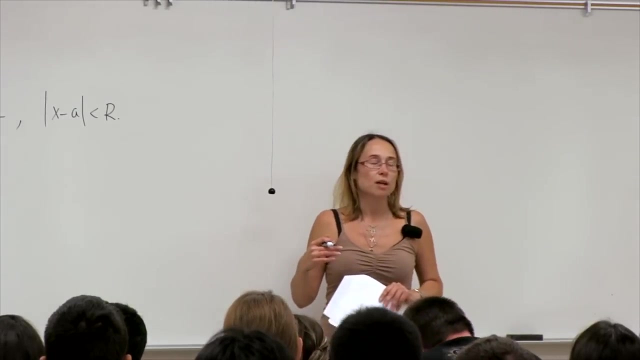 And that had a nice power series representation. And the rest of the examples actually were some variations on the same thing. Either we replaced x with some other combination functions of x, or we differentiated, integrated it, and so on. A more general question is that 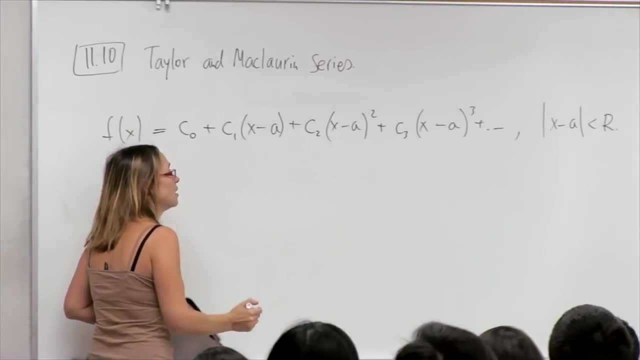 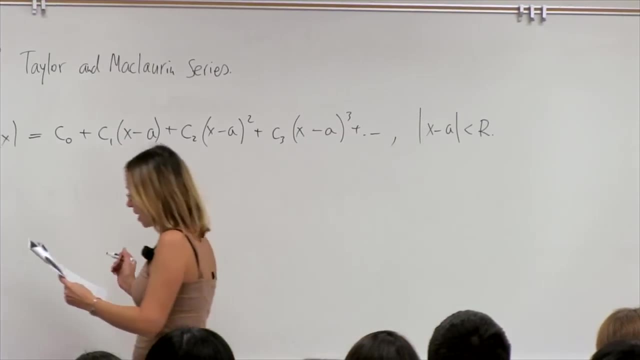 which function is the power series? Which function is the power series? Which function is the power series? Functions can be represented like this: and for what values? of x. right, We want to see how general this representation is. okay, So let's suppose that there is a function f that looks: 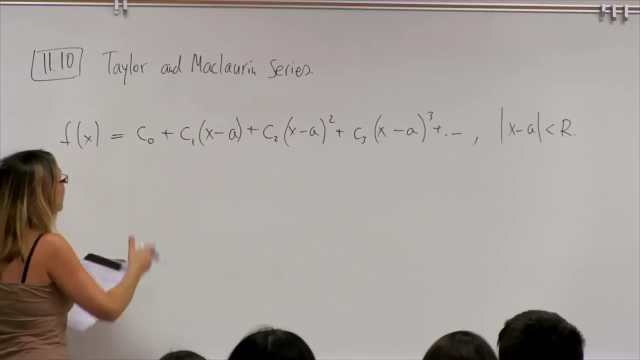 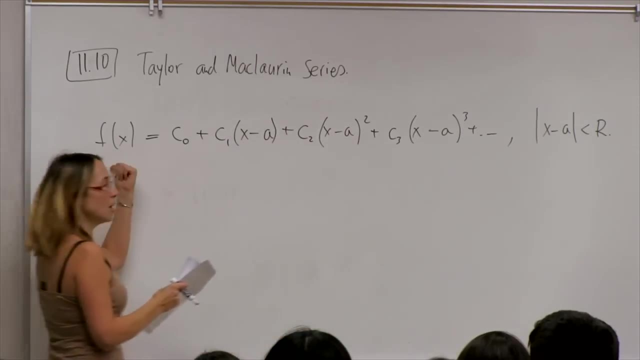 like this and try to find out something about the function f from the numbers c0,, c1,, c2, and so on. What do these numbers tell us about the function f? So the first thing we're going to do, we're: 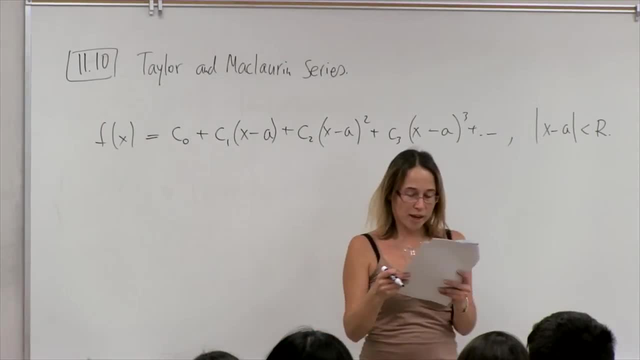 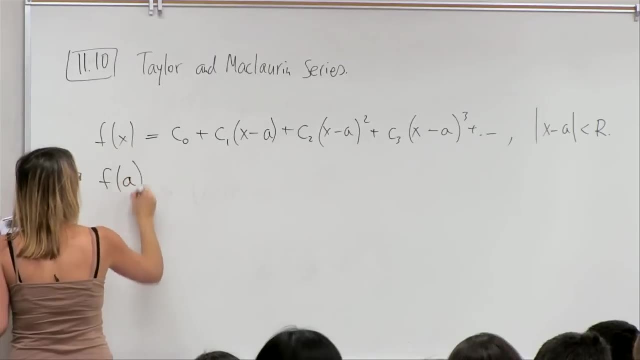 going to take this expression and we're going to take the function f and we're going to take the function f And we're going to take the function f and we're going to take the function and evaluate it at a. so we say x equals a. so on the left we have f of a right. 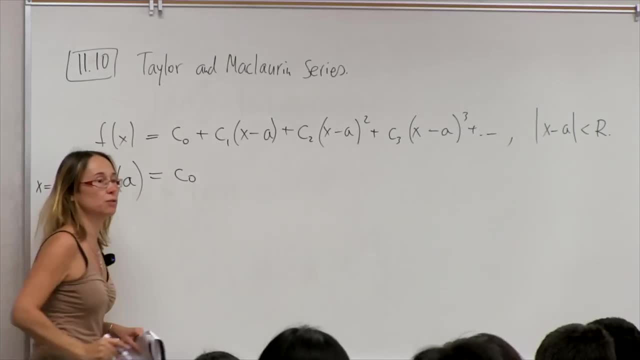 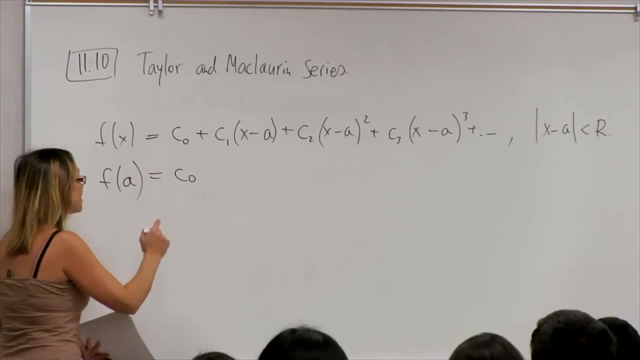 here we have c naught. what about the rest of the terms? they're all zero. so this is a nice piece of information. look, the first coefficient tells us the value of that function at the particular point, a. so this guy is responsible for the value of the function f at the center a. okay, the next thing I'm going to do, I'm: 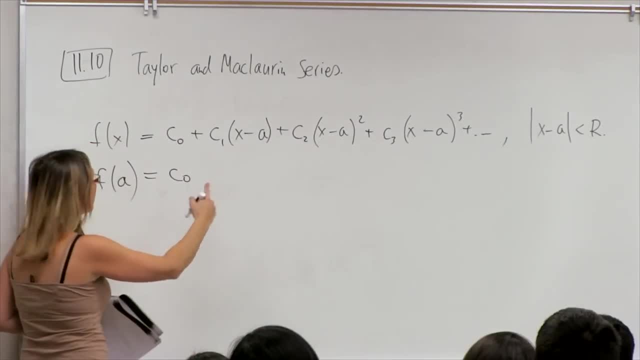 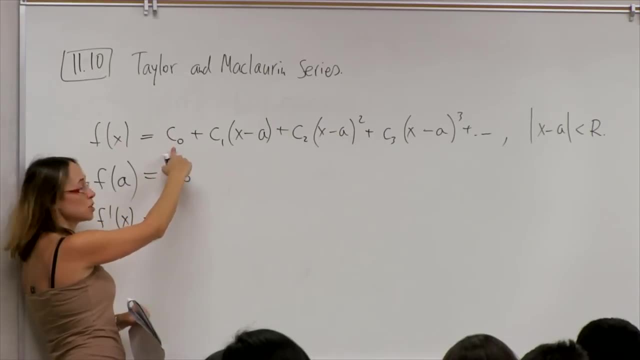 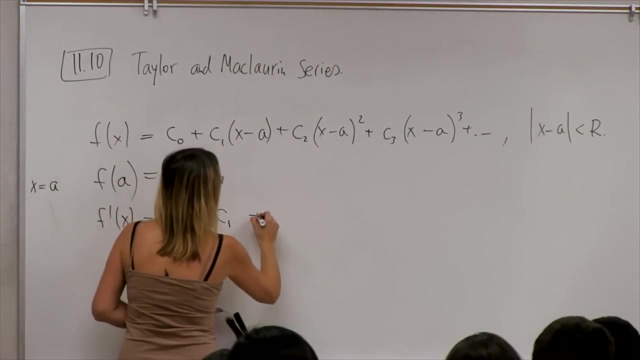 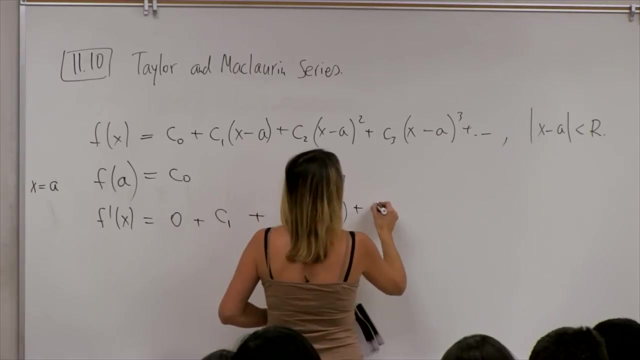 going to take this expression and differentiate it with respect to x, so f prime of x. when I differentiate it, c naught disappears. so this gives me 0 and I have c1. the next term gives me 2. c2 x minus a, the next term gives me: 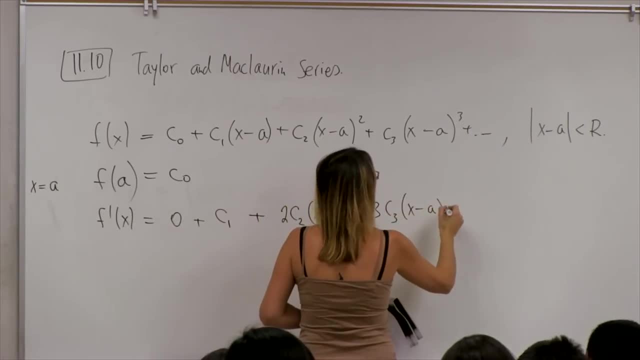 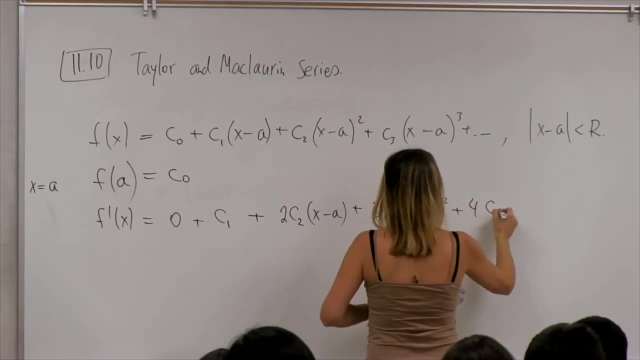 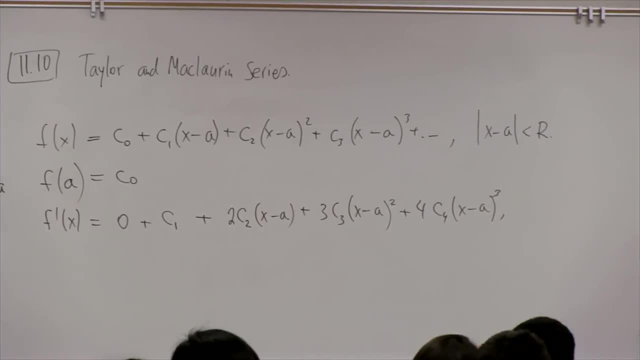 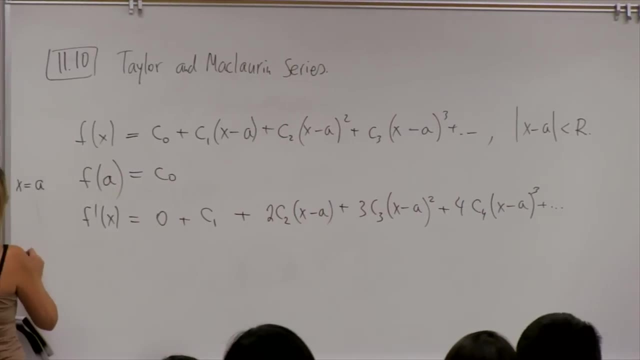 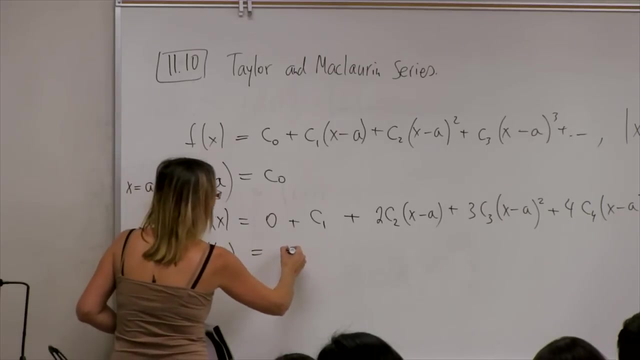 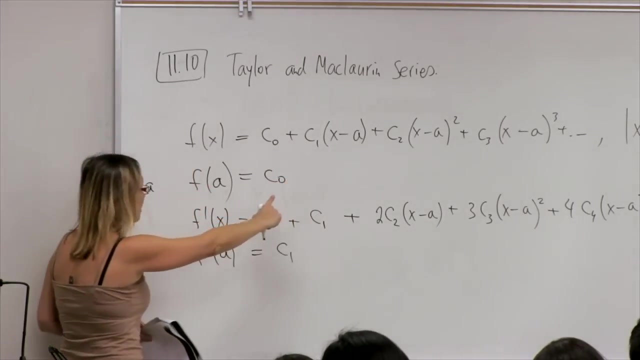 plus dot, dot, dot. Okay, how can I use this expression Again? let's set x equals a and evaluate this at a. So on the left I have f, prime of a. On the right I have c1.. How about the rest of the terms? Zero? So the second coefficient, c1, tells me the value. 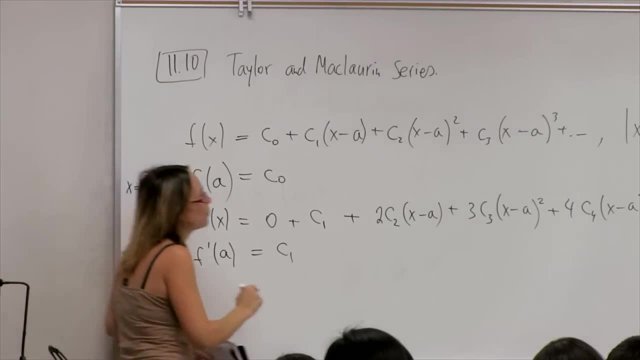 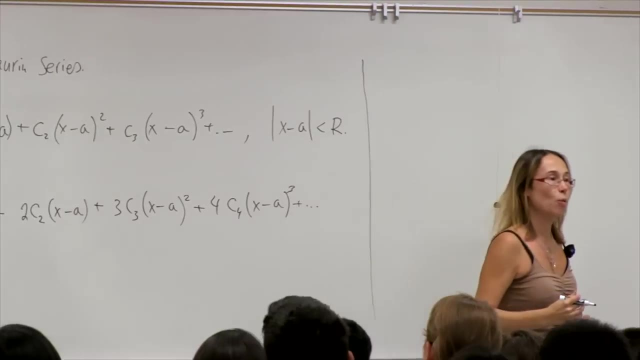 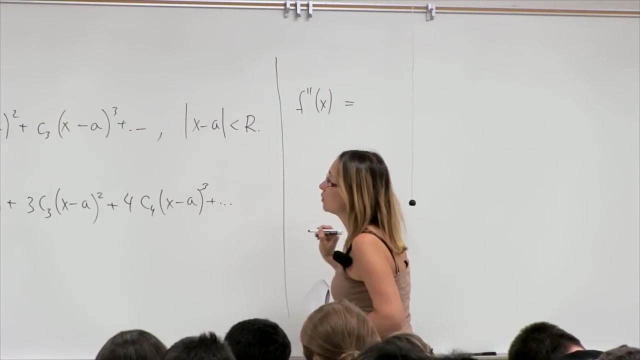 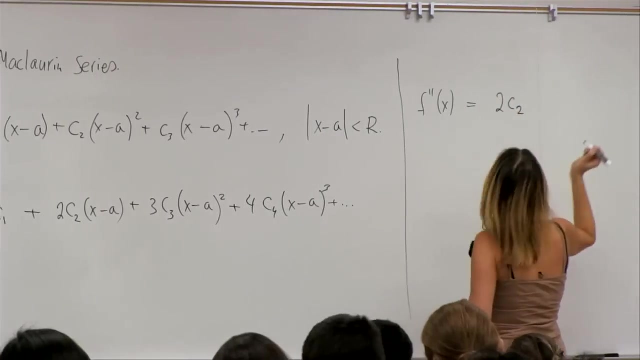 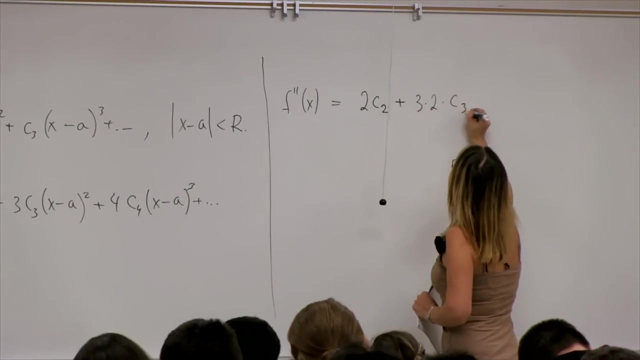 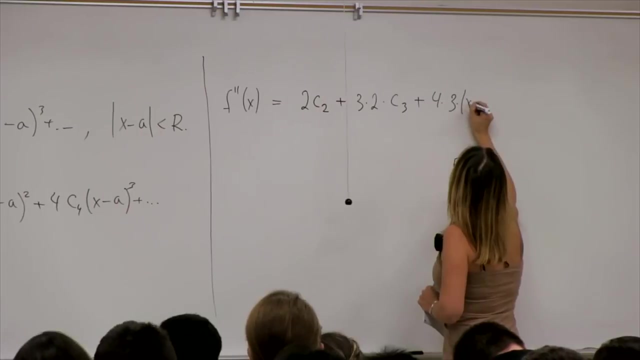 of the derivative of f at a Okay. Next, I'm going to take this expression and differentiate it once more with respect to x. So I get f prime prime on the left And on the right. this gives me zero. This is 2 c2 plus 3 times 2 c3, 4 times 3 x minus. 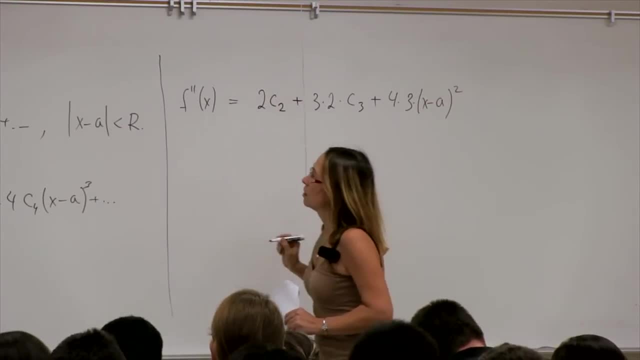 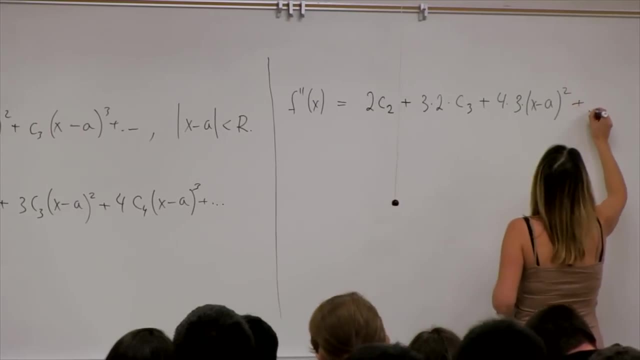 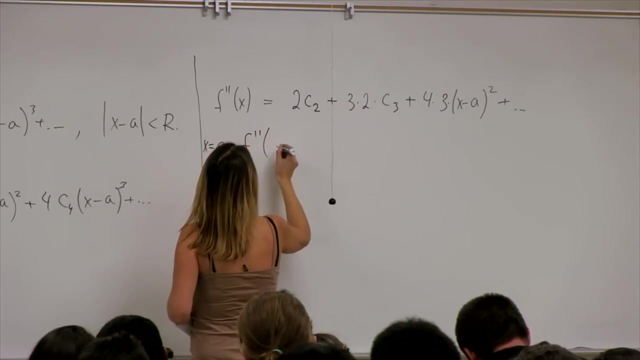 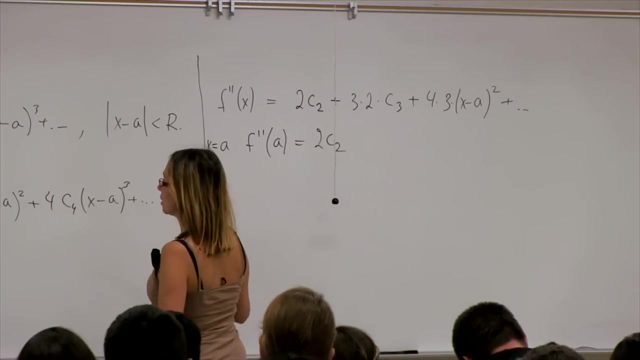 a squared and so on. Okay, Using the same procedure, take x equals a. What do I get? F prime. prime of a is equal to 2 c2.. Oh, something is wrong. It should be an x minus a term after 2 times 3 c3.. 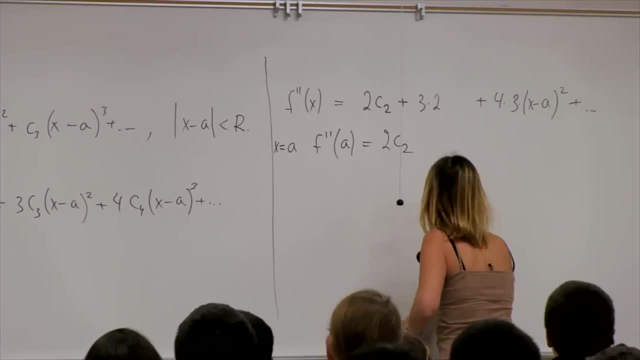 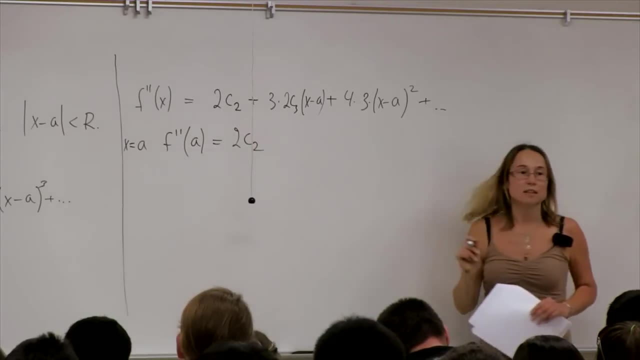 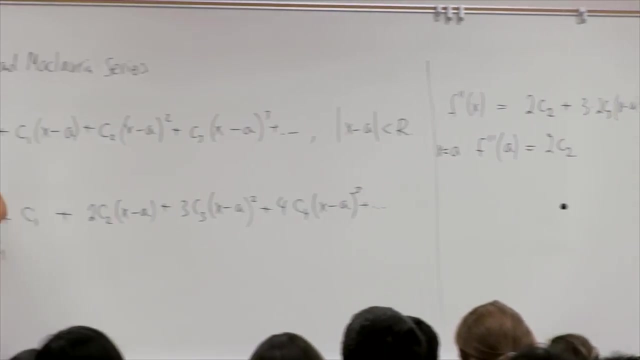 Yeah, c3,. yes, x minus a, Thank you. Okay. 2, c2, and the rest of the terms is zero. So we thought we'd guess the pattern right. We thought that each coefficient tells me the first, the second and so on. derivative. 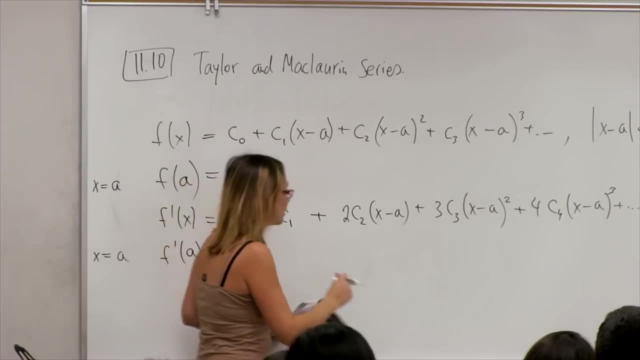 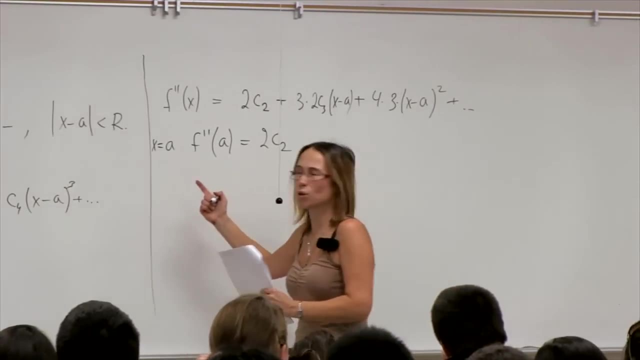 of the function f with respect to x. at point a, Not quite. Here I have a factor of 2, so I have to do a little bit more work, okay, Because I don't know what happens. So let's do the third derivative. 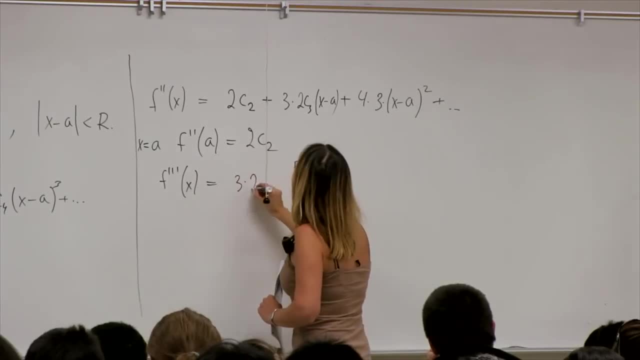 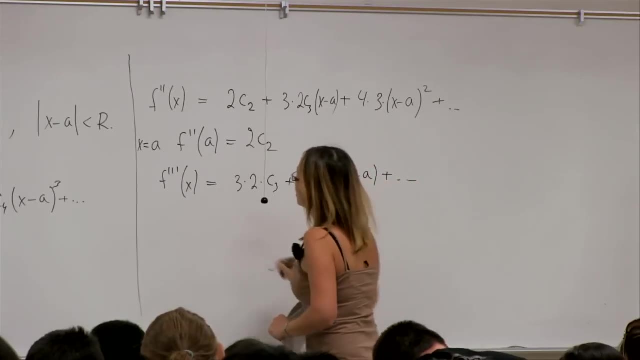 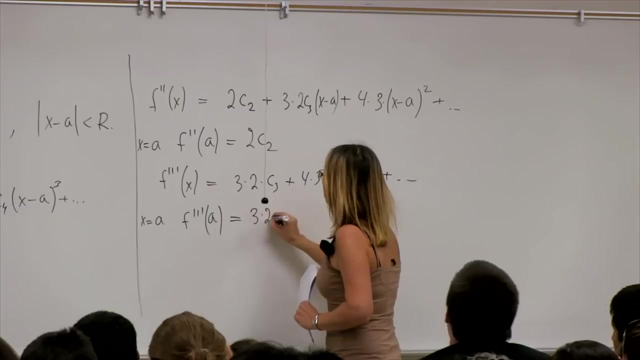 And I have to take this expression, differentiate it, Okay, And evaluate it at a. So the third derivative at a is given by 3 times, 2 times c3, and the rest of the terms do contain a power of x minus a. 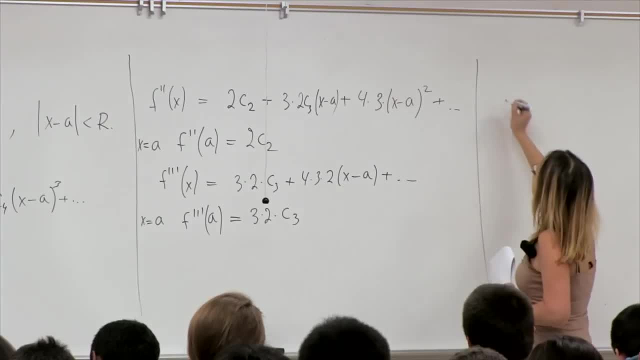 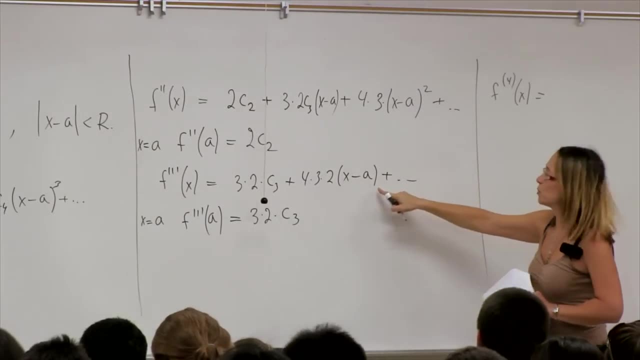 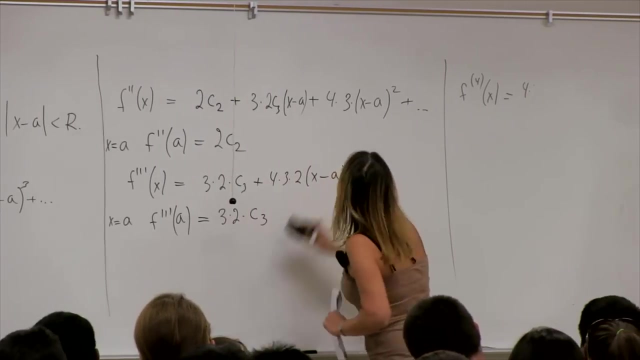 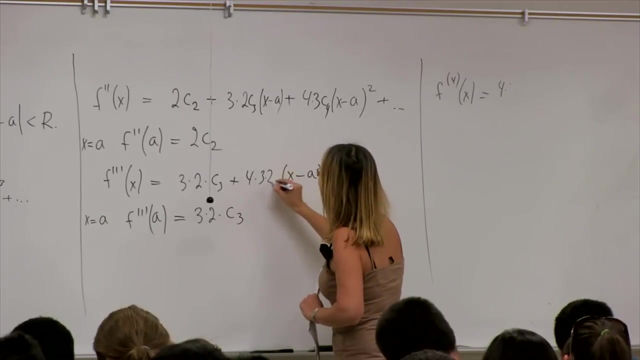 Let's do one more: F4.. Okay, So I have to take this expression and differentiate it. I only have one term. Okay, I have 4 times. oh, and I forgot the coefficient C4 here. sorry, This is terrible. 3 C4, like this, sorry. 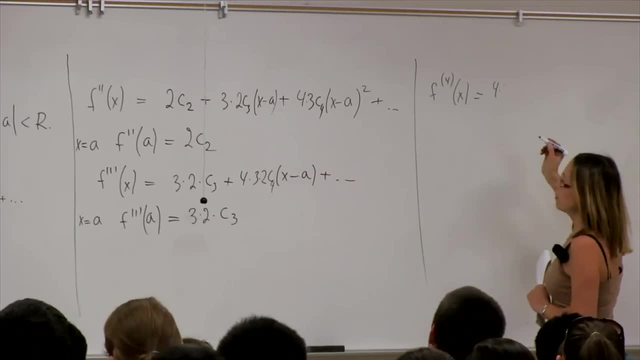 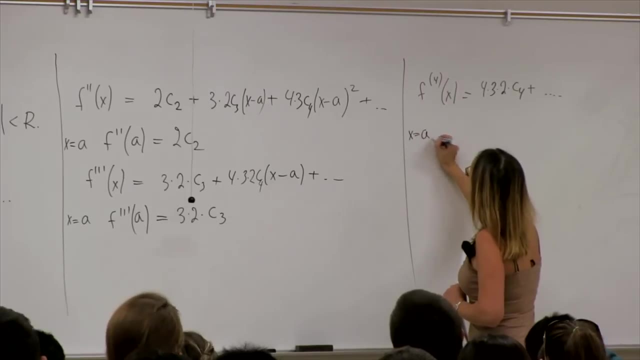 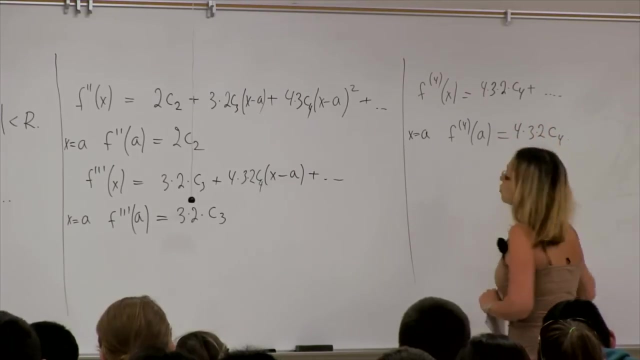 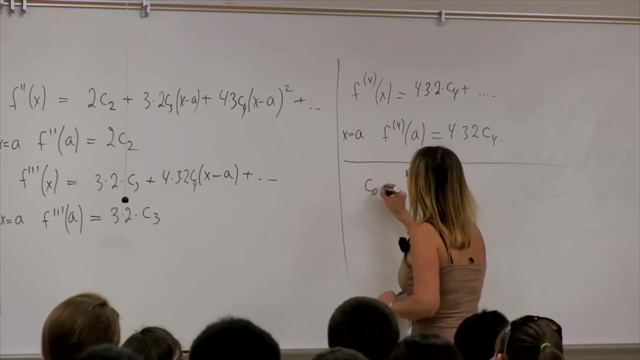 So I have 4 times 3 times 2 C4 plus something else. So, evaluating at A, I get the fourth derivative, that is equal to 4 times 3 times 2 C4.. Okay, let me summarize. So C0 is equal to f of A. That's from the 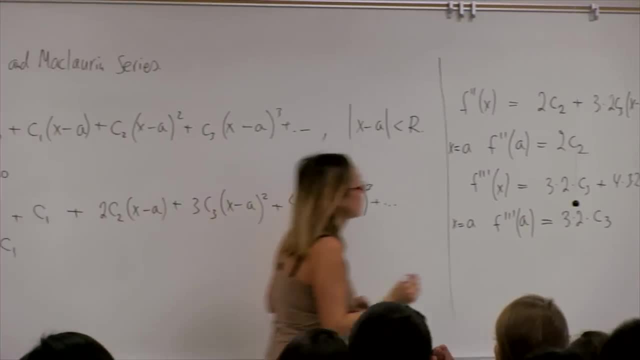 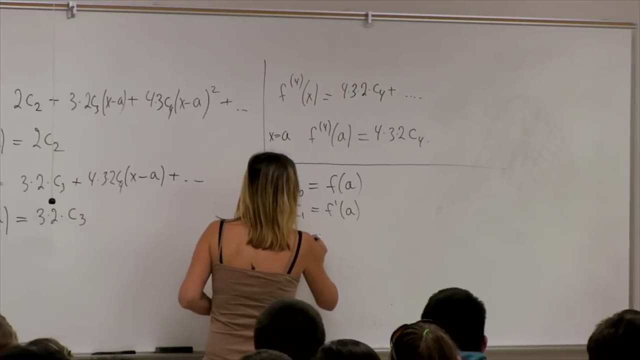 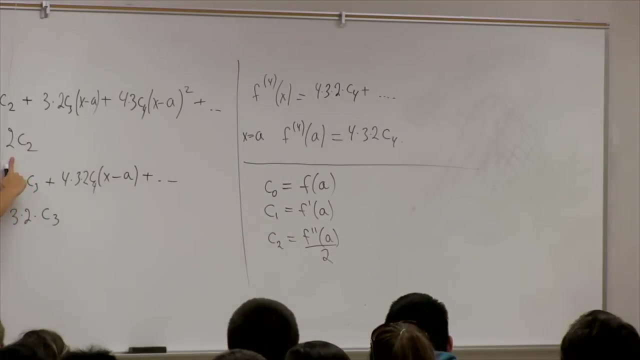 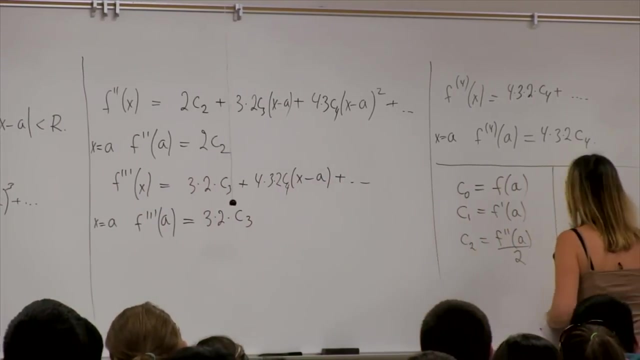 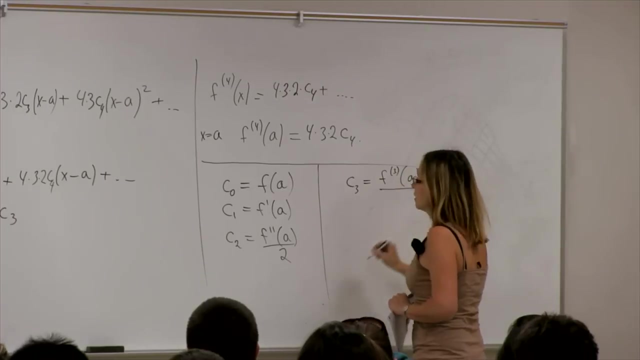 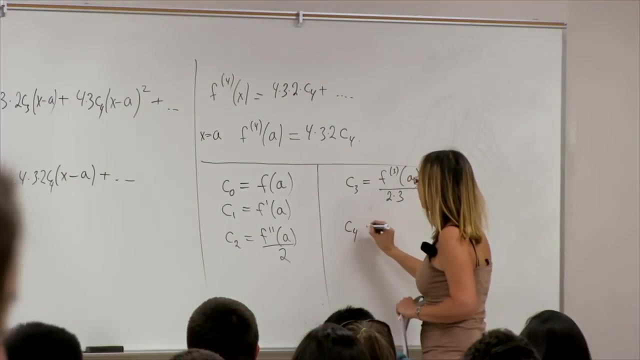 first experiment: c1 is f, prime of a. c2 is f, prime, prime of a, divided by 2. from this expression remember that number 2 that popped up: c3 is f, the third derivative at a, divided by 2 times 3.. c4 is the fourth derivative, that's from here. 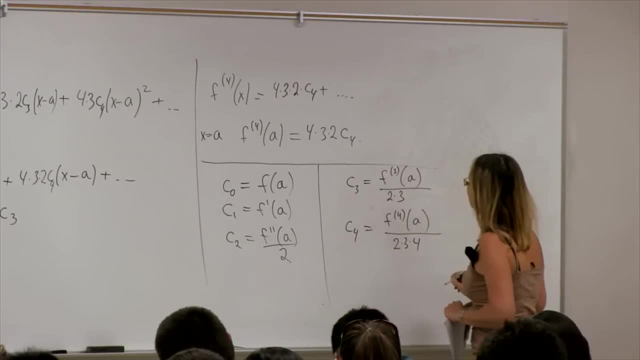 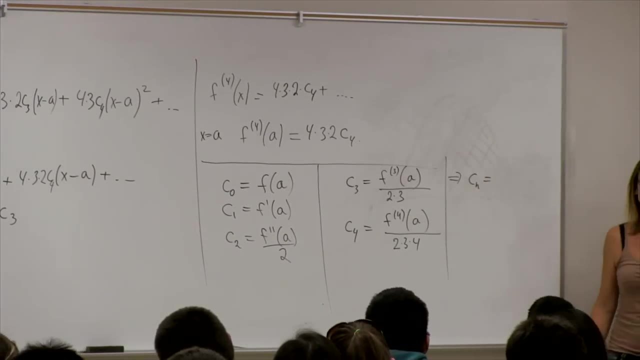 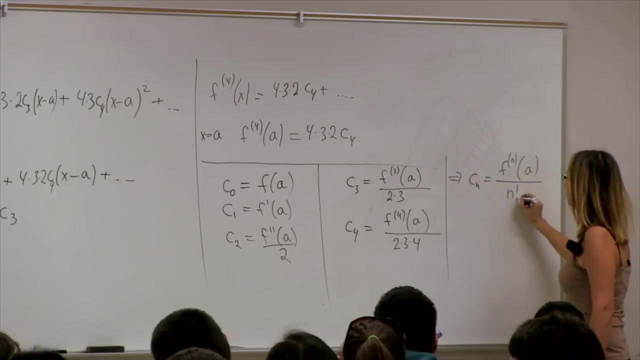 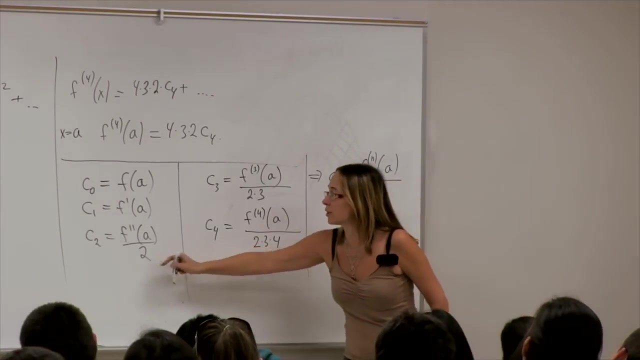 divided by 2 times 3 times 4.. I now ask you, what is cn guess the pattern? f? nth derivative evaluated at a n factorial, yes, okay. so one question. so I can see a 2 factorial here. right, how about this one? this is 1 factorial, that's okay, this one. so we have to make. 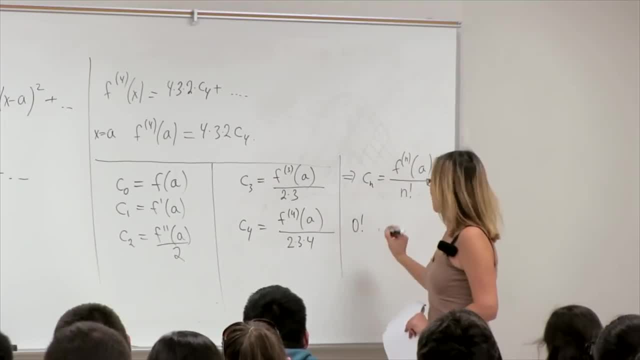 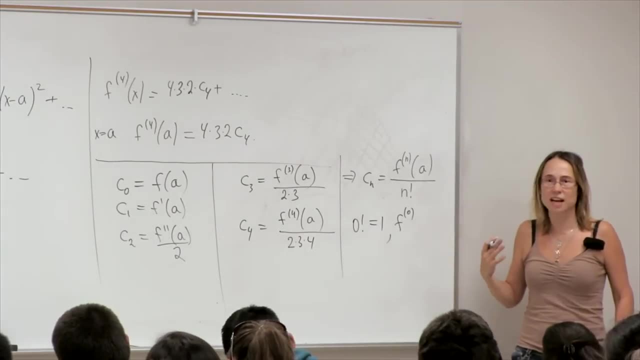 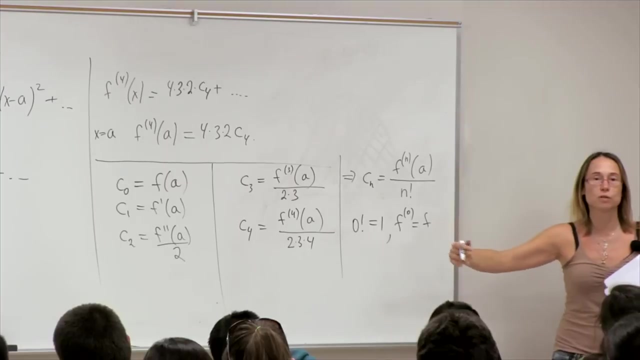 some notation. so what is 0? factorial is 1, and what is f? the 0s derivative, that's when you take a derivative 0 times. so that's just f. okay, so everything is great. we have a whole pattern that works for any index. okay, so this is a very nice. 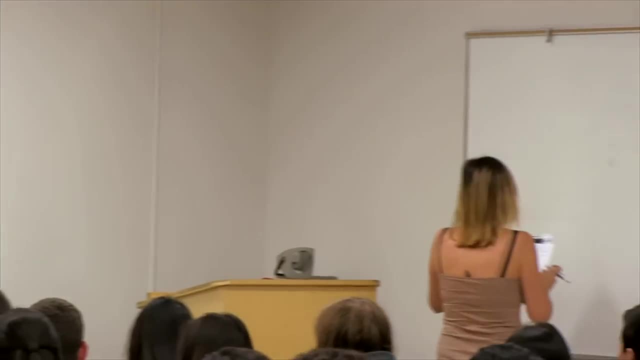 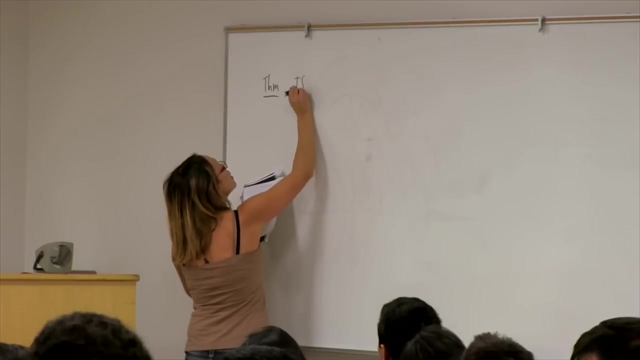 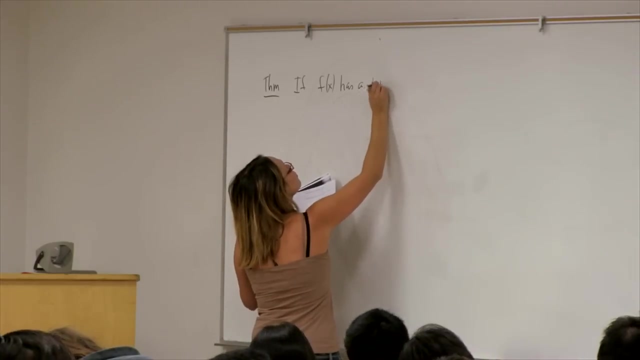 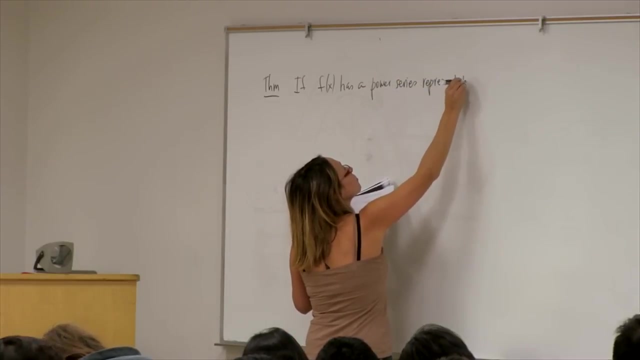 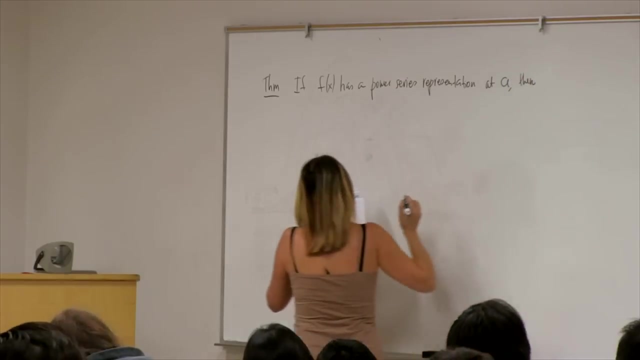 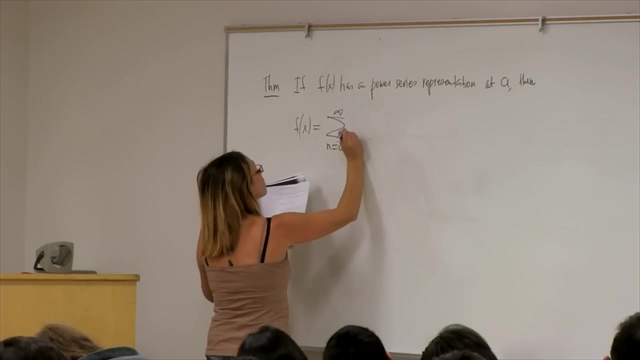 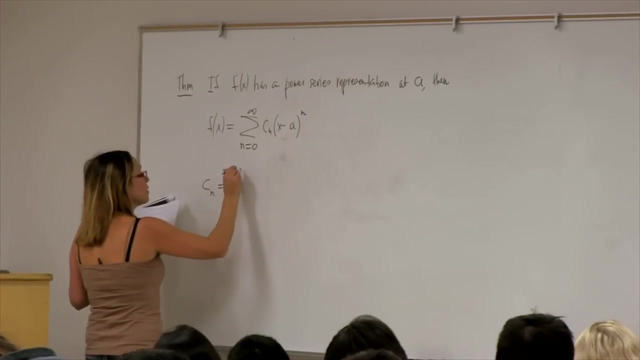 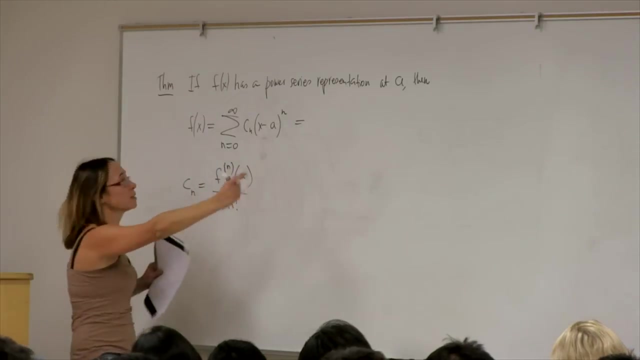 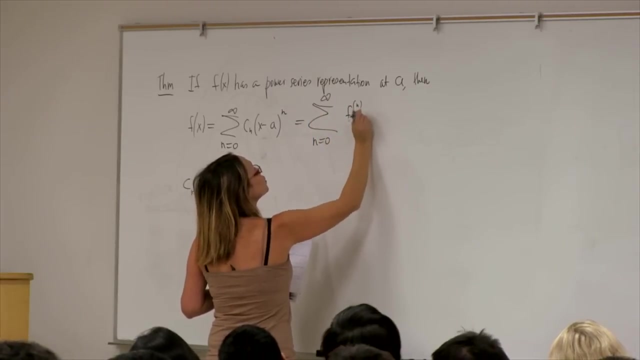 discovery which we can formulate in the following theorem: if f has a power series representation at a, then f of x is given. by this formula, we are c. M is f? nth derivative of f at a, divided by n? factorial, which allows me actually to write this formula in a more explicit fashion. I have f? n derivative of a over n. 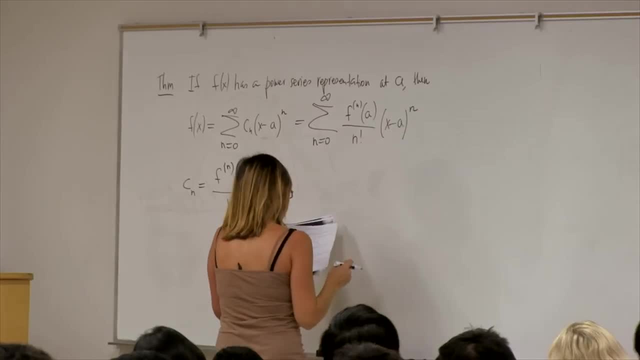 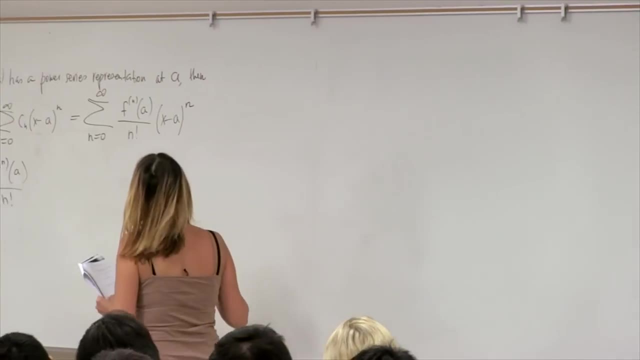 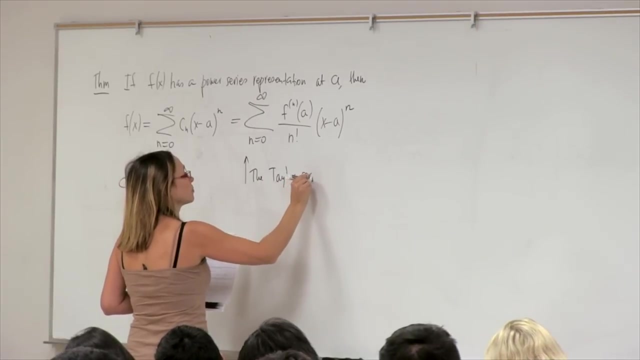 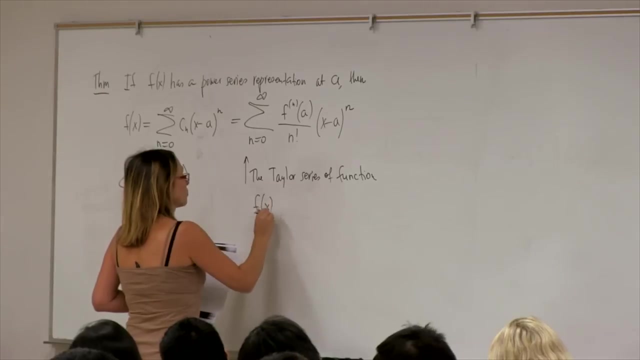 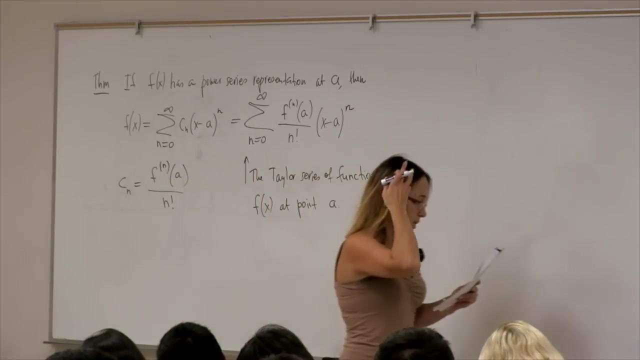 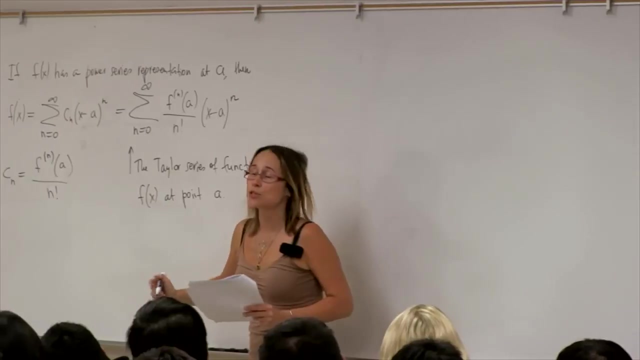 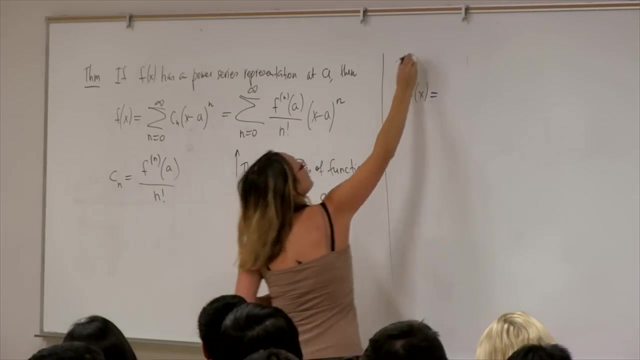 factorial: x minus n: factorial. okay, this is called the Taylor series of function. f at point a, at point a- and there is a special name for this series- when we expand at a equals zero. so you can write down: f of X, set a equals zero. okay, this works for. 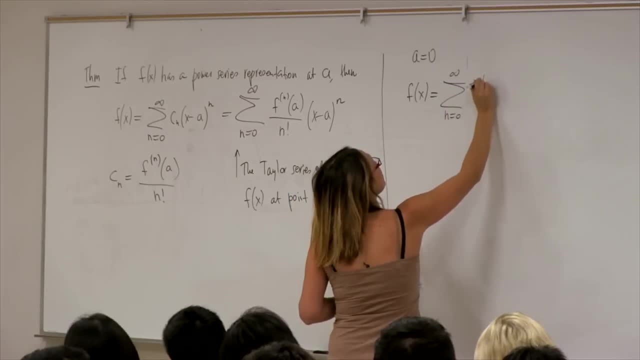 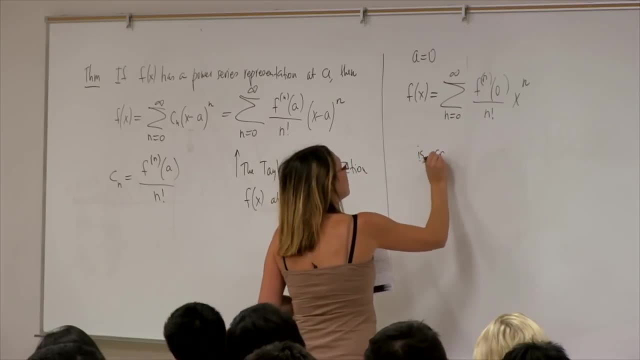 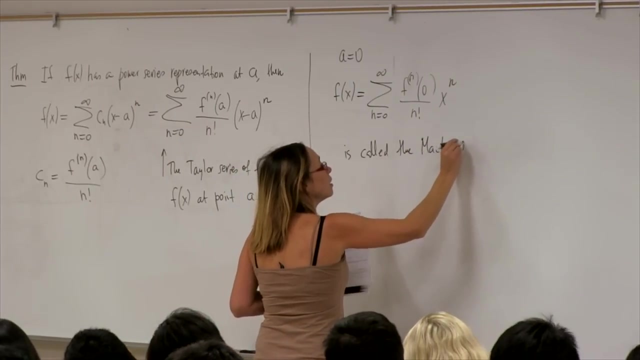 any a. so you can write down f of X, set a equals zero. okay, this works for any a. so I can write down f of X, set a equals zero. okay, this works for any a. so I let me write the special form at zero is called the Maclaurin series of function. 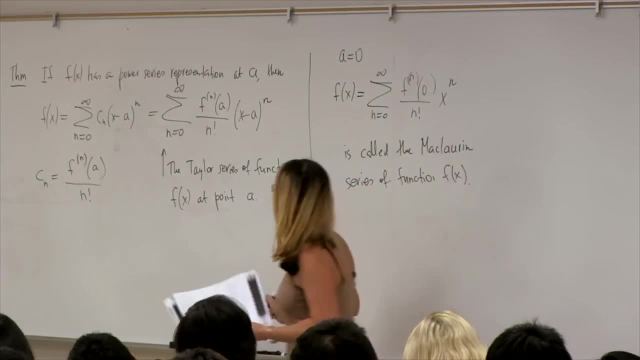 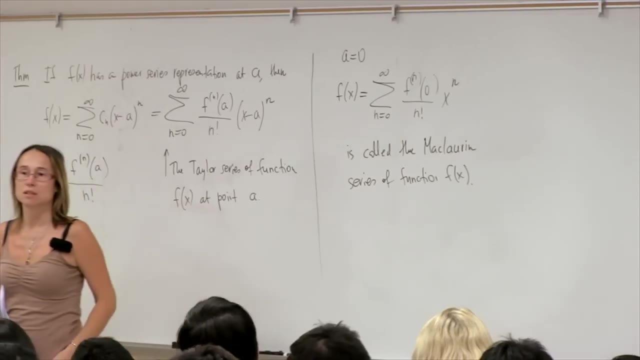 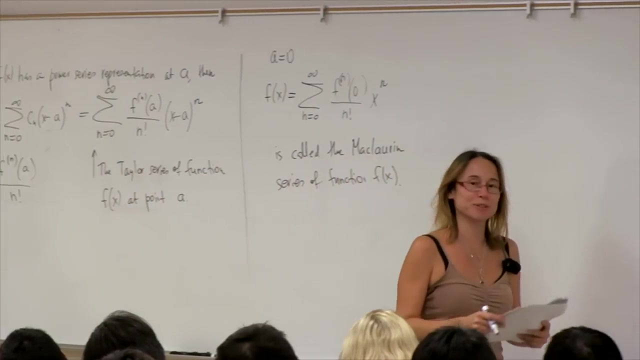 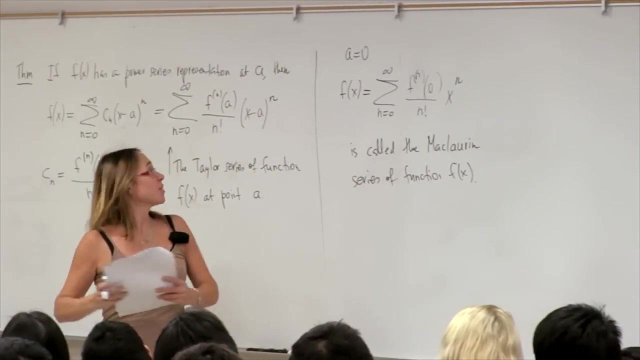 f. so when you write down the Taylor series at zero, this is called the Maclaurin series of function. but nobody uses that, at least well, not in my area of math. okay, so there are a lot of if statements here. this expression or this only makes sense if 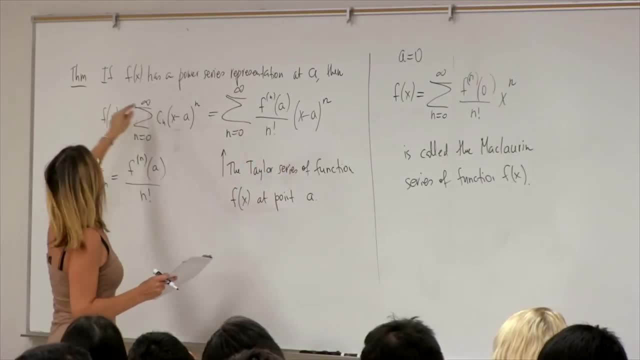 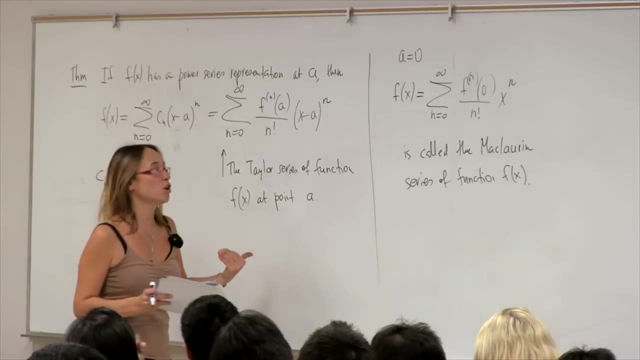 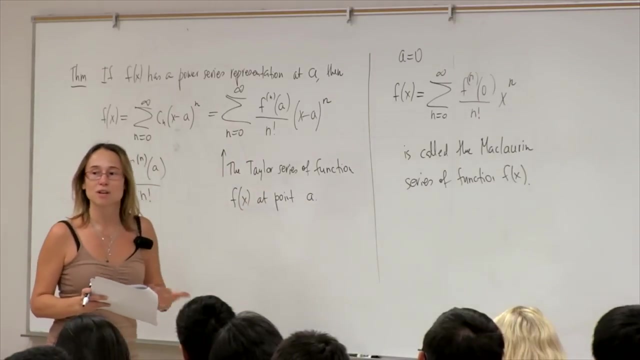 it could be very just right and we said that if f of X has a representation as a, as a power series, then this is true. so we don't actually know whether this converges and we don't know, if it converges, whether it converges to the function F. this are, these are still things that we 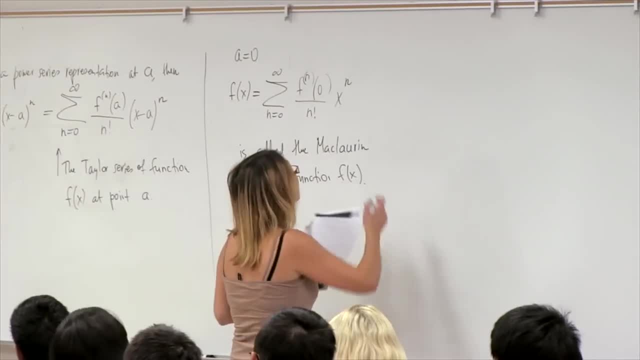 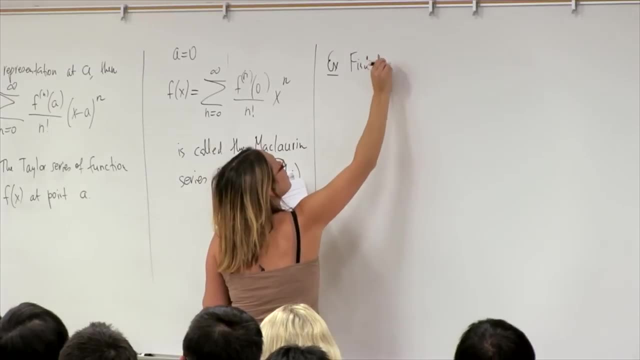 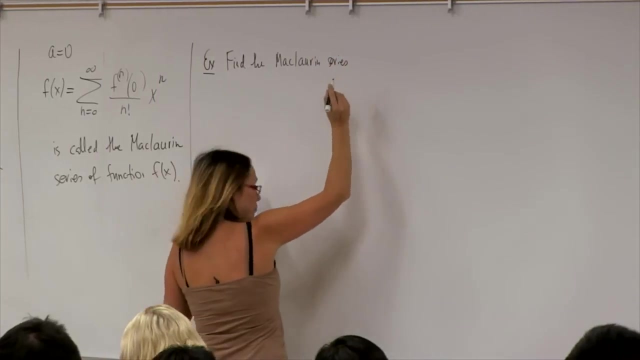 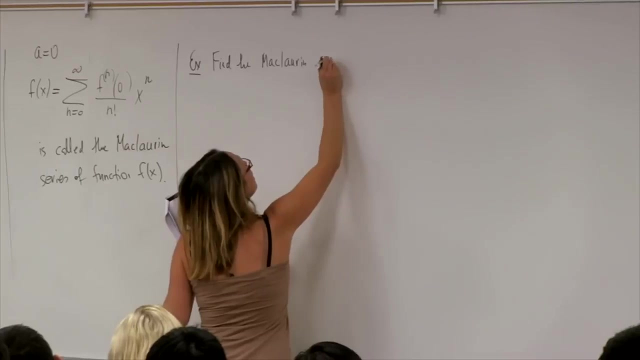 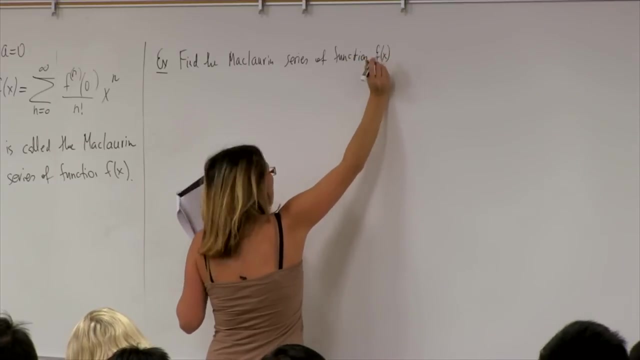 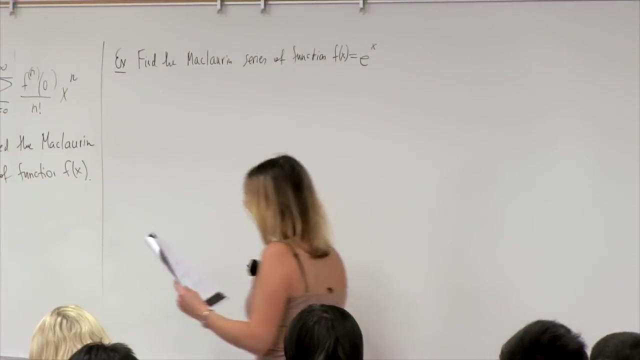 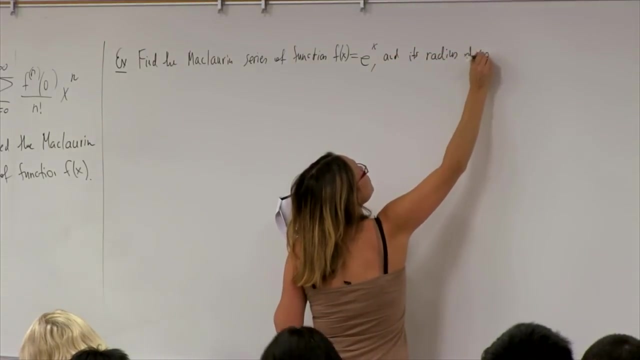 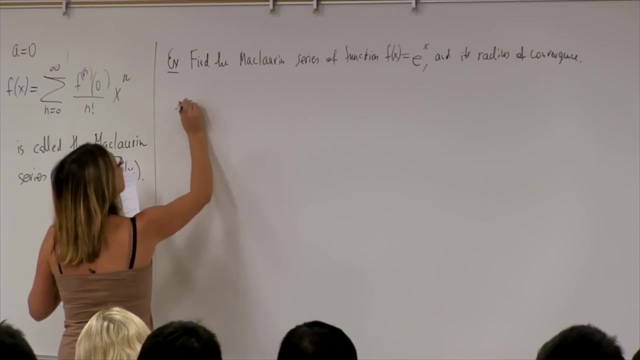 have to address. ok, so are, but will work with some examples. find the Maclaurin serious of function f of x. f of x equals e to the x. this is the easiest serious expansion and its radius of convergence. so if f of x. in order to write down, 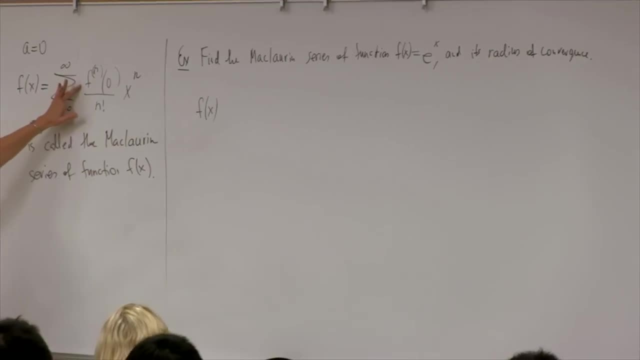 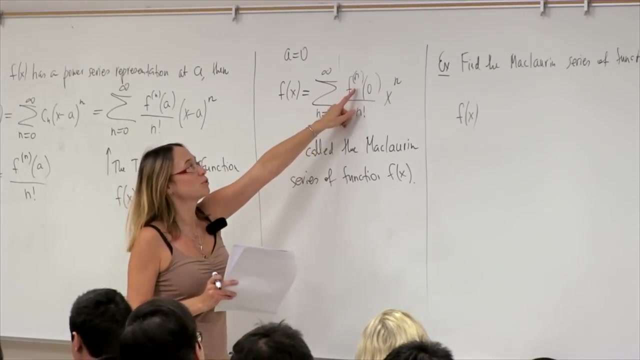 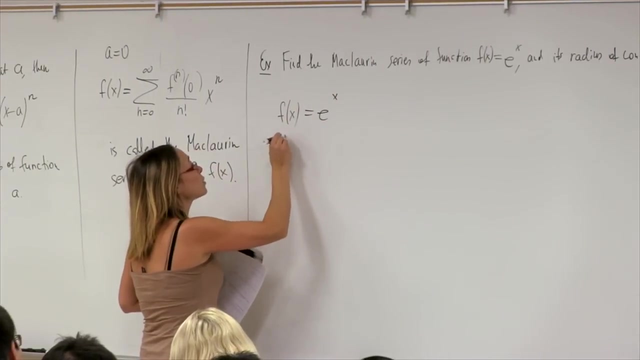 the Maclaurin series, I have to evaluate the derivatives of f at 0, the infinite number of them, the first derivative, the second derivative, and so on. let's do it for the exponent. so if f of x is equal to e to the x, then what's f? prime of x? 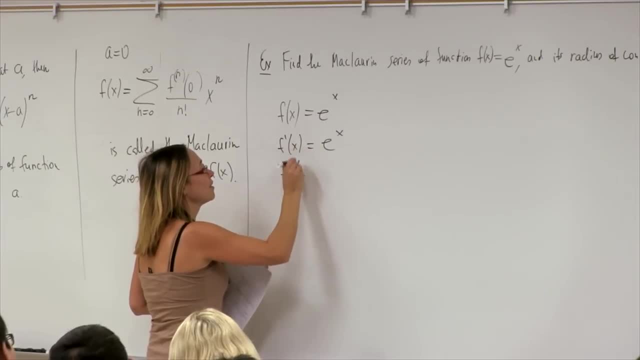 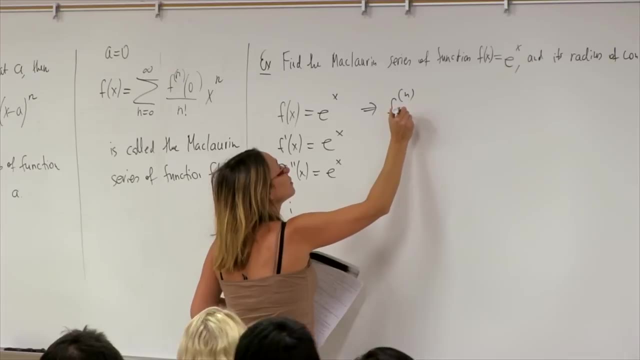 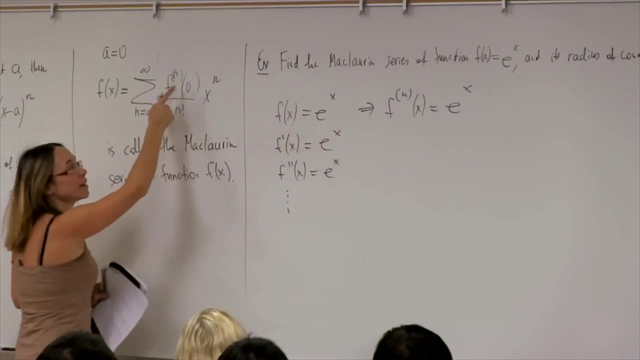 uh-huh, how about f, prime, prime and so on? right, so we can say that f? n of x is e to the x. what we really need is f? n of 0. f n of 0 is e to the 0, which is 1. 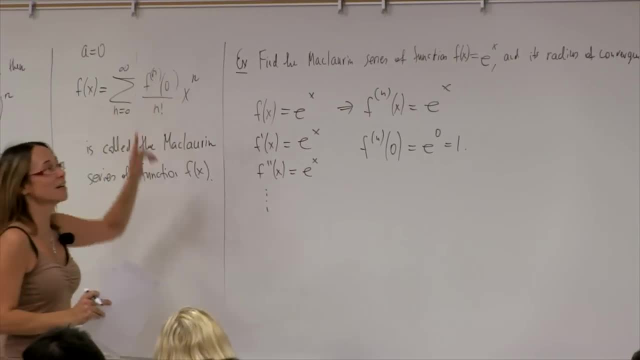 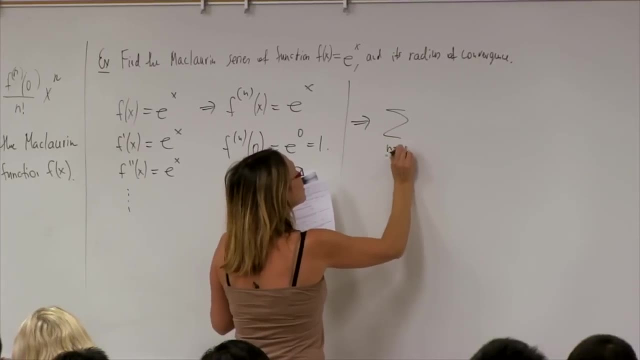 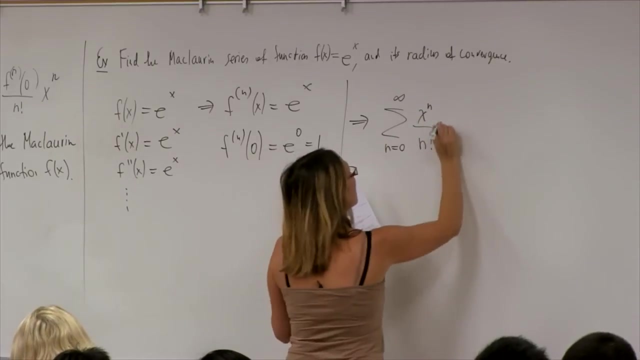 so all of these are 1, that's why it's the easiest. so we can say that: um, we have the sum from 0 to infinity, x to the n? n factorial, and I'll write it down, skipping the sigma notation, just to show you what it looks like. 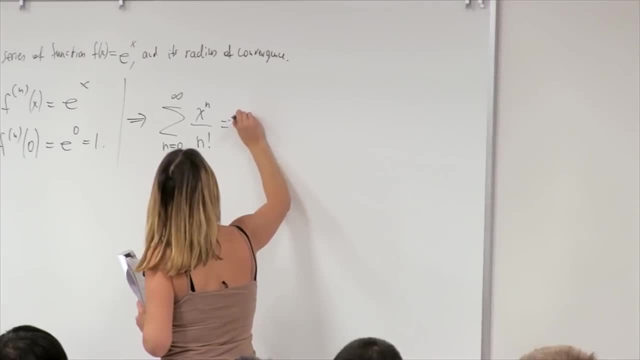 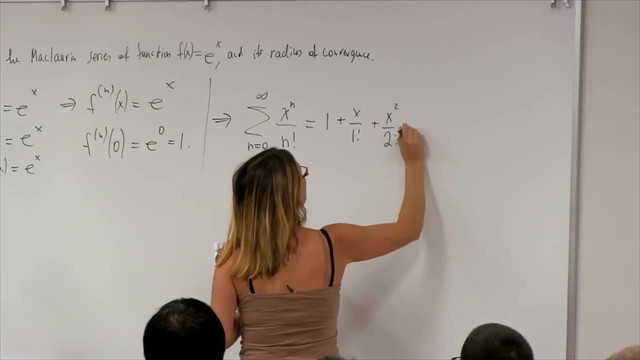 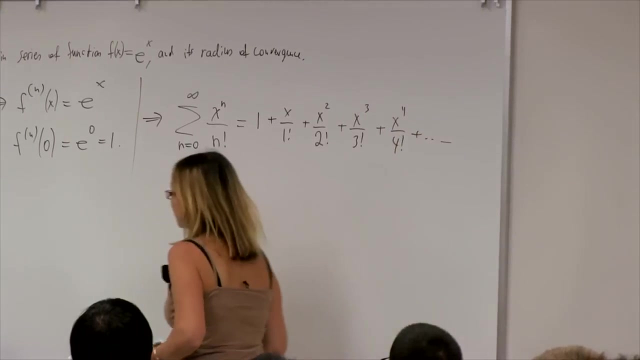 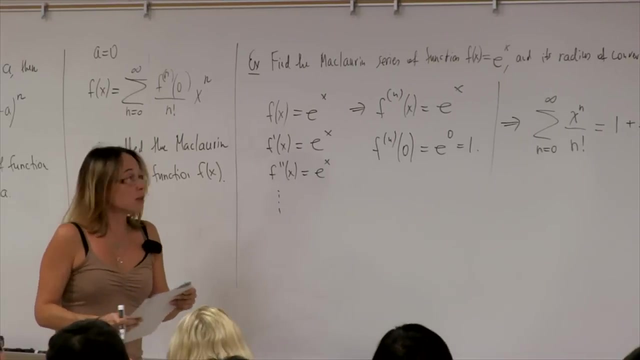 so when n equals 0, we just have 1, and then we have x over 1 factorial plus x squared over 2 factorial, plus x cubed over 3 factorial plus x, 4 to the 4 factorial, and so on. ok, um, fine, find the radius of convergence. 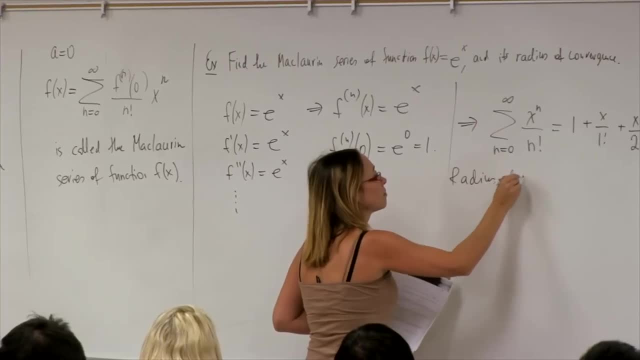 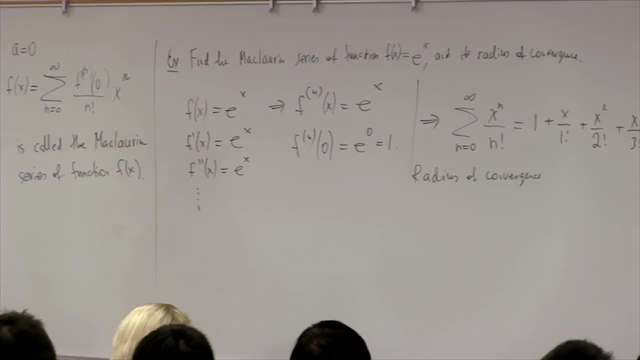 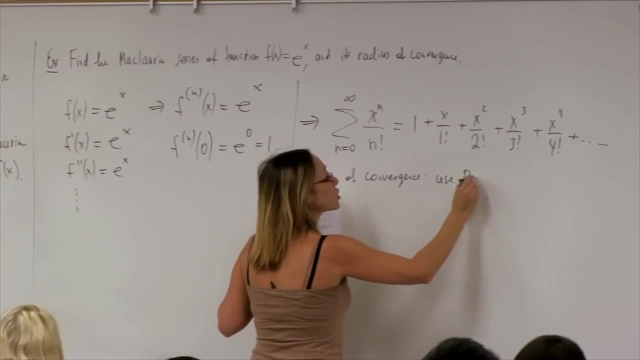 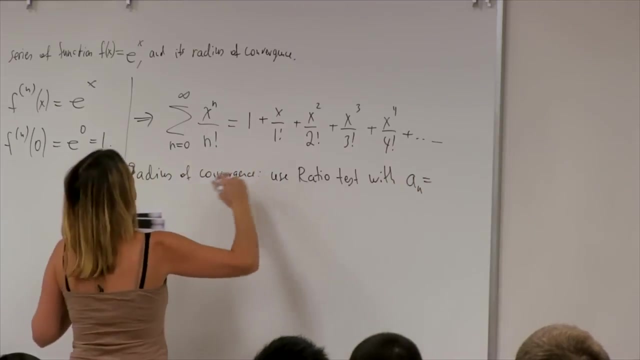 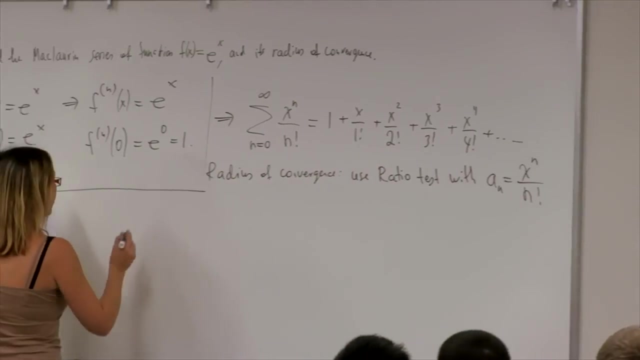 we always use the same method to find the radius of convergence. we'll look at the ratio test. ok, so um, with a n, use ratio test with a n. what's my general term? a n? it's equal to x, to the n over n factorial. so we have 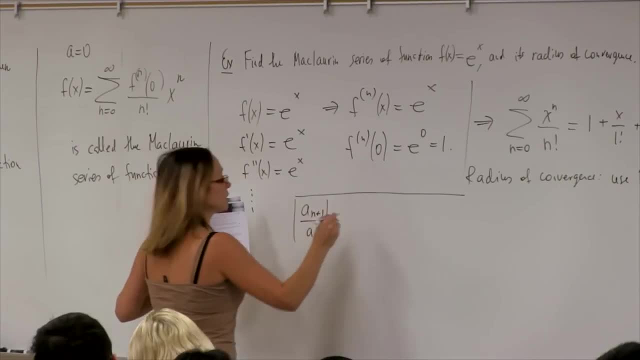 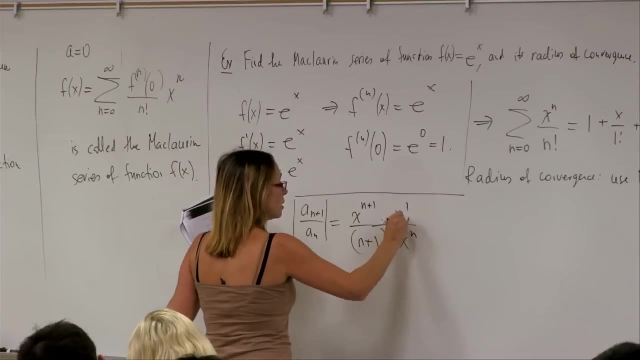 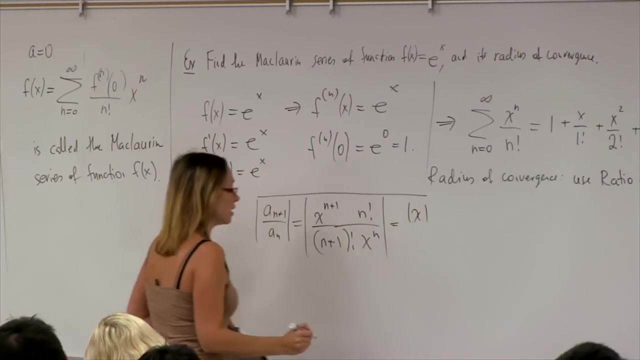 a n plus 1 over a n is x to the n plus 1. n plus 1 factorial divided by x to the n factorial, n, n factorial, like this, so x to the n cancels. I have 1 x here and I have n plus 1. 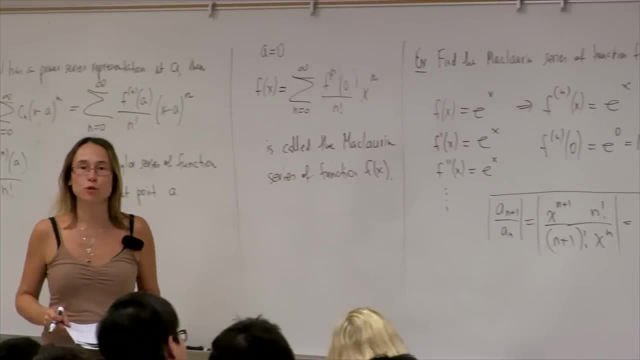 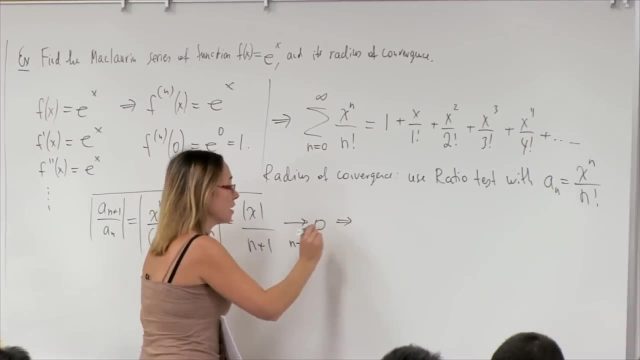 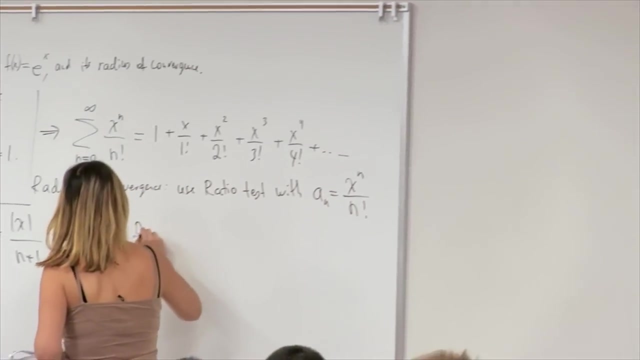 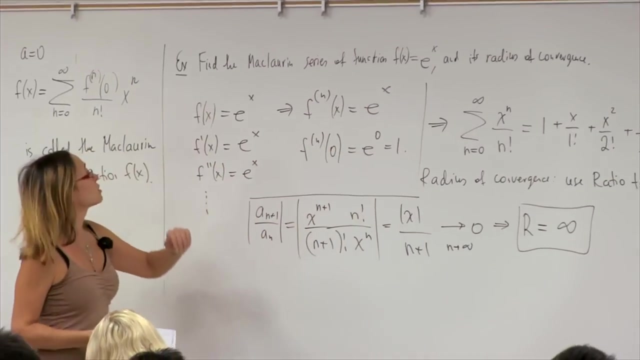 what happens to this when n goes to infinity? for any fixed x goes to 0 as n goes to infinity. therefore the series converges. for any x right, the radius of convergence is infinity. the exponent is very nice. this way it's convergence for any x question. 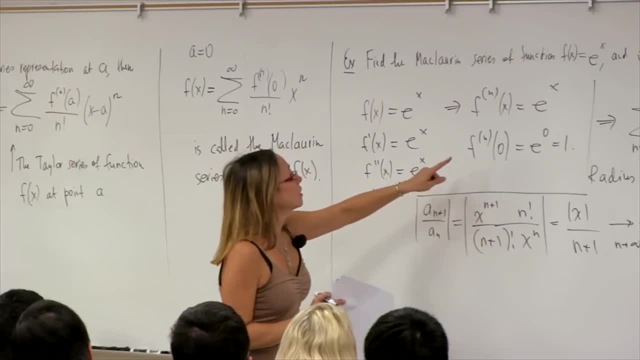 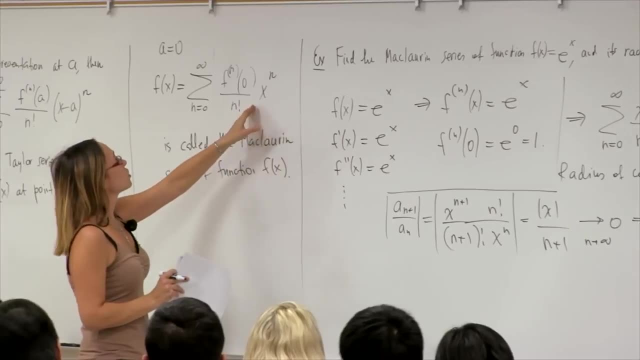 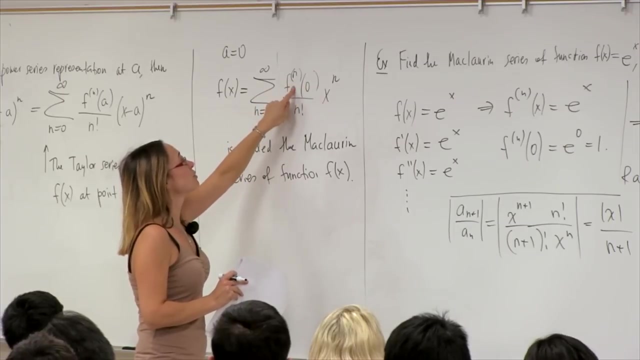 how did you get x to the n over n factorial, from e to the x? this one, yeah, how did you get that? so this is the general formula. ok, so x to the n is there, n factorial is there. the missing component is my function evaluated at 0. 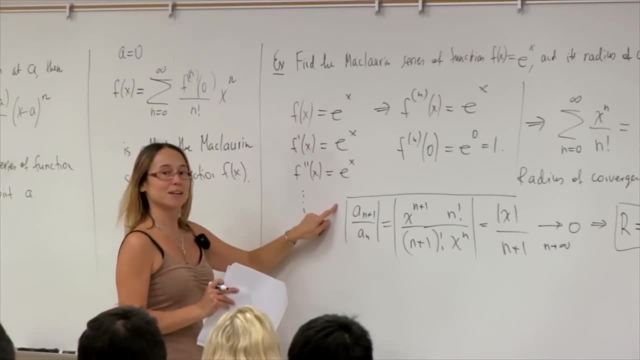 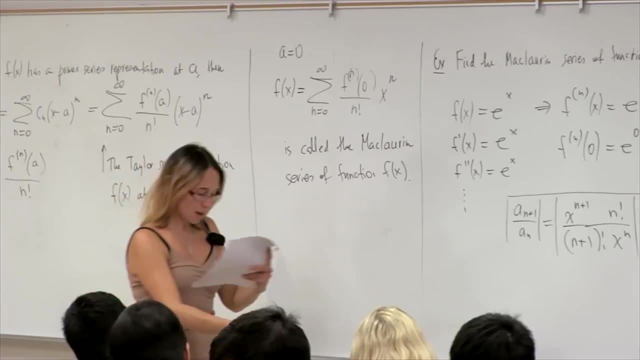 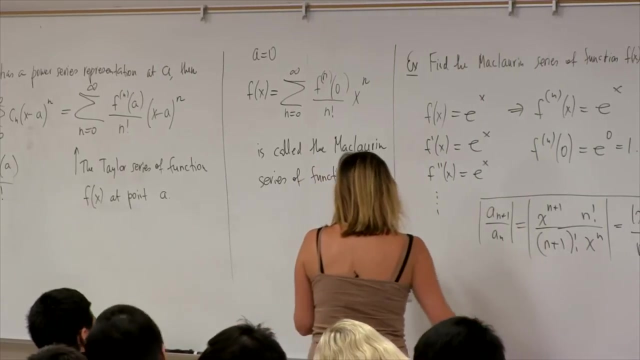 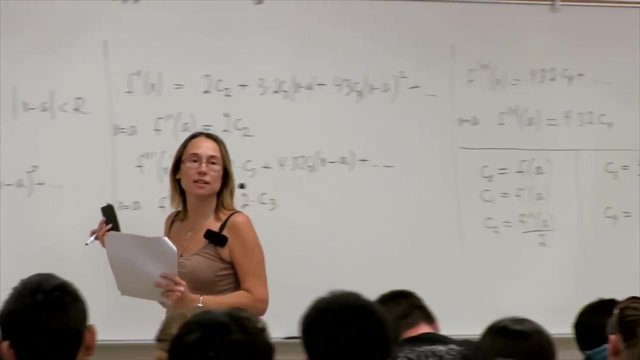 my function is the exponent. all the derivatives are exponents. evaluated at 0, they all become 1s. ok, more questions. ok, so how do we know whether a power series converges to, whether the Taylor series converges to the target function f we can take. 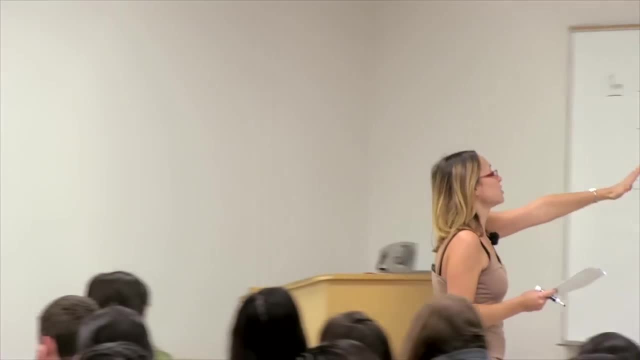 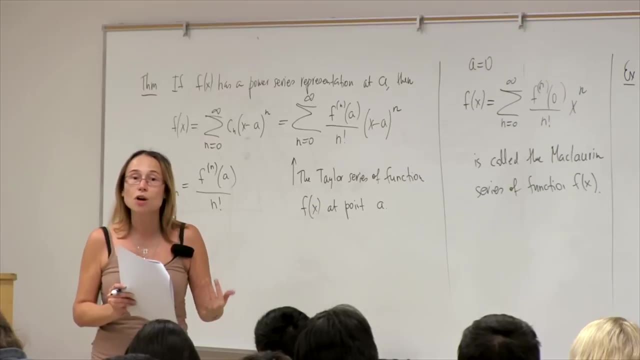 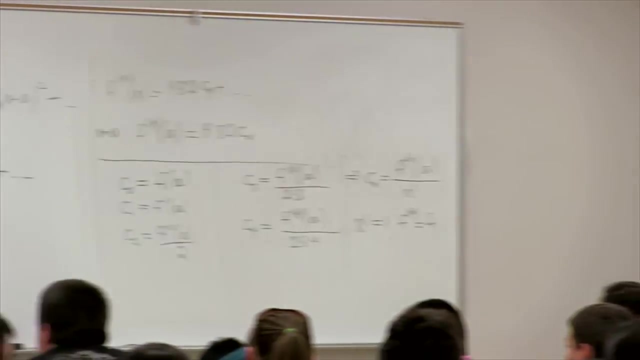 a given function f, write down this representation and even evaluate its convergence, we'll say, ok, it converges, but where does it converge to? we should still evaluate the limit, ok, and most importantly, we should figure out whether it indeed converges to the function f right. so 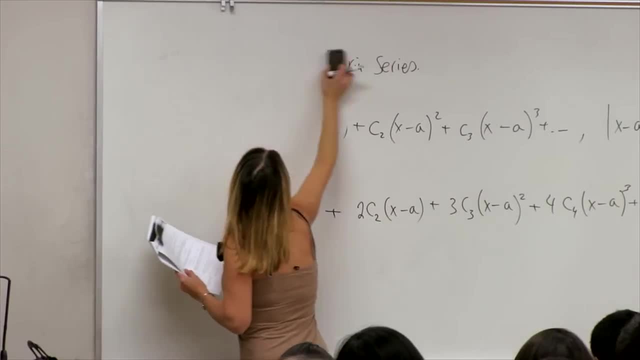 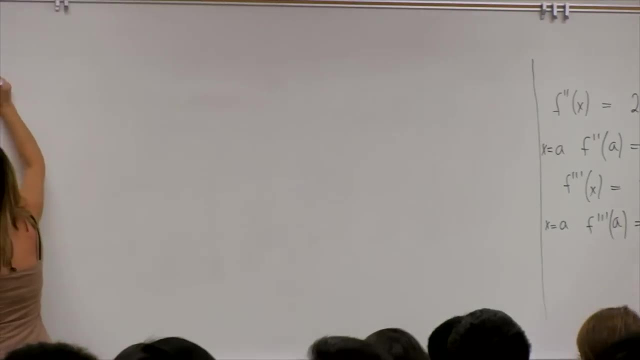 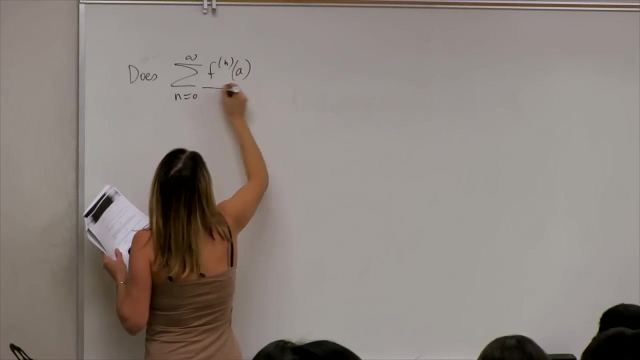 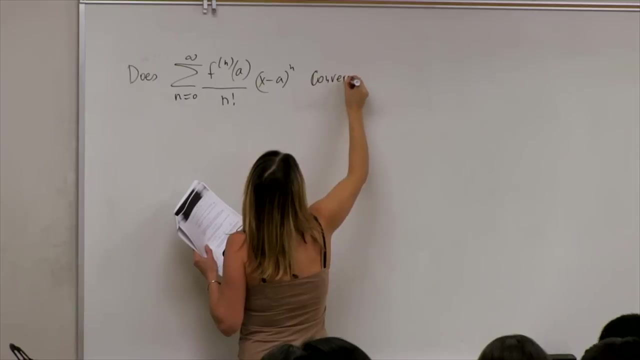 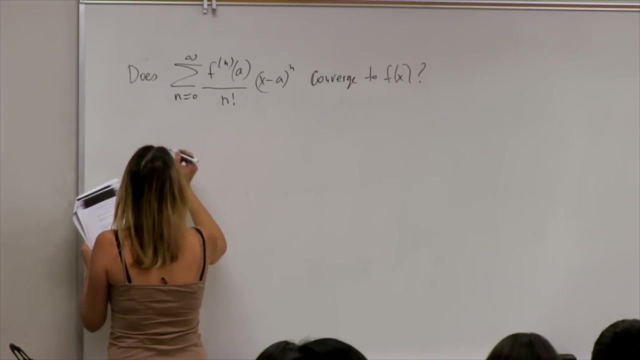 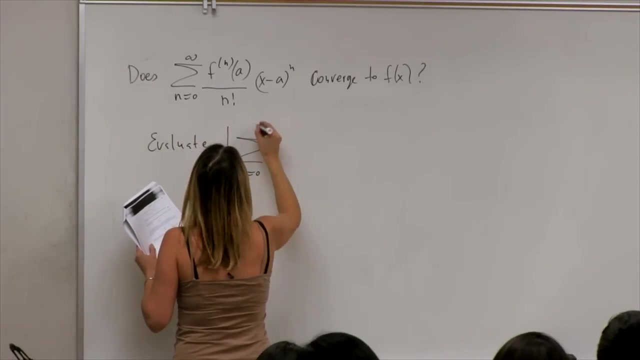 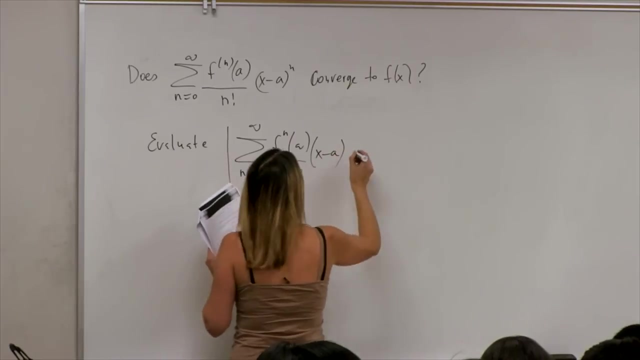 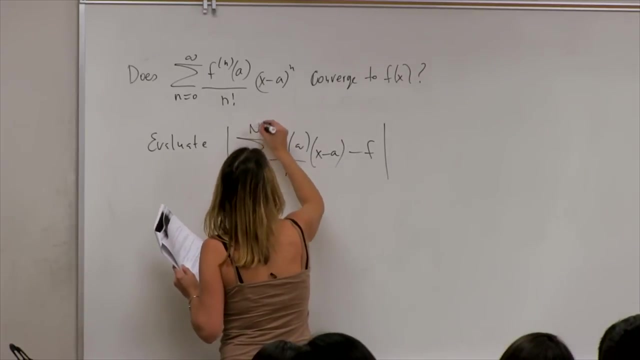 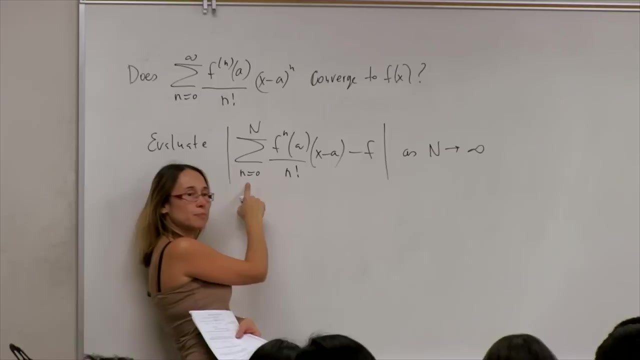 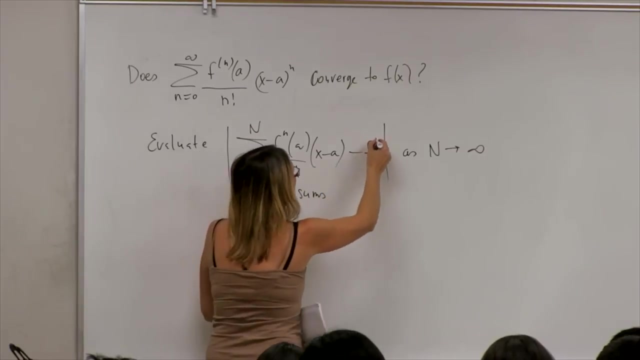 the general method of doing it is to compare the series with the target function f. so does this converge to f, right? so we have to evaluate the difference. as n goes to infinity, we want to look at partial sums, partial sums, and we want to figure out what. 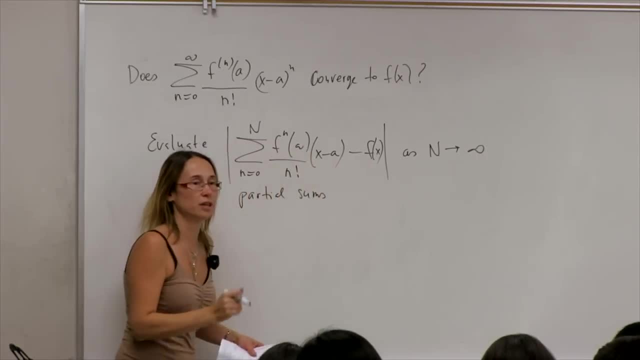 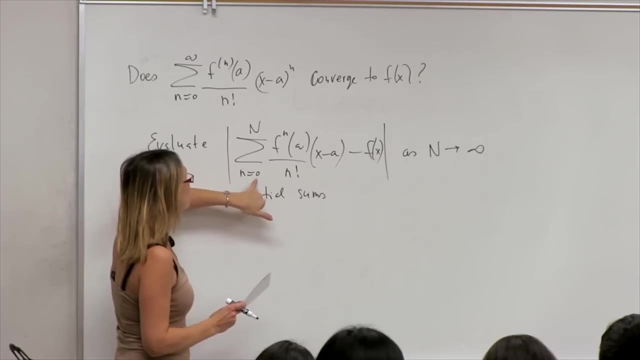 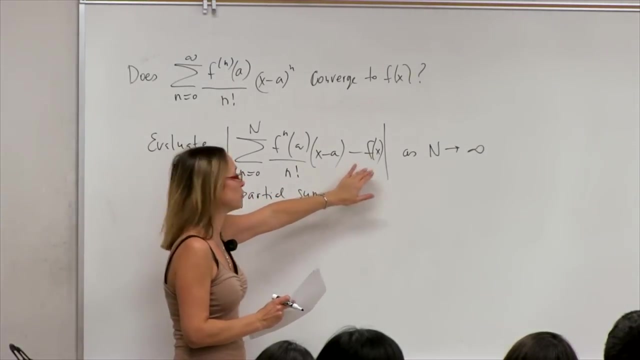 how close we get to the target function f, as n goes to infinity. n is where I cut my infinite summation. so I'm going to sum from n, from 0 to capital n and take the difference between the partial sum and the target function, and I want to make sure that. 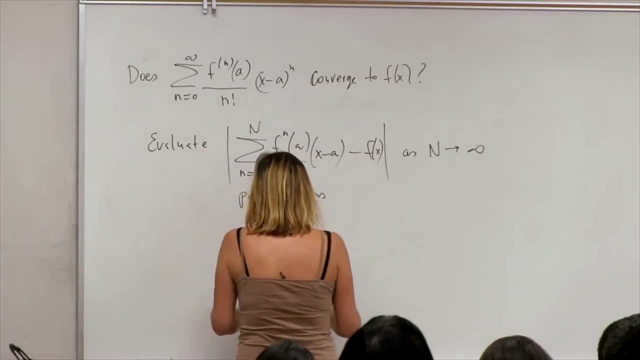 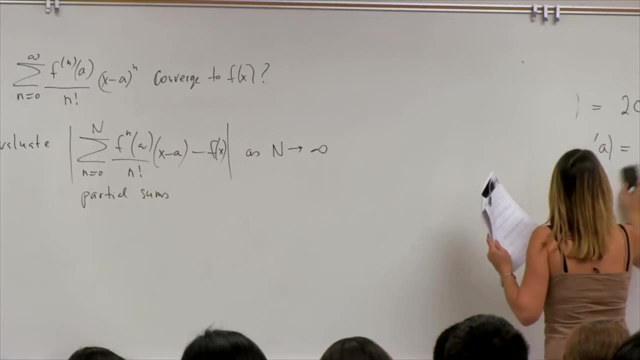 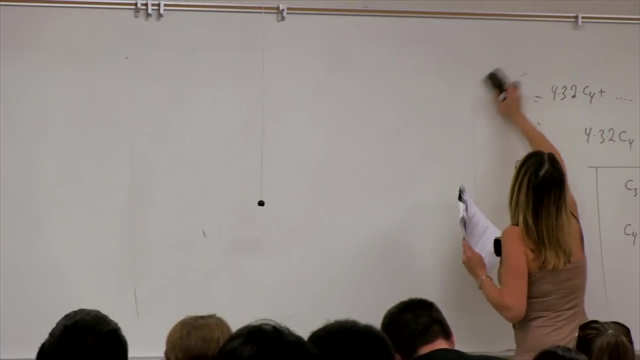 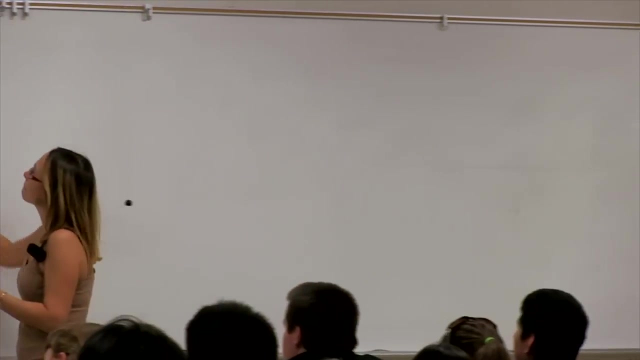 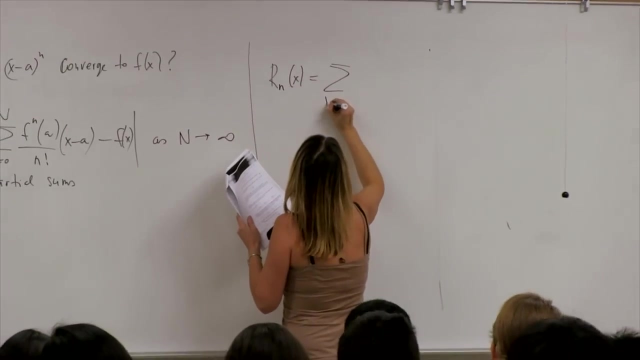 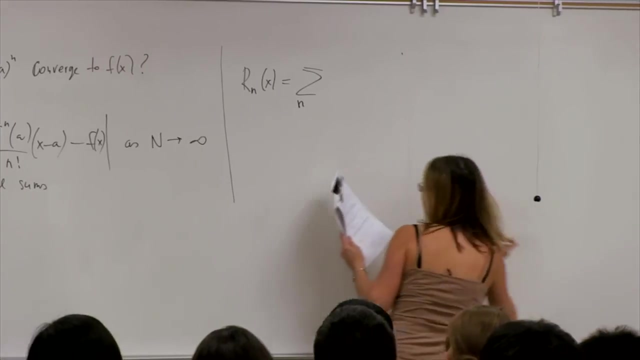 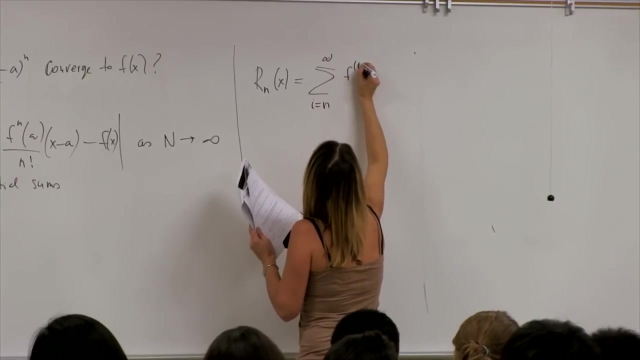 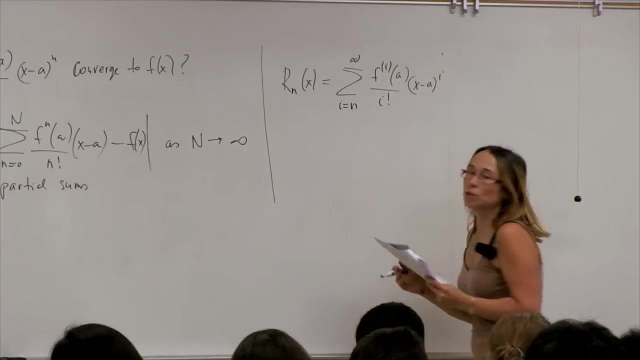 as n goes to infinity. this goes to 0. ok. this is called the remainder. ok, um. ok. rn of x is defined as n? um ok. rn of x is defined as n? um. ok. rn of x is defined as n? um ok. these are all the terms that remain. 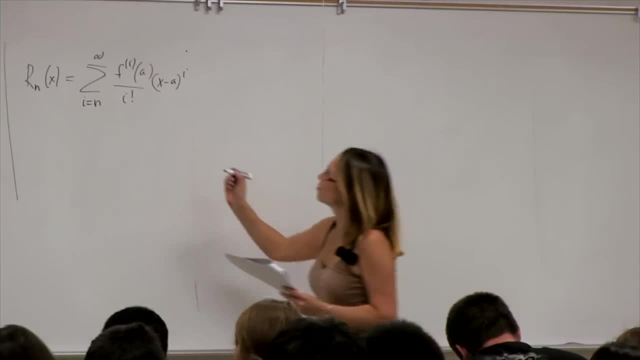 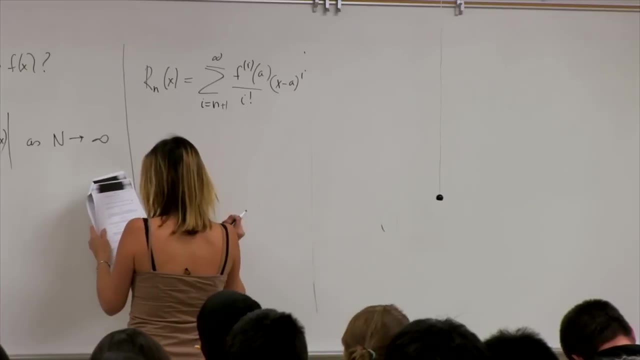 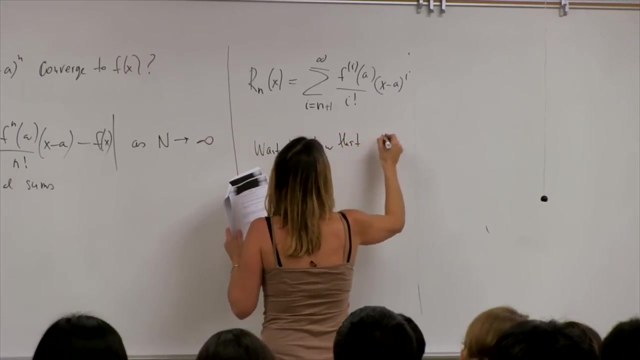 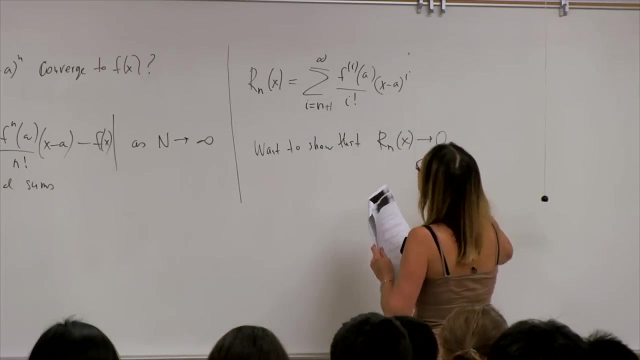 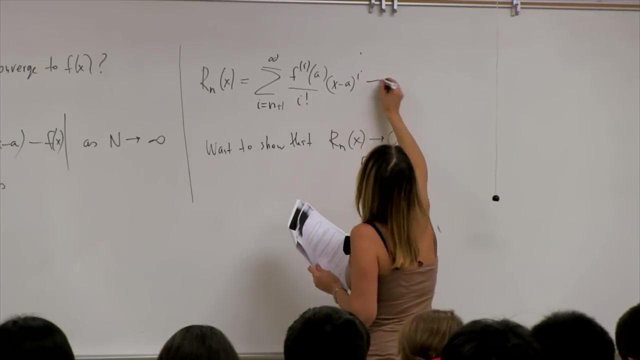 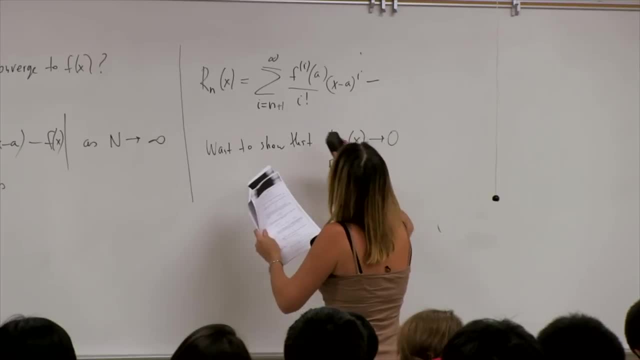 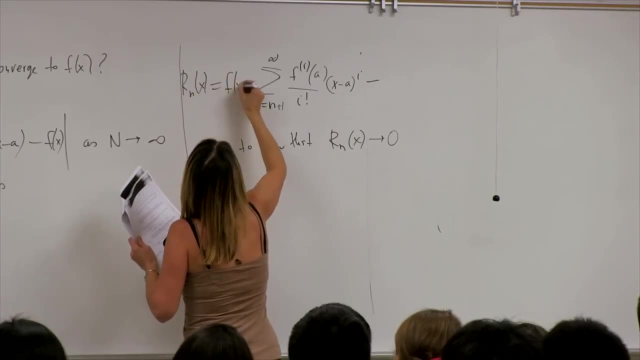 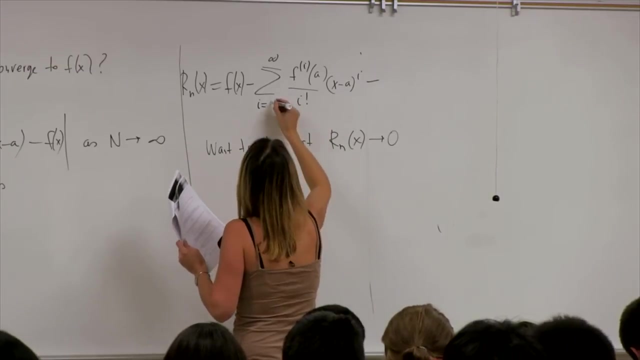 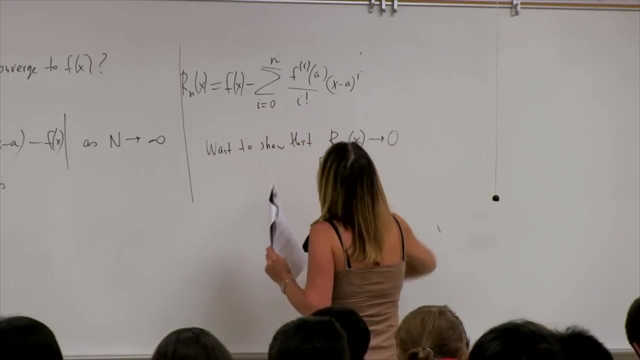 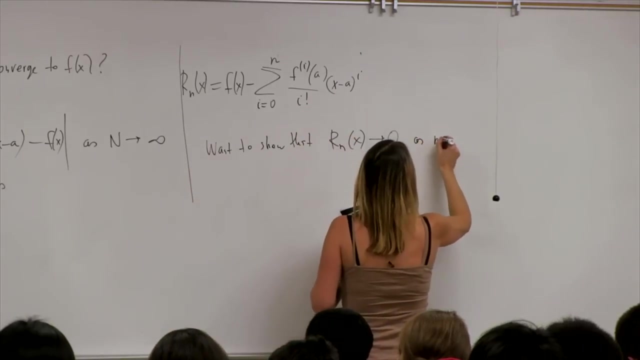 I'm sorry, I'm confused. I'm confused the notation. so this is the definition. so it's the difference between the target function and the first n terms. in my summation I want to show that this goes to zero, as n goes to infinity And there is a theorem. 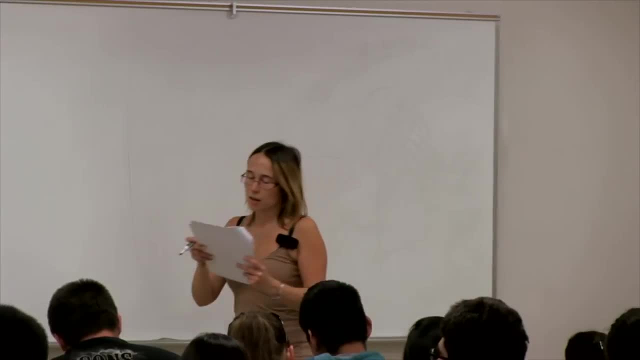 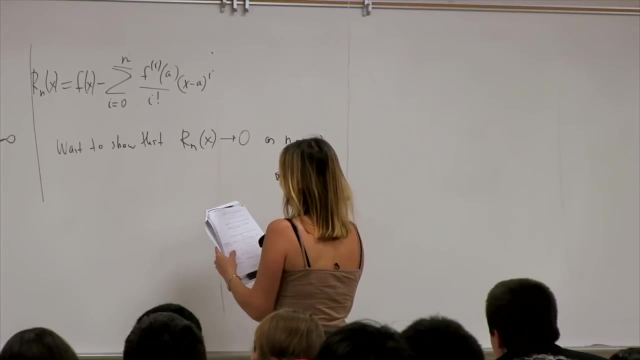 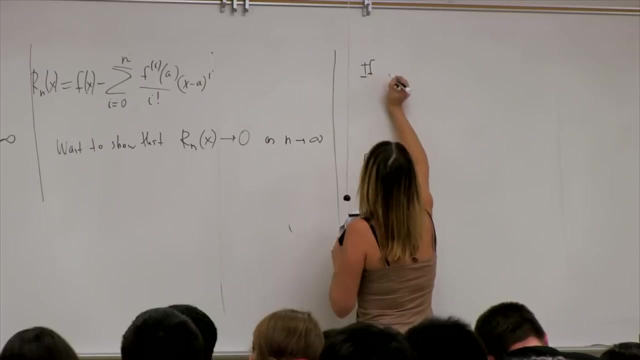 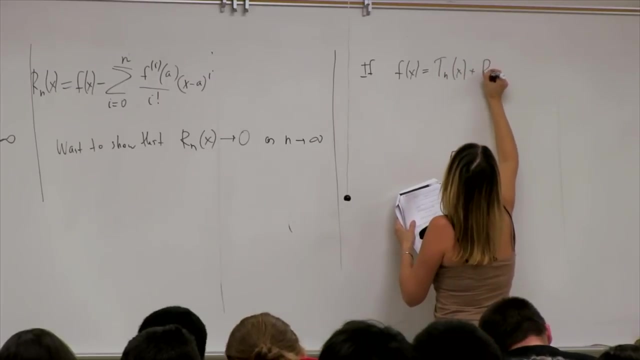 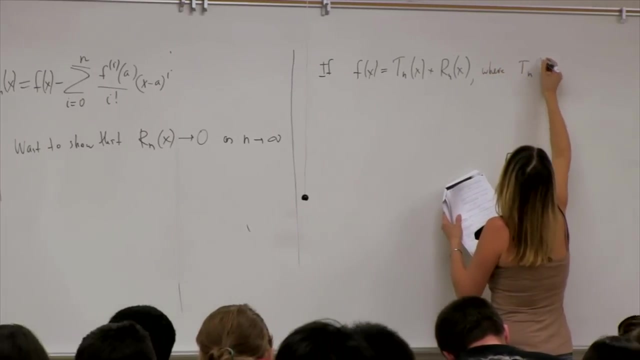 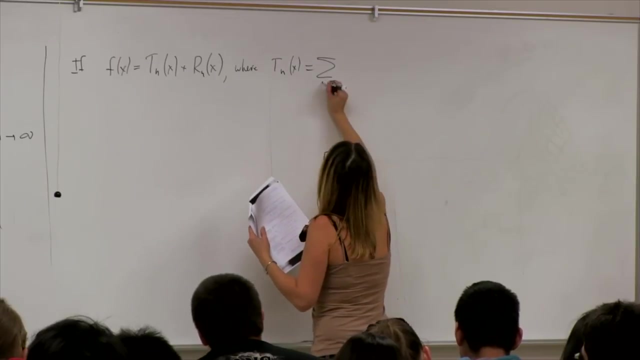 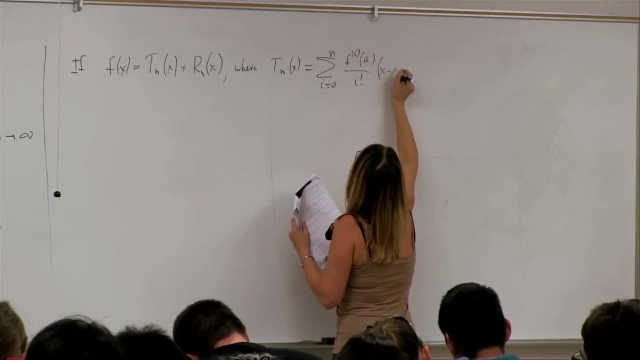 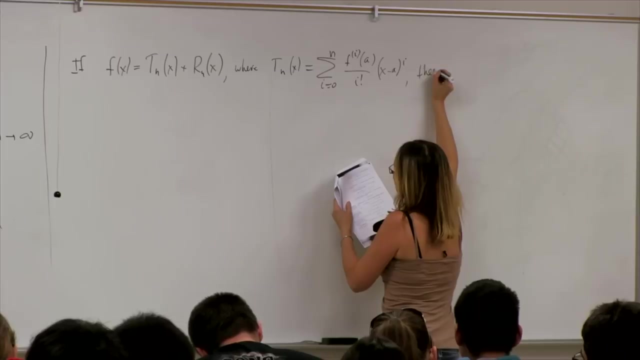 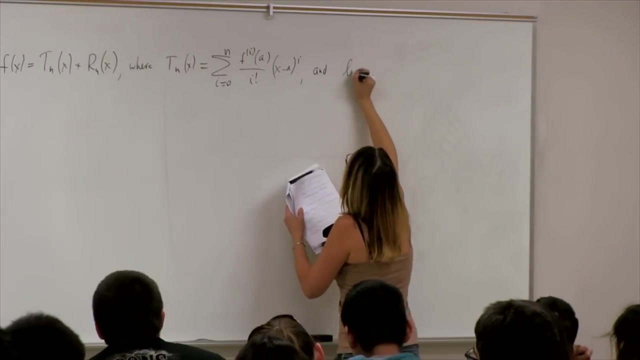 that appears without proof that allows us to calculate, to reason about this quantity. so if f is given by T of x plus r n of x, where T, n is all the terms from zero to n, and I just defined r n and the limit as n goes to infinity of r n, 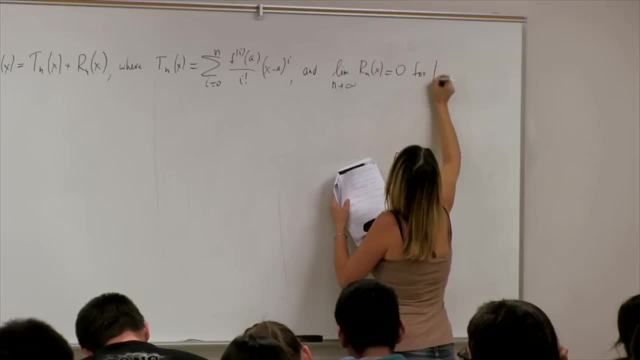 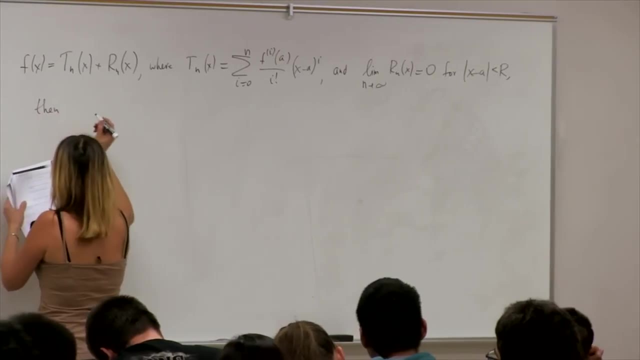 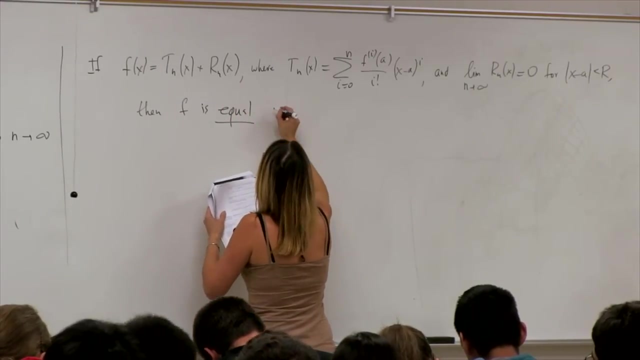 of x is zero for x minus a inside the radius of convergence, then we can say that f is equal to its Taylor series. So this is the equation for r: n of x is zero for x minus a inside the radius of convergence, Then we can say that f is equal to its Taylor series. 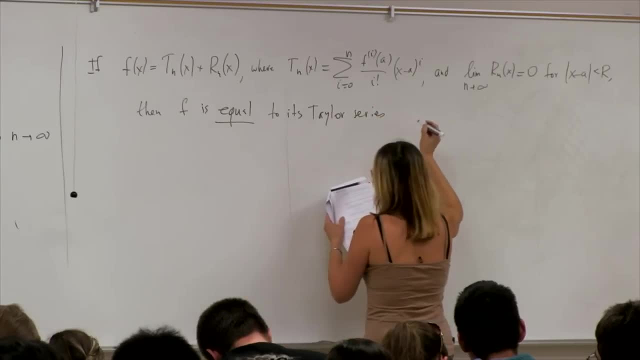 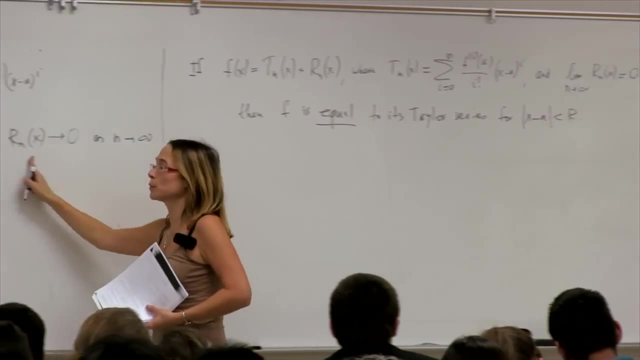 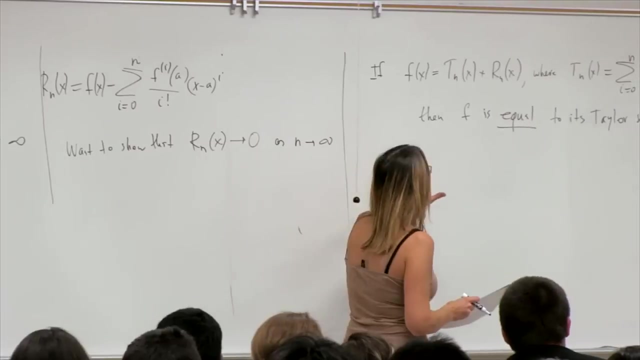 This is the flavouring matrix as x stop, x for x inside the radius of convergence. so basically, if we can show, if we can show that the remainder goes to zero, then f is equal to its- uh, steady representation. So what? we have to somehow get the handle. 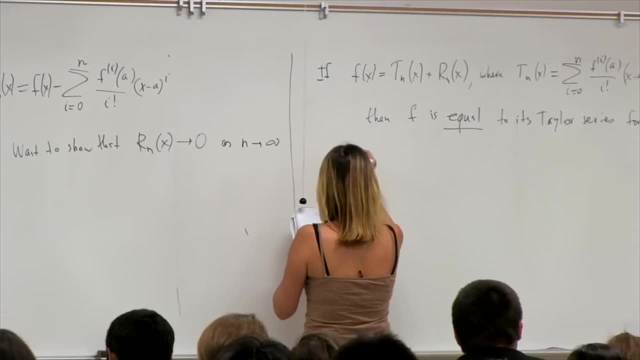 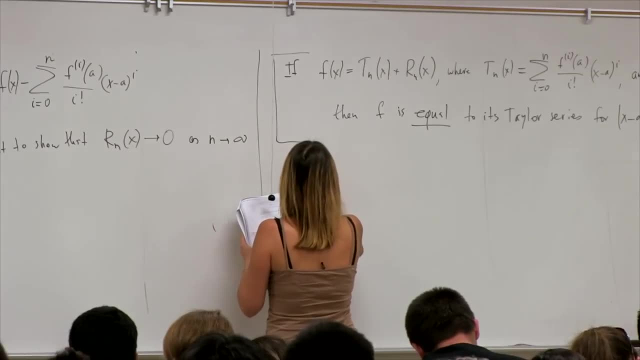 on this remainder Um. so here's a, a theorem um that helps us do this. It's called Taylor-. allright, we'll call this a V f of k over x and get a K of x plus uh fighting a uh美國. this is where all the marks and and values areérique to this. 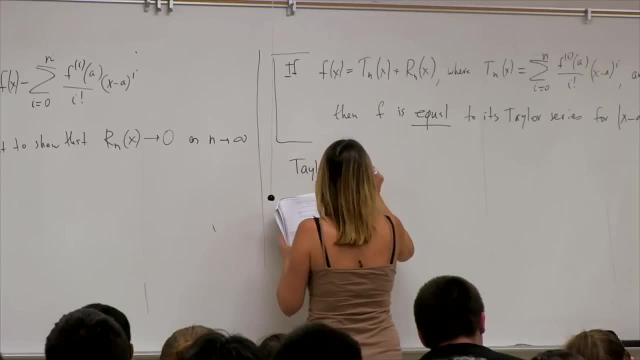 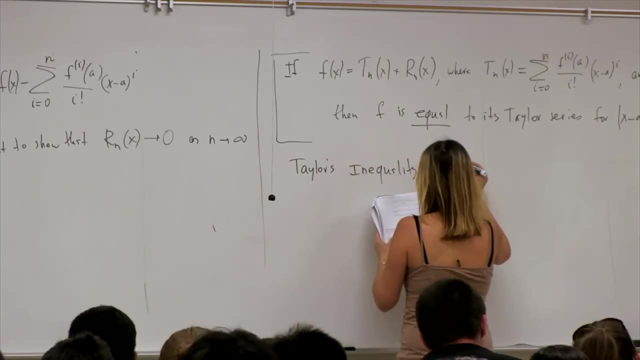 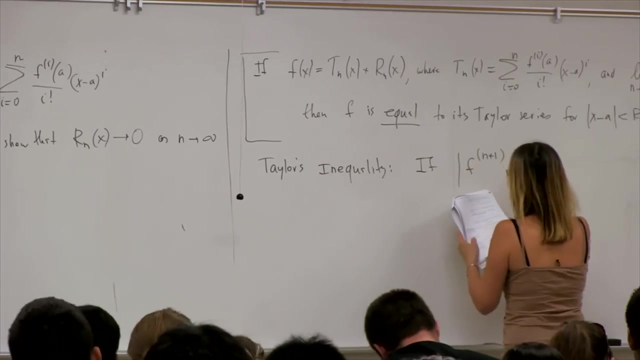 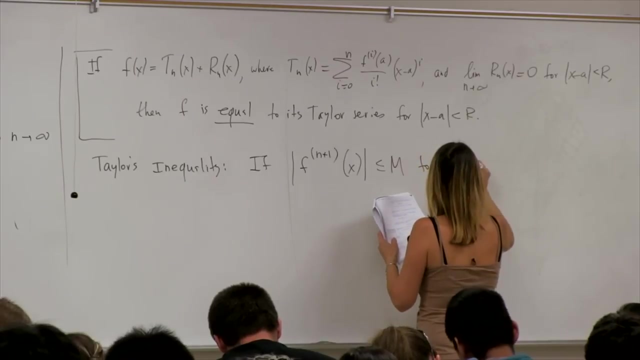 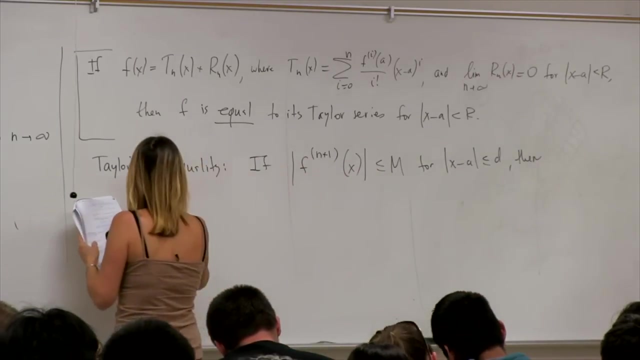 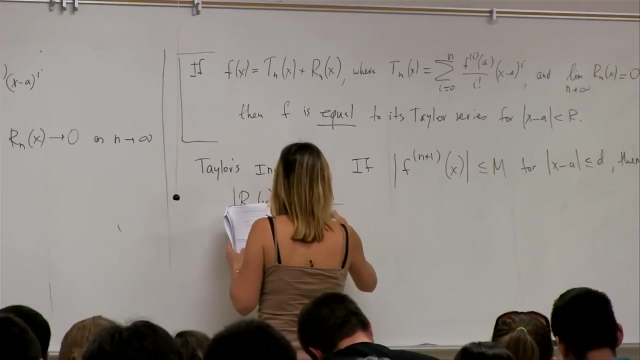 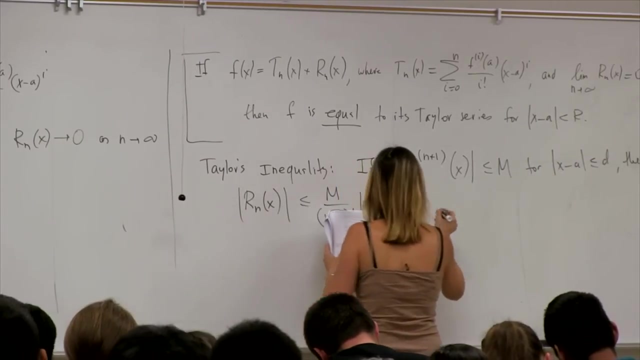 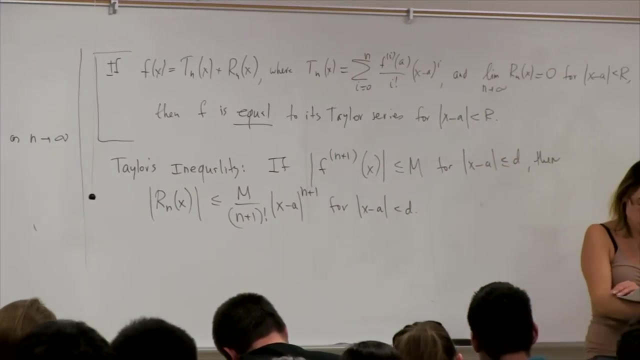 Taylor's inequality. If we can show that the derivative of order n plus 1 of x is bounded inside the radius of convergence, then Rn of x satisfies the following inequality. So I will show you, just write it down now and I'll show you what it means. So we will. 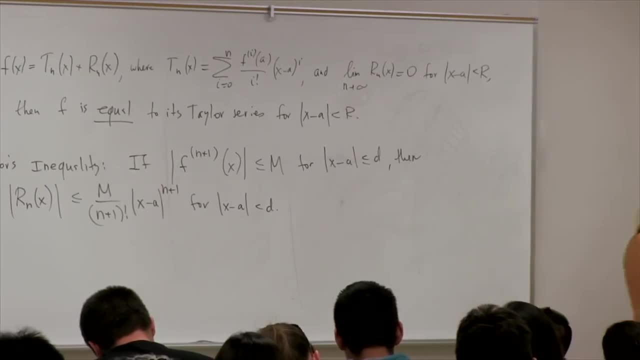 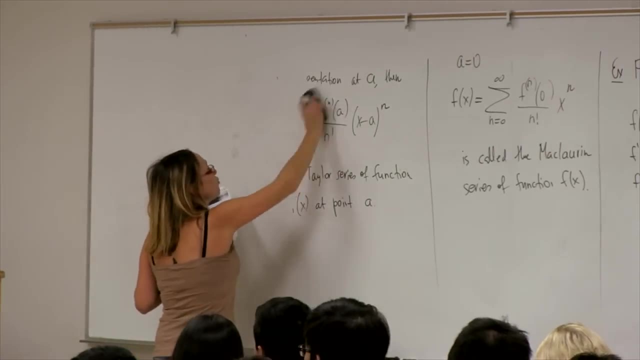 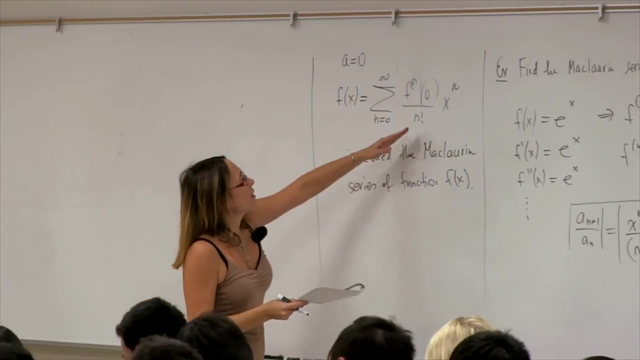 use an example. this example, the example of the exponent. So what have we done so far with the exponent? What have we done so far with the exponent? What have we done so far with the exponent? What were the logical steps? We've done two things out of three. We evaluated the terms. 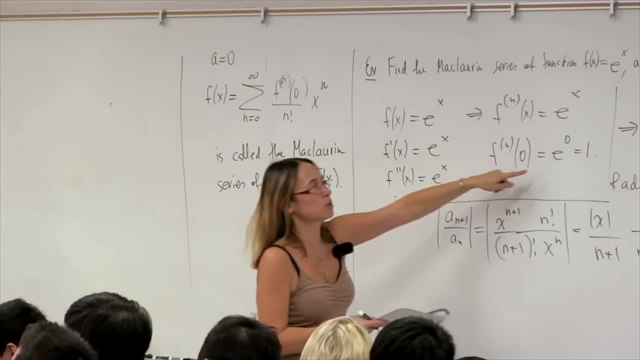 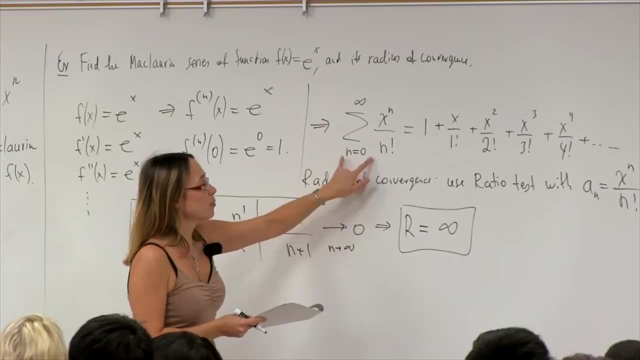 in the Maclaurin expansion by calculating all the derivatives, which are all equal to 1.. So we wrote down the Taylor series. That was one step. The second step, we calculated the radius of convergence. That was infinity. The third and final step was to show that 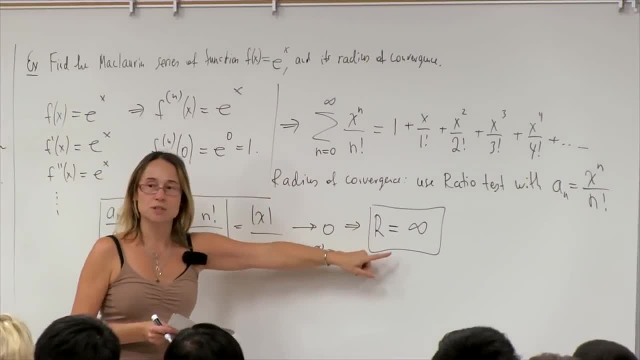 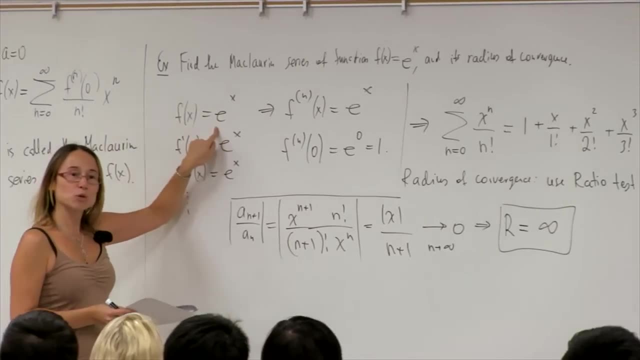 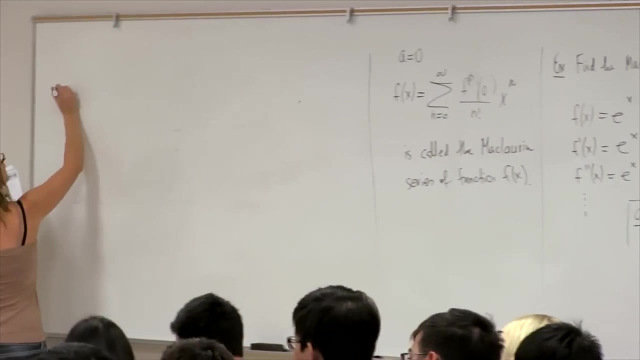 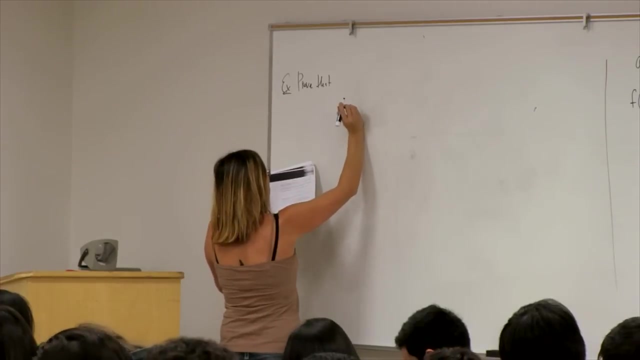 this series when it converges- and it always converges- that it indeed converges to this function, And to do that, we have to show that the remainder goes to zero. This is what we will do now: Prove that e to the. 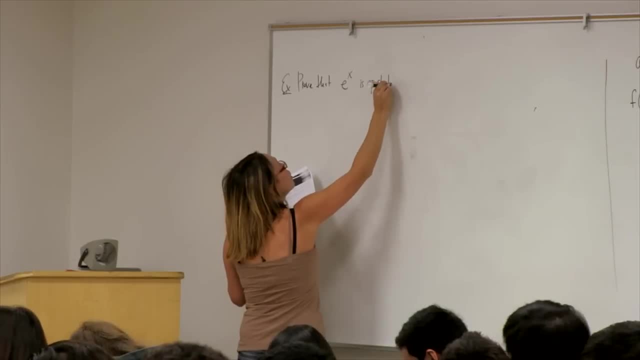 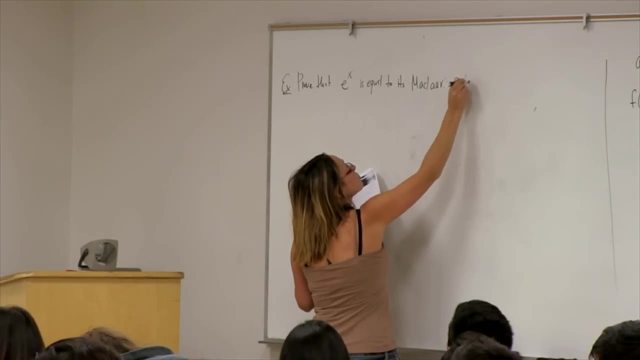 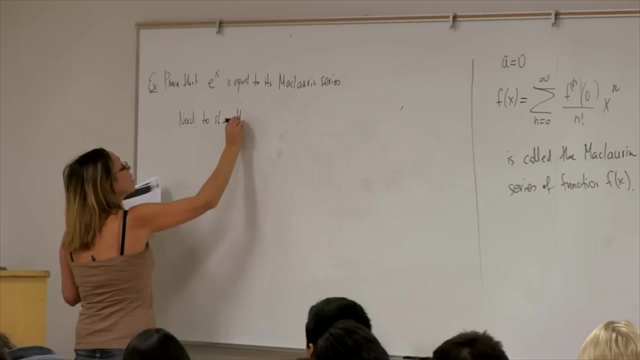 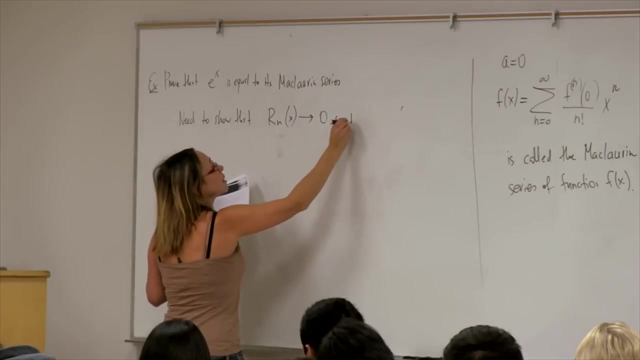 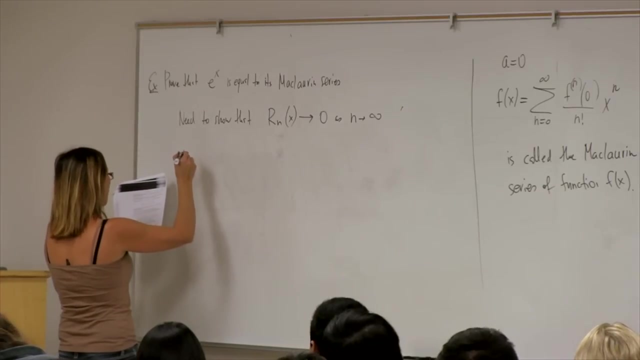 x is equal to its Maclaurin expansion. What we'll do now is we are going to point x in a series, So we need to show that Rn of x goes to zero as fact goes to infinity. So suppose we increase to infinity. So suppose we increase. 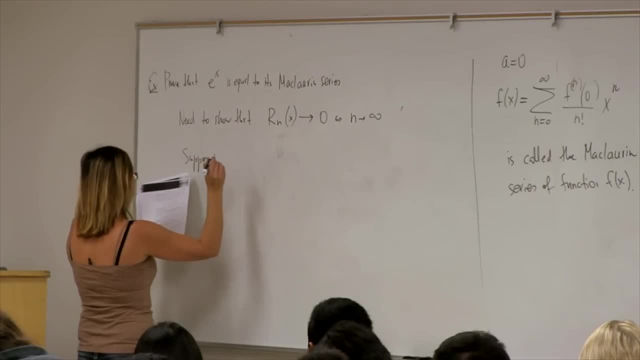 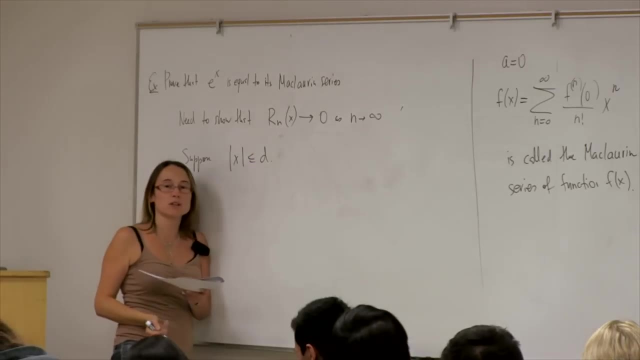 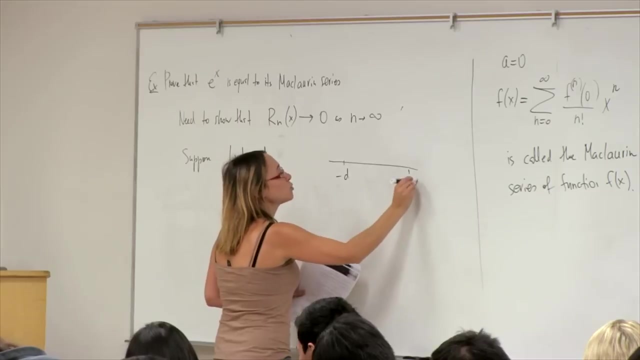 10 sharp platinum here. U else best trick is to write down m to x, and i entering positive and negative particles, And then we solve for somatic that x belongs to some interval from minus d to d. okay, we're going to put a limit to. 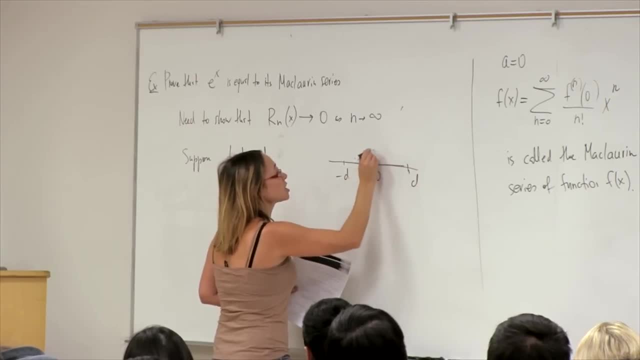 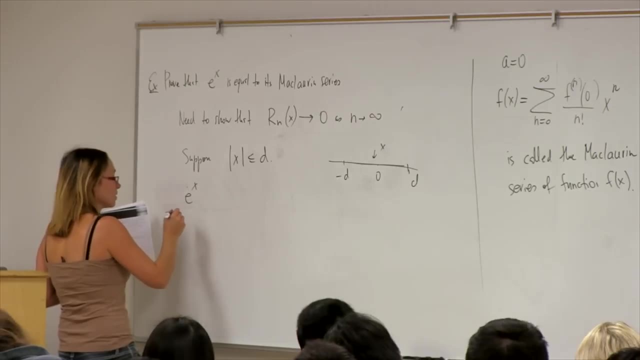 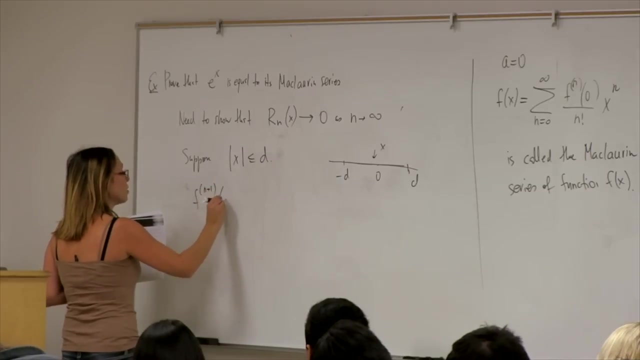 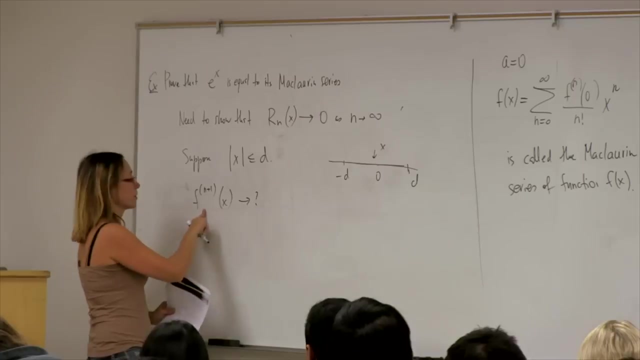 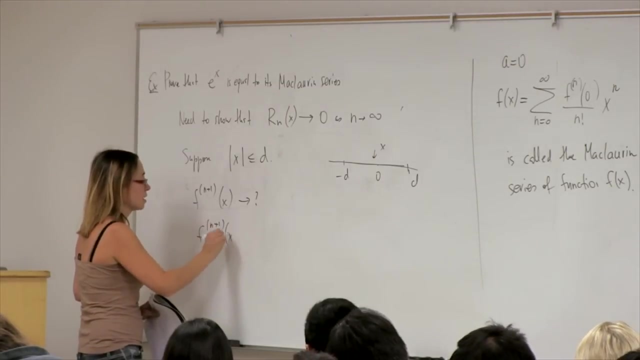 the values of x. so let's suppose that x belongs to this interval. What can we say about the nth n plus first derivative f of x inside this interval? So the derivative of the order n plus one of the exponent is actually equals to the exponent. okay, 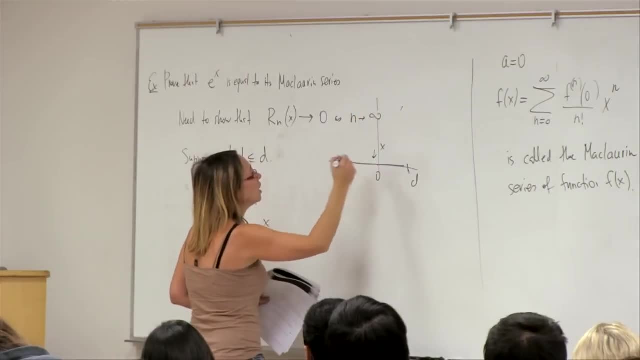 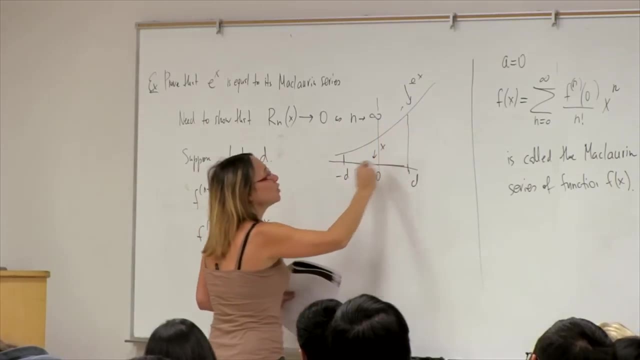 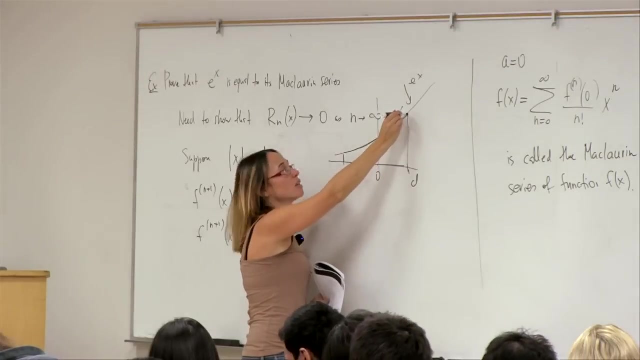 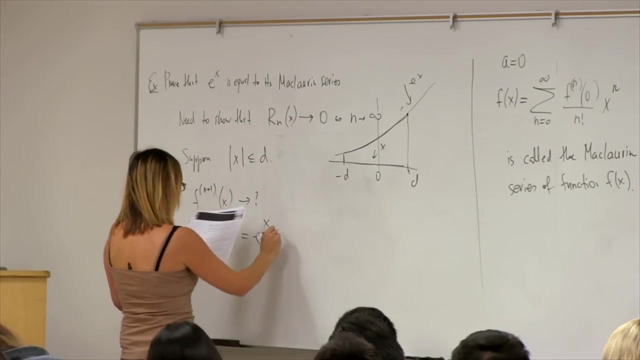 so what does the exponent do? It's some function that looks like this: This is e to the x, so, on an interval between minus d and d, it's a growing function of x, and the biggest value that it achieves is given by e to the d right. so we can. 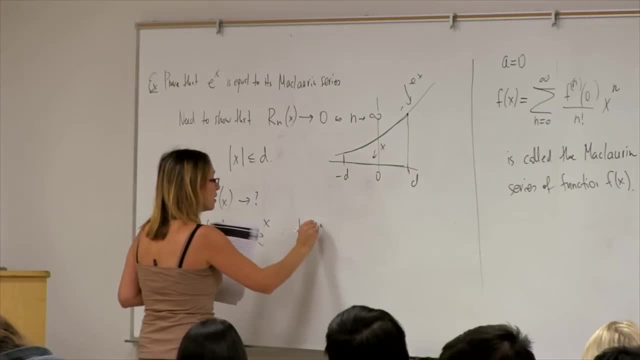 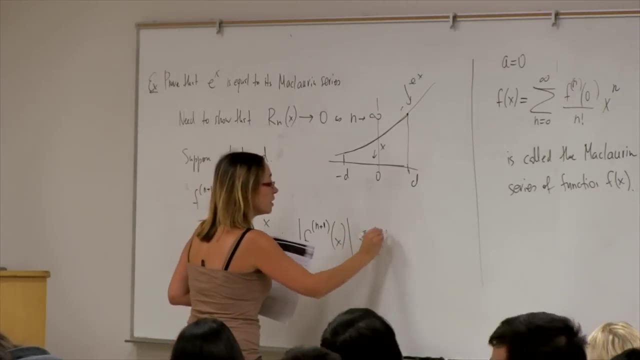 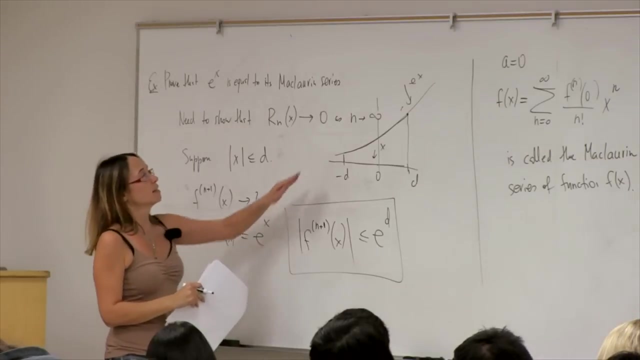 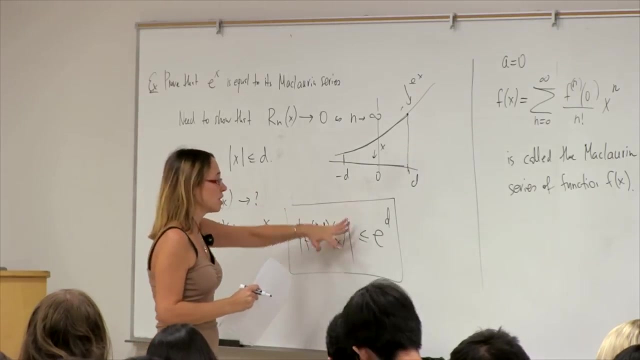 say that f, n plus 1 of x, the absolute value is less or equal than e to the d. just because this function is simply an exponent, in this case the exponent does this- it never grows larger than e to the d. okay, it's a finite quantity, that bounds. 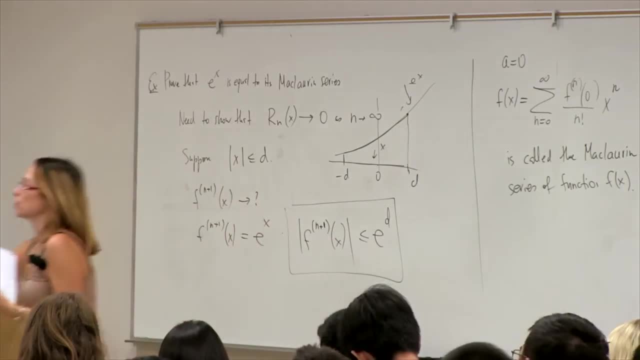 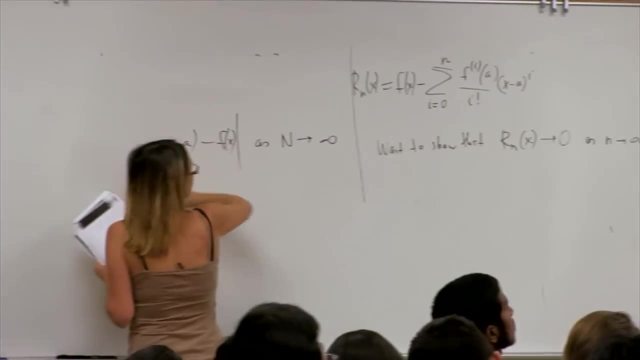 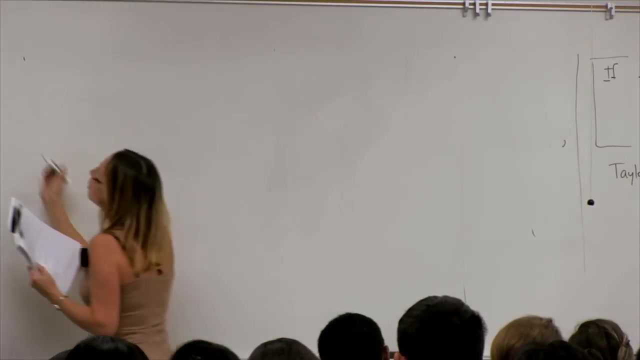 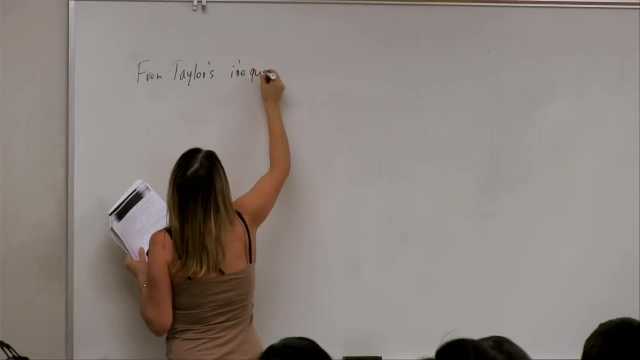 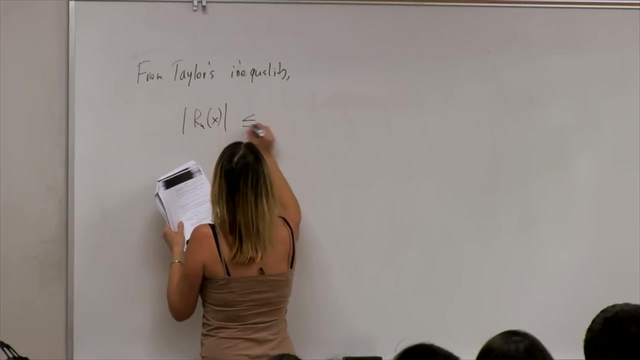 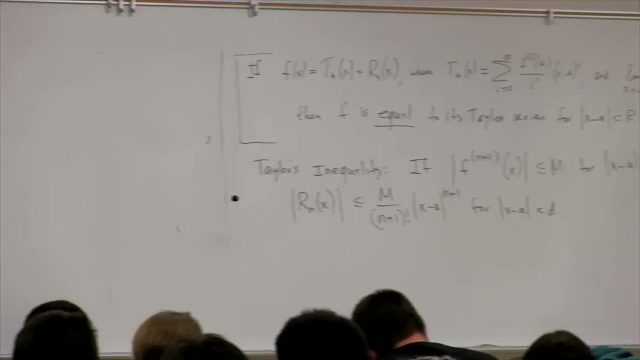 this derivative. and now we go to this theorem, to Taylor's inequality. from Taylor's inequality, we know that the remainder on d is less or equal to m, the bound for the derivative divided by this times this: so we have e to the d. okay, n plus 1,. factorial x: n plus 1. 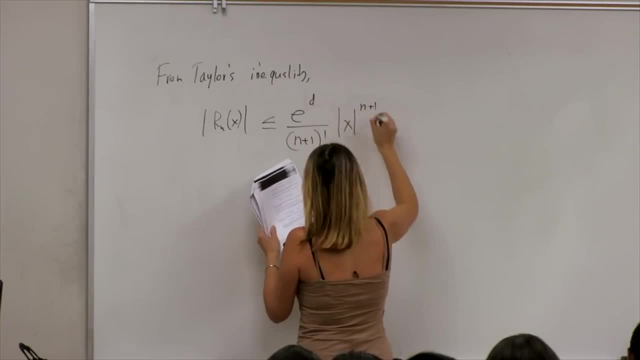 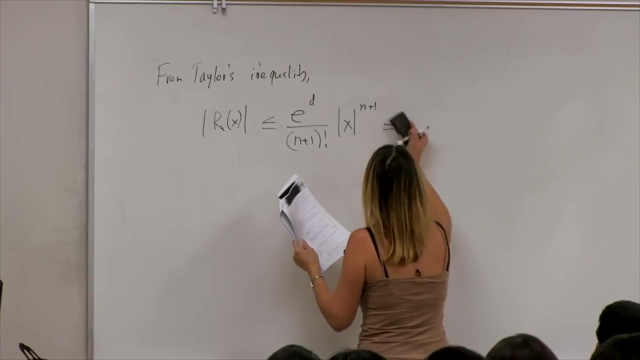 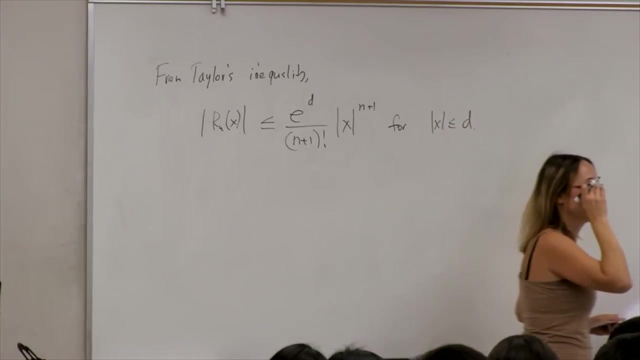 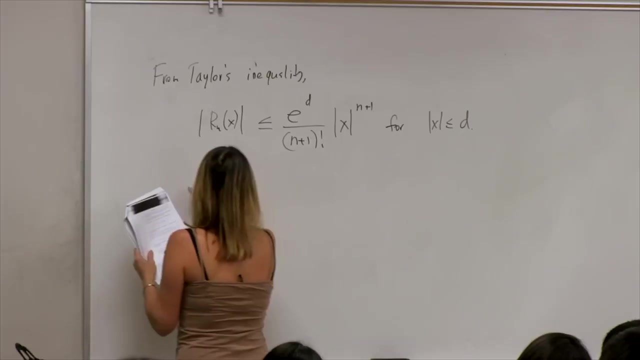 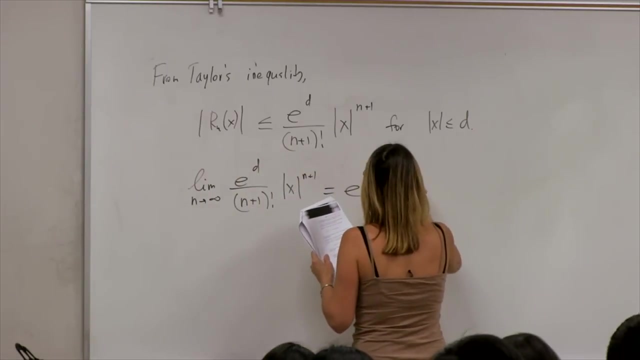 n plus 1, factorial x n plus 1. So for x in the interval bounded by d. So this is the So this is the value of m. Now we take the limit, The limit, as n goes to infinity- of this quantity, e to the d? n plus 1. x n plus 1 is the same as e to the d, because that's a constant x n plus. 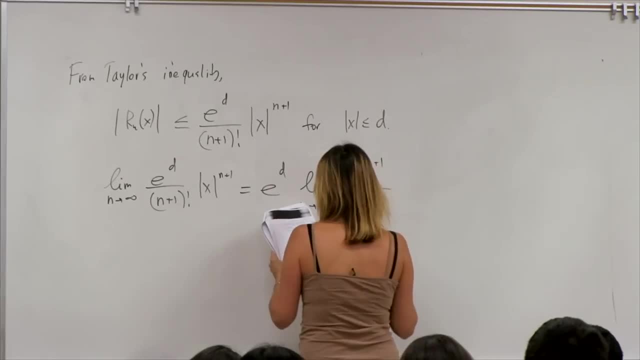 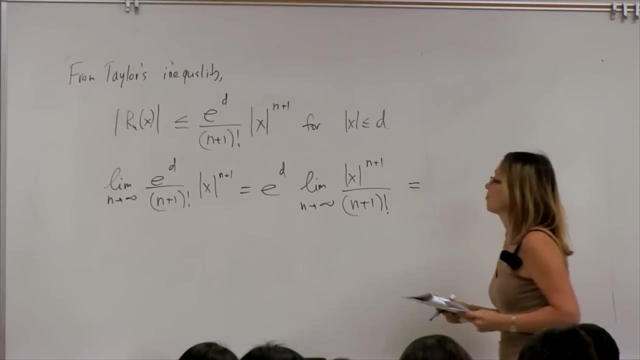 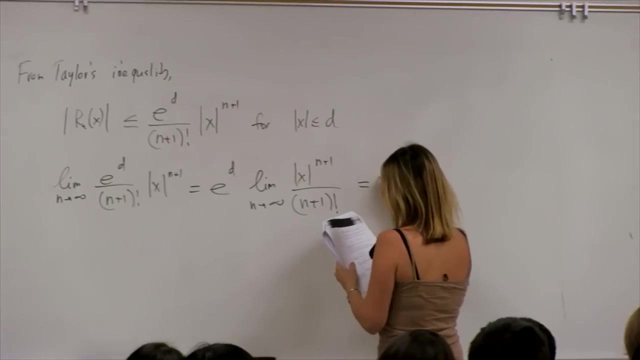 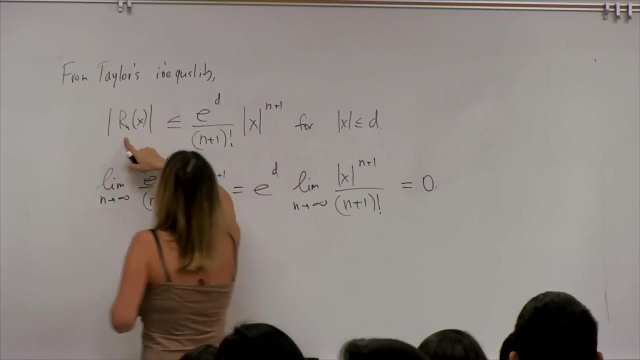 1 factorial. Okay, what's the limit of this quantity? We've had this example before and it's equal to 0, okay, So, therefore, because the remainder, the absolute value of the remainder, is smaller than this quantity and this: 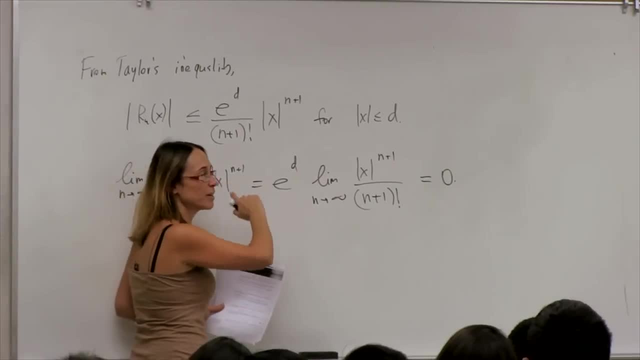 quantity is less than because of theении of the istrand…. the absolute value of the remainder is even smaller than this quantity, And this quantity quantity tends to 0,. by the squeeze theorem we can say that the remainder itself goes. 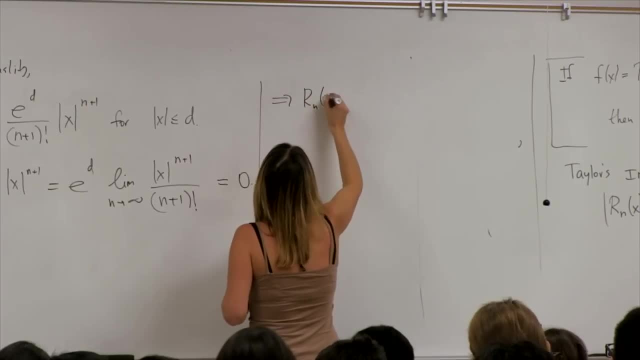 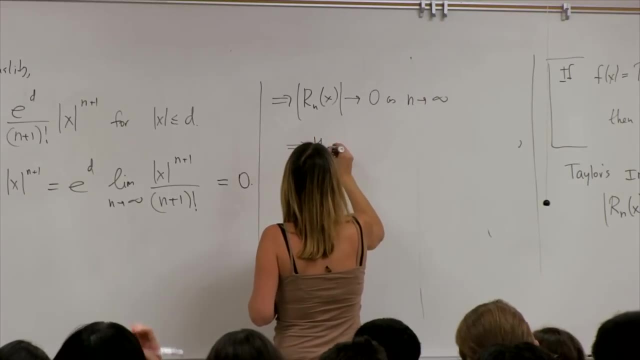 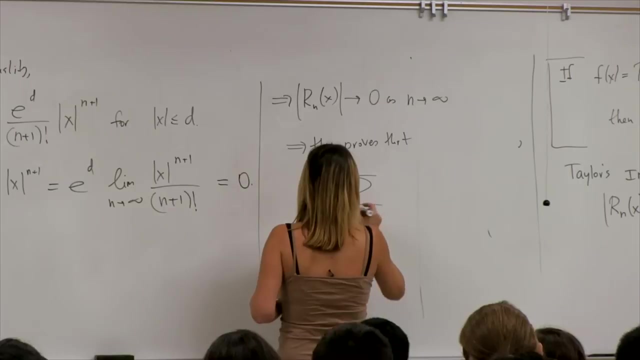 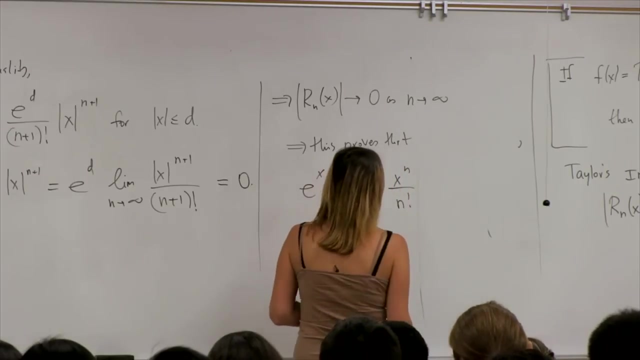 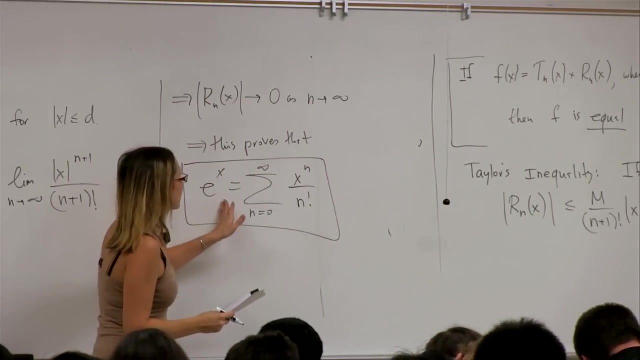 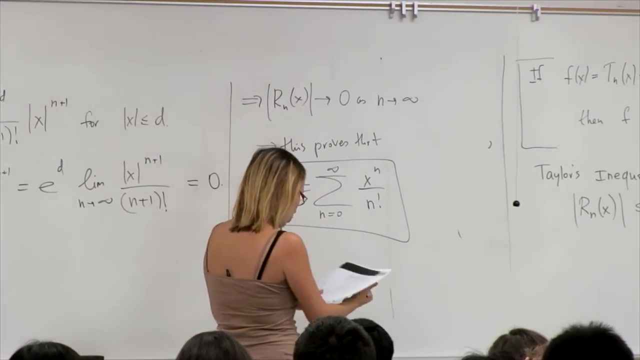 to 0. Therefore Rn of x goes to 0 as n goes to infinity. So this proves that e to the x is equal to its Maclaurin expansion. So this is a famous formula and it allows many calculations that otherwise would be impossible. I'll show you today what we can do with this. 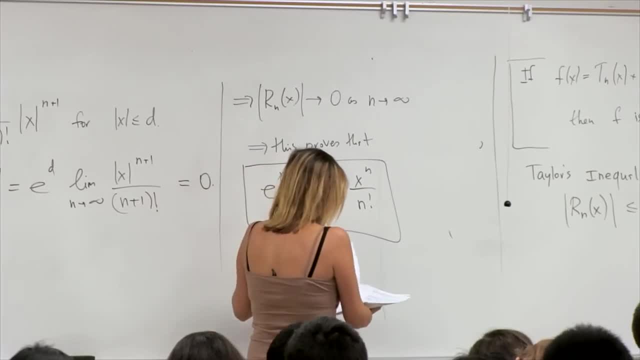 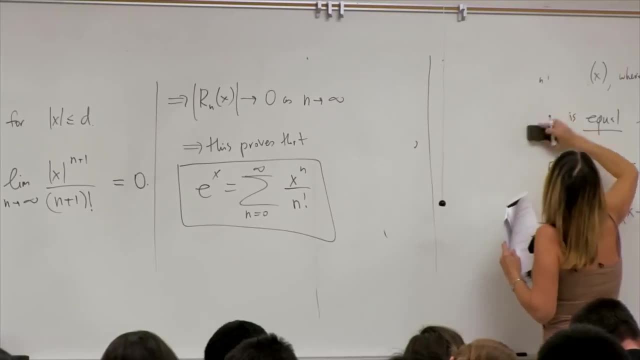 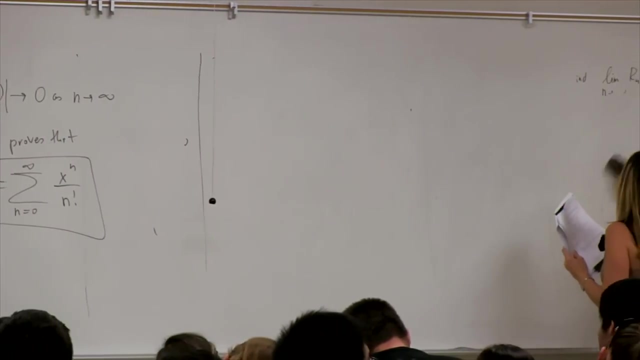 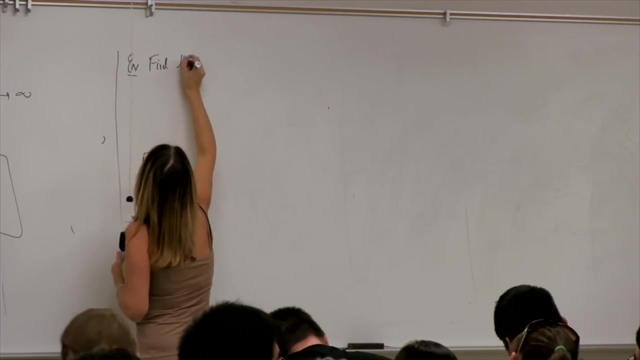 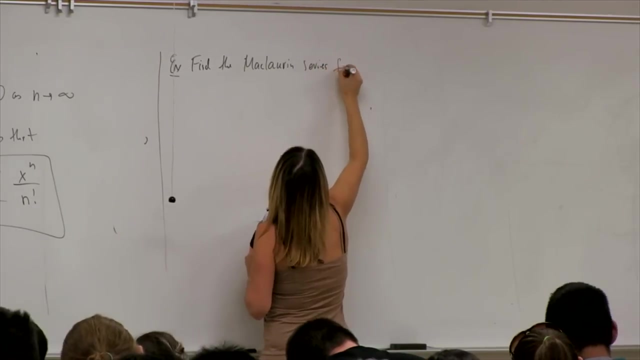 just for this particular function, the exponent. So I want to show you some other Taylor's series of different functions. You can see that. you will see that it's sometimes quite easy to calculate them. So as the next example, we'll find the Maclaurin series for function. 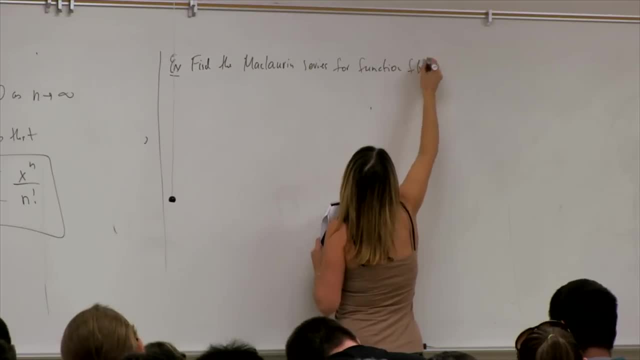 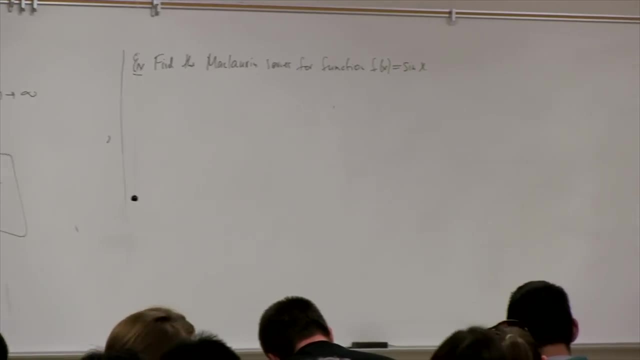 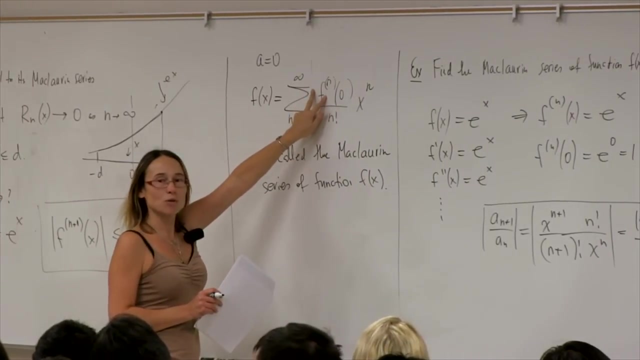 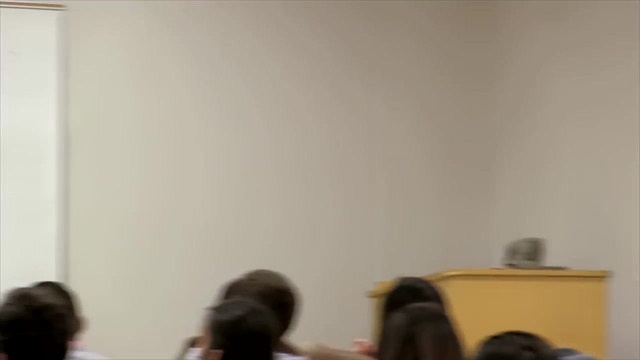 f, f of x given by sine x. So go back to the general formula. We need to populate the series with the n-th derivatives of sine at 0. So the 0-th derivative is the same as f of x is sine x. 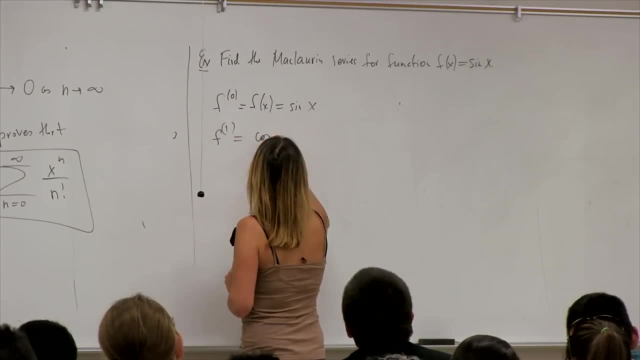 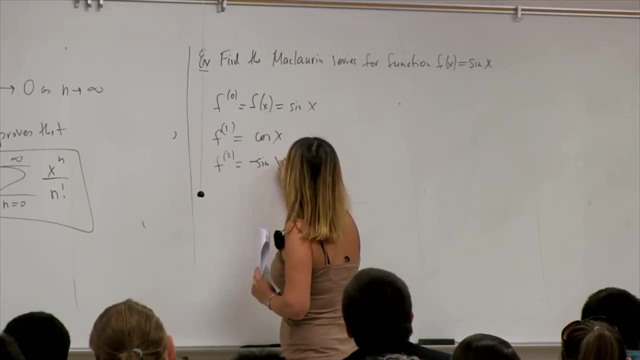 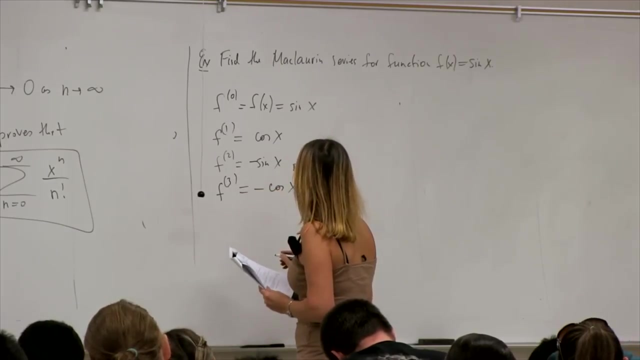 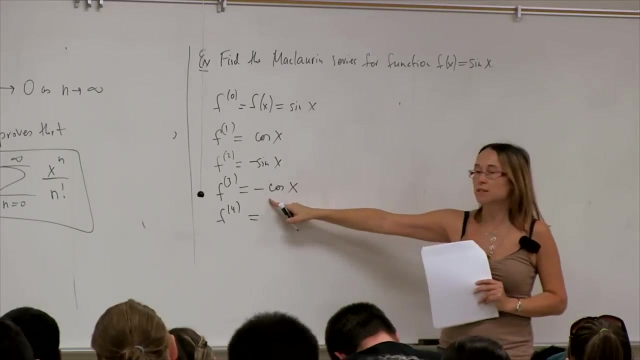 The first derivative is cosine x, right. The second derivative is minus sine x. The third derivative is minus cosine x. The fourth: what is the derivative of minus cosine x? Sine x. And you can see that this closes the circle. 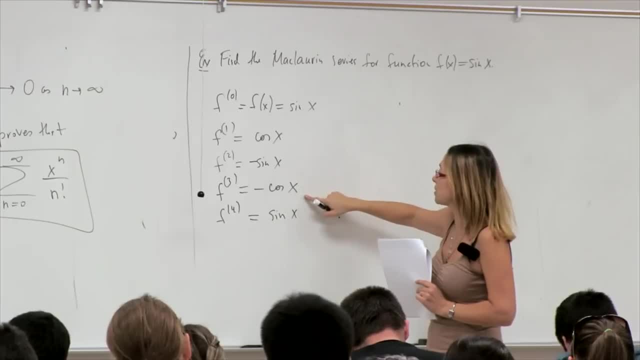 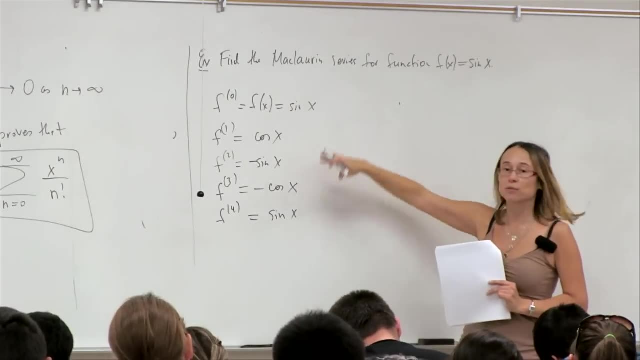 So we go from sine x to cosine x, From sine to cosine to minus, sine to minus cosine, And then back to sine, and it repeats. So as we do it for an infinite number of derivatives, we're going to have this repeating cycle. 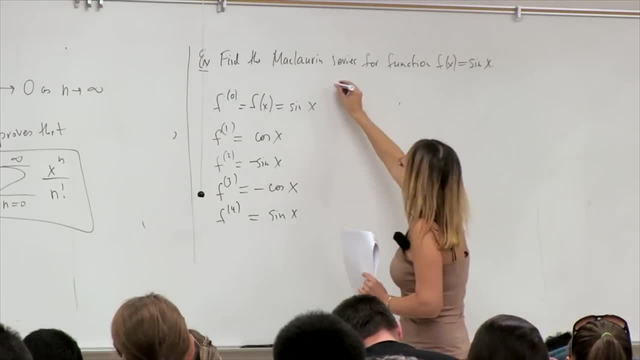 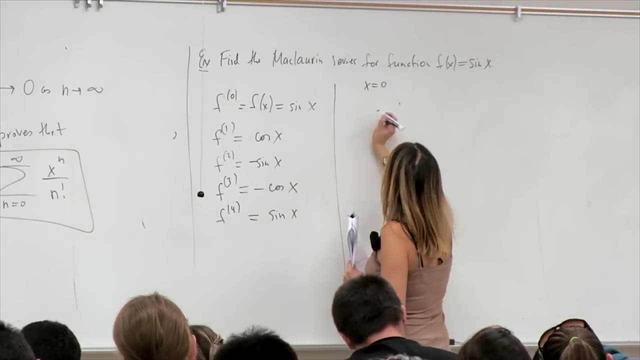 So there are going to be no other functions, just these Here. I don't need these for any x. I need to evaluate them at x equals 0.. So to set x equals 0, we have f of 0 is 0. 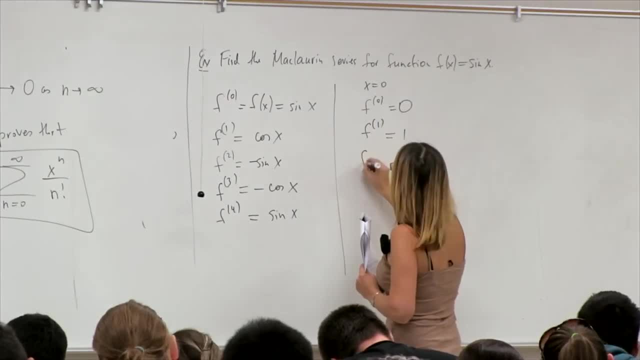 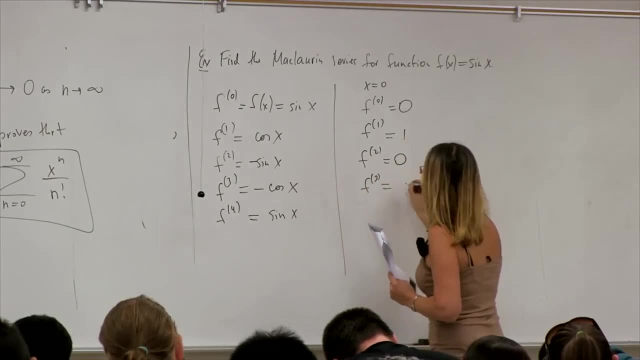 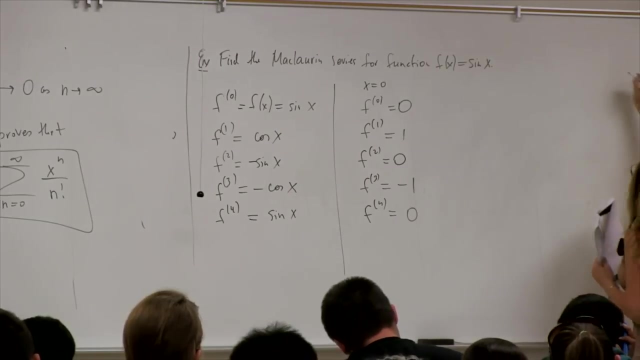 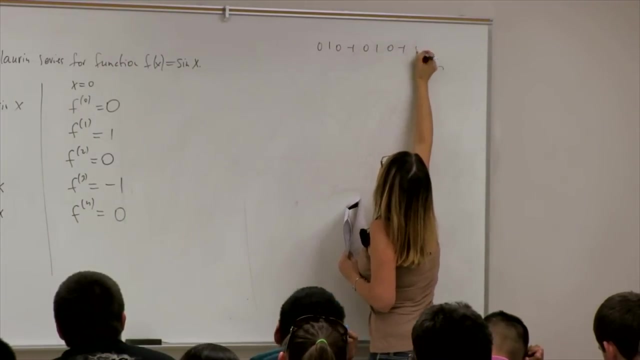 The first derivative is 1.. The second derivative is 0.. The third derivative is minus 1.. And the fourth derivative is 0 again, And it's going to repeat. So what is the sequence? 0, 1, 0, minus 1, 0, 1, 0, minus 1, 0, 1, and so on. 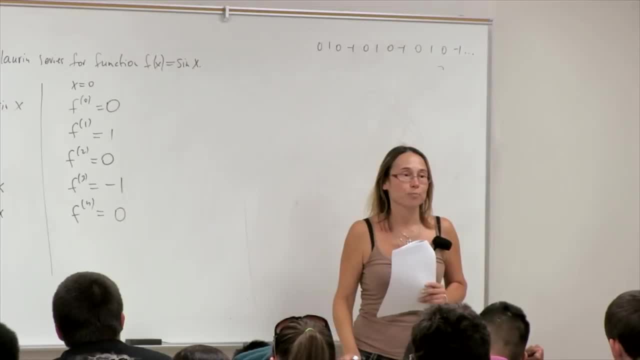 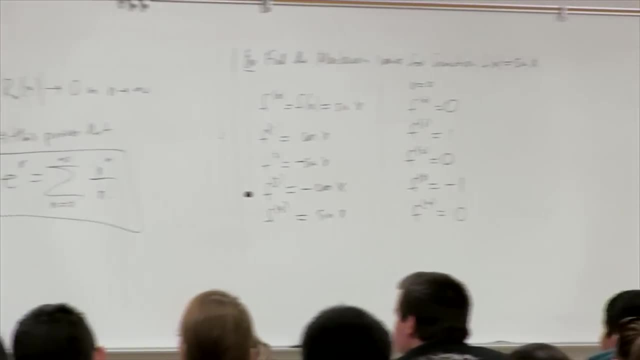 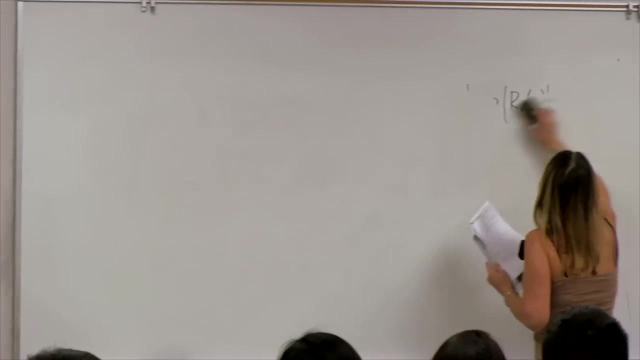 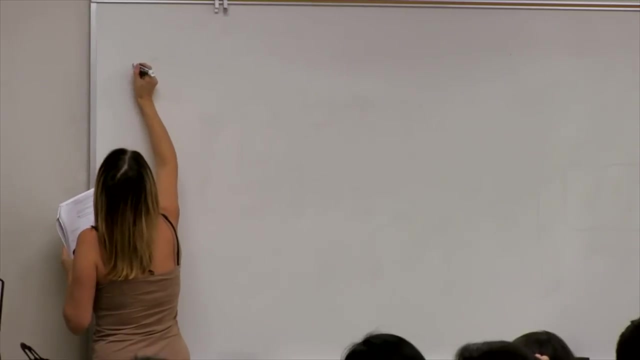 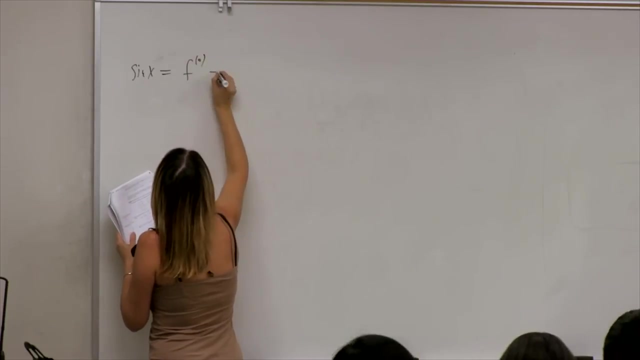 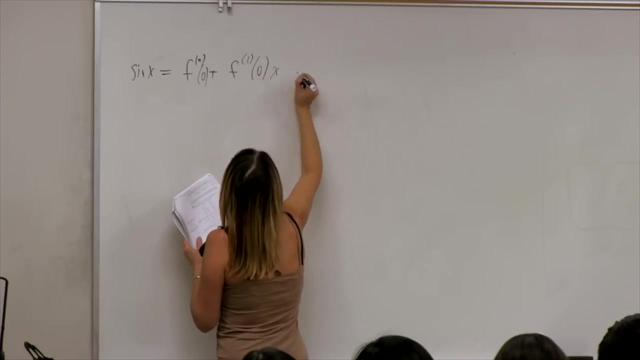 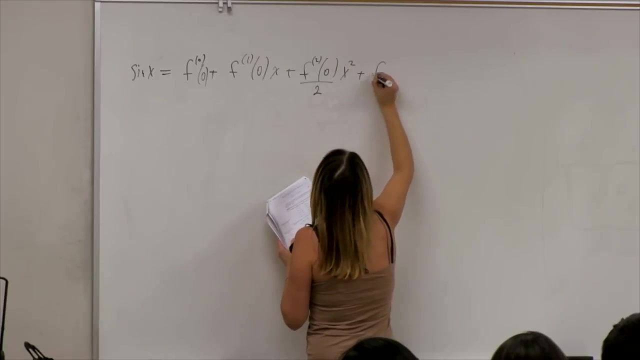 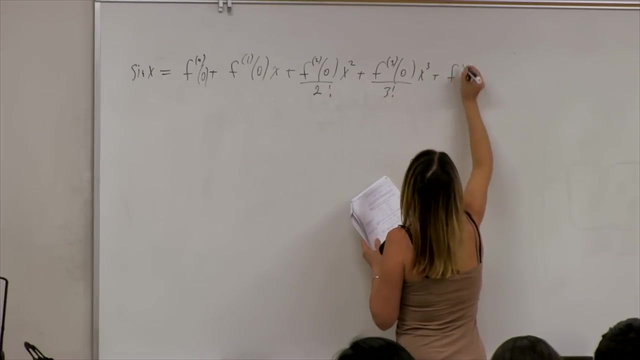 These are all the derivatives of sine evaluated at 0.. OK, So let us use this information to write down the Taylor series for this function. So sine x is given by f of 0.. f of 0,, 1 of 0, x. 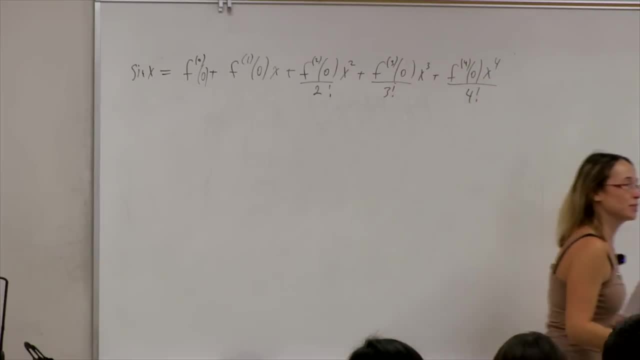 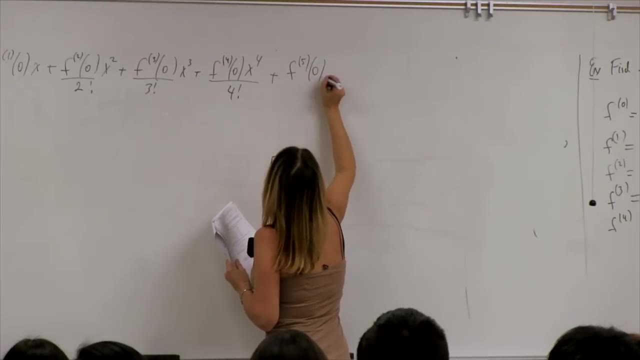 This is the general expansion Here. I haven't put any information about the derivatives yet. I'm going to do it in a second. Let me just Go to the fifth term. Fifth 5: factorial right And so on. 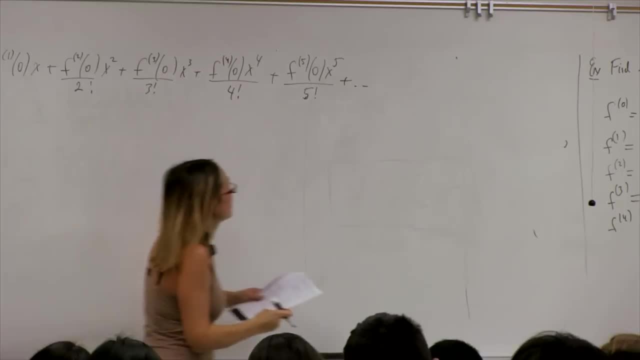 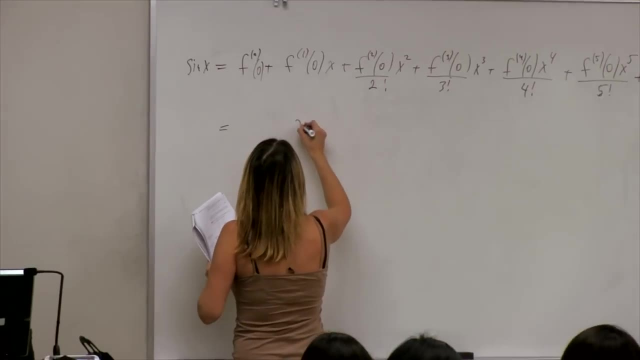 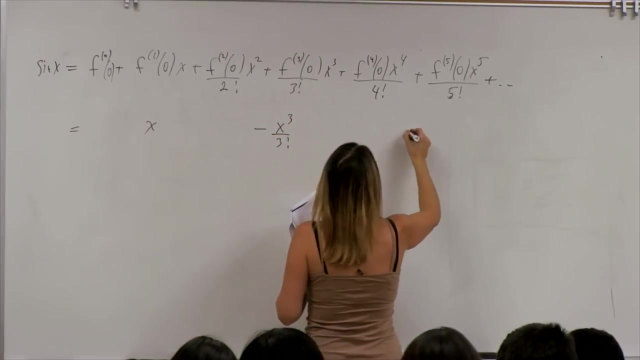 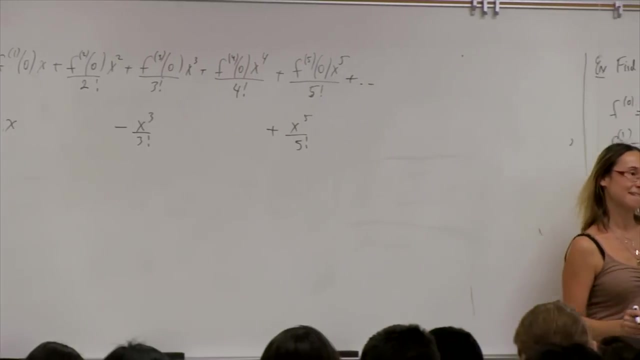 Now we are going to populate it. The first one is 0, 1, 0, minus 1.. So I have nothing. I have 1. Nothing Minus 1. Nothing, 1. Nothing. What's the next term? 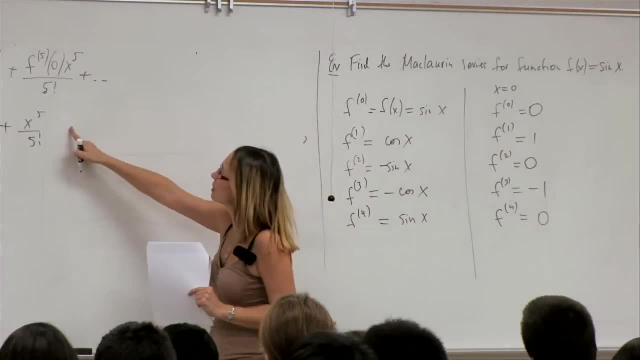 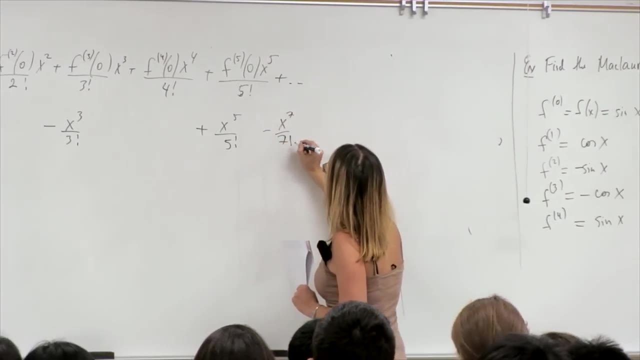 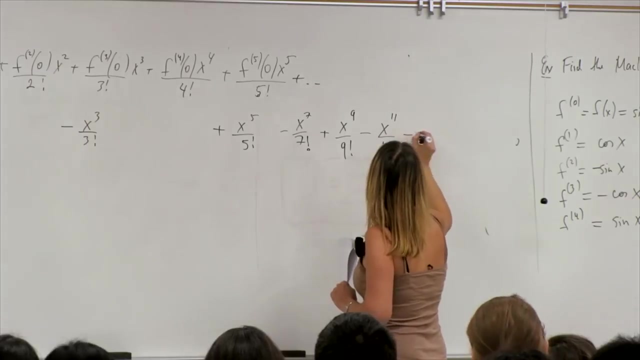 What's the next term? What's the next non-zero term? Yes, Absolutely: 7 factorial plus x to the 9, 9 factorial minus x to 11, 11 factorial and so on. Right, You can see a beautiful pattern here too. 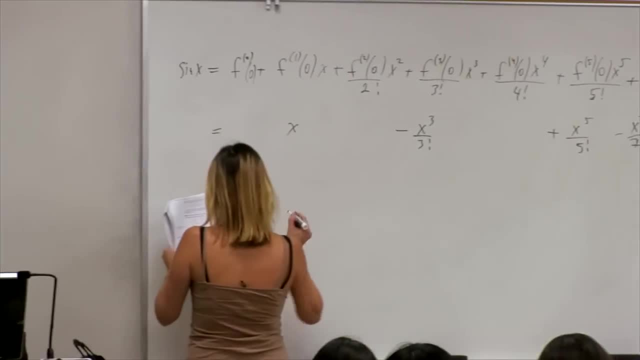 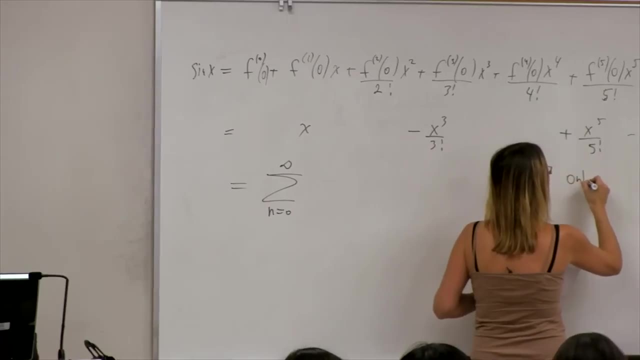 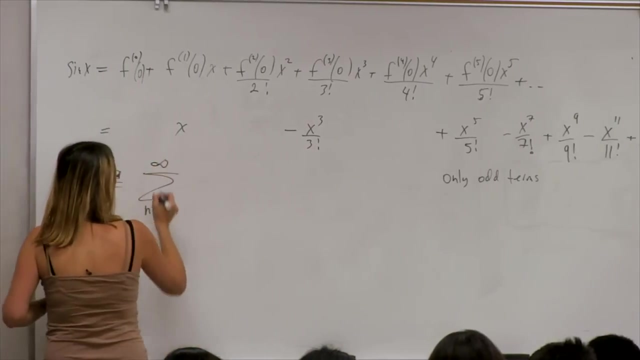 How do we write it? It's a sigma notation, So you can see that we only have only odd terms. OK, So if n goes from 0 to infinity, it goes 0,, 1,, 2,, 3,, 4,, 5.. 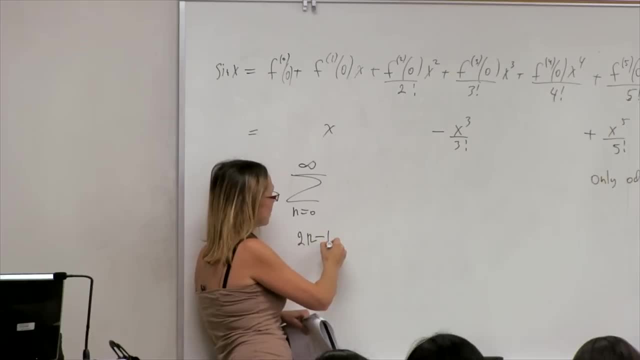 I want to look at the combination 2n minus 1, plus 1.. What does this do? OK, When n is 0, this is 1.. When n is 1, this is 3.. When n is 2, this is 5.. 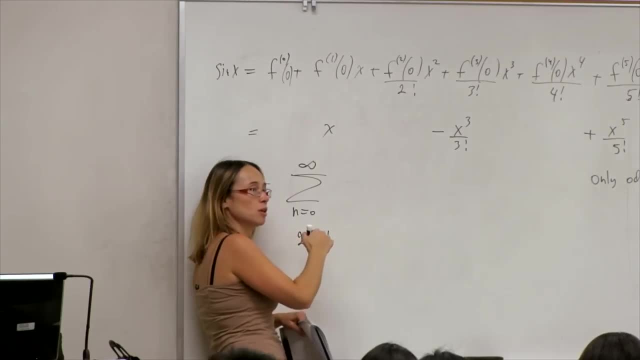 So, as n goes 0,, 1,, 2,, 3,, 4,, 5,, this goes 1,, 3,, 5,, 7,, 9,, 11.. So this is a machine that only creates odd numbers. 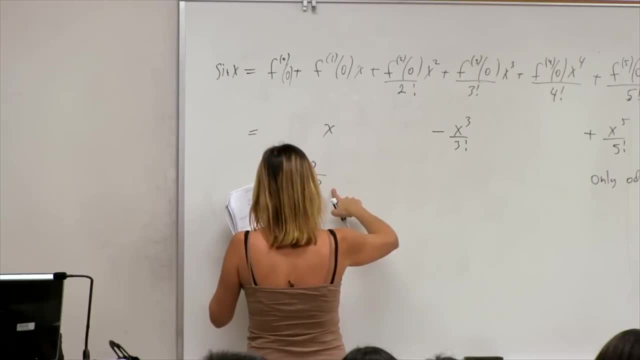 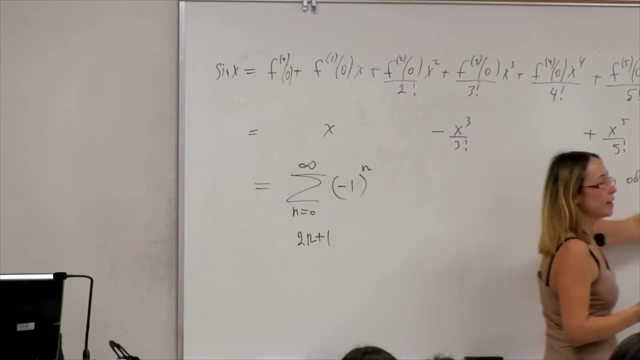 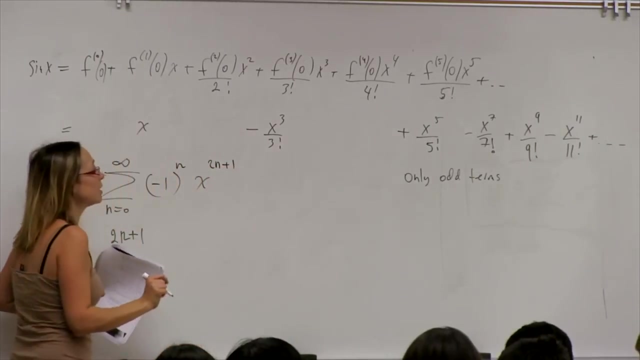 OK, So I'm going to use that. I'm going to have the alternating sign incorporated like this: x comes in the power of 2n plus 1.. These are all the odd powers of x And in the denominator I have the matching factorial. 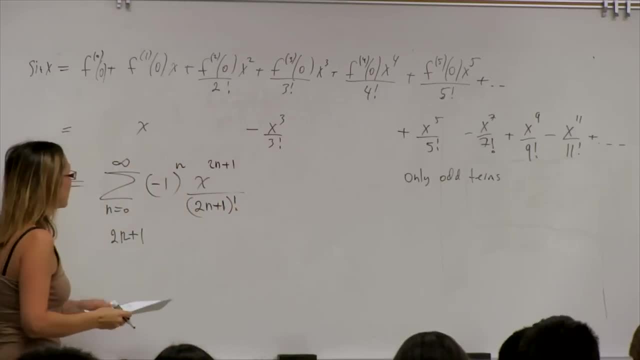 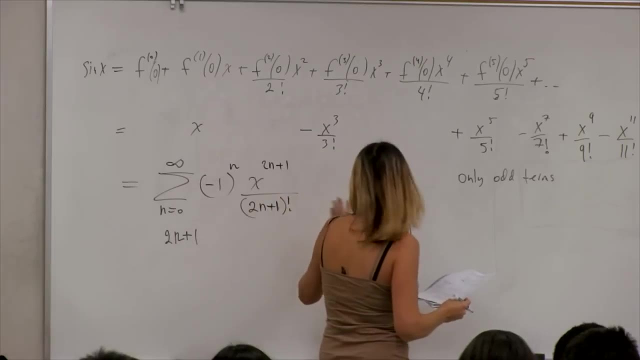 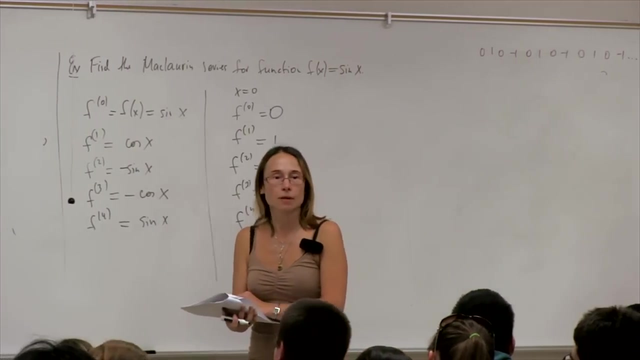 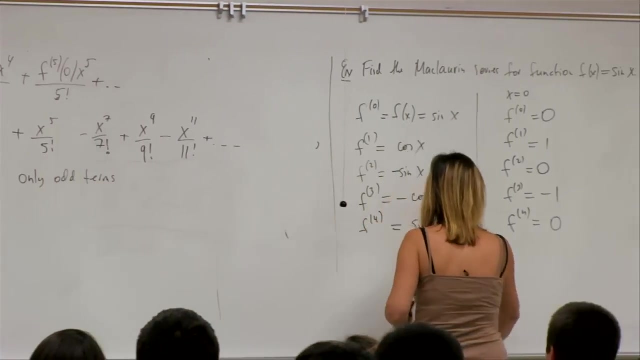 OK, So this is the Maclaurin series of the function sine x, written in the denominator In terms of sigma. notation Questions: OK, Now how about cosine? So, in principle, every time you do this- this is a nice way of doing it systematically- 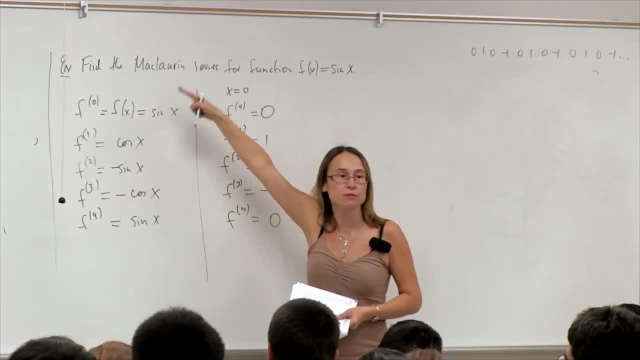 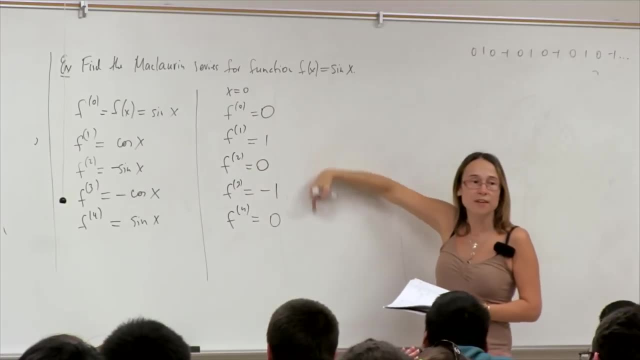 On the left you write the function, its derivative, second derivative, third derivative, in general. So the next line is the differentiation of the previous line. On the right, you take all these things and evaluate them at a whatever your center of your series is. 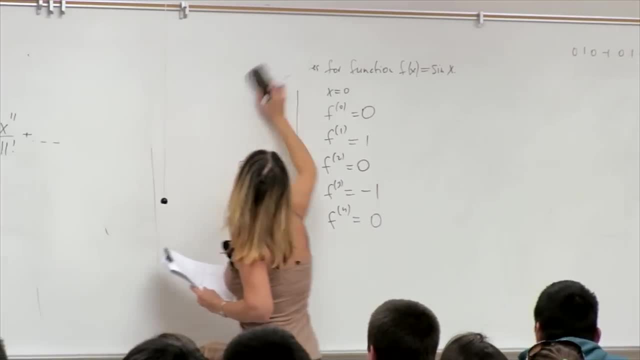 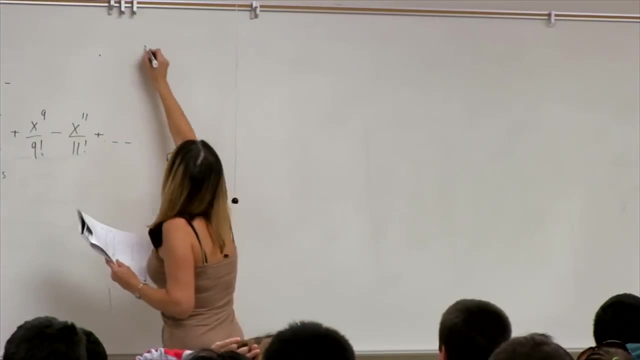 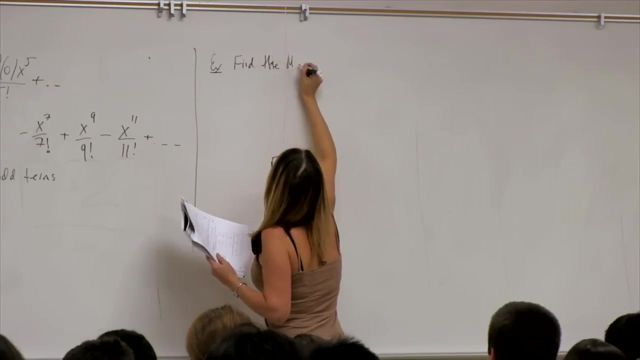 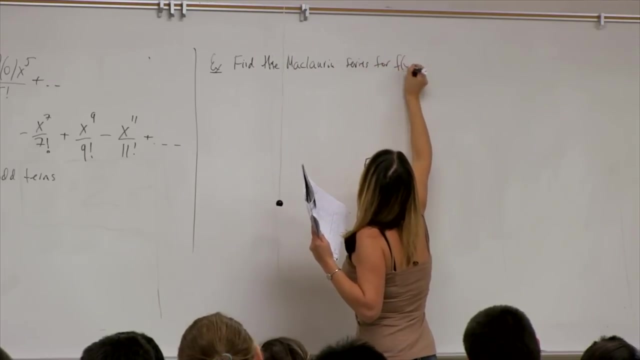 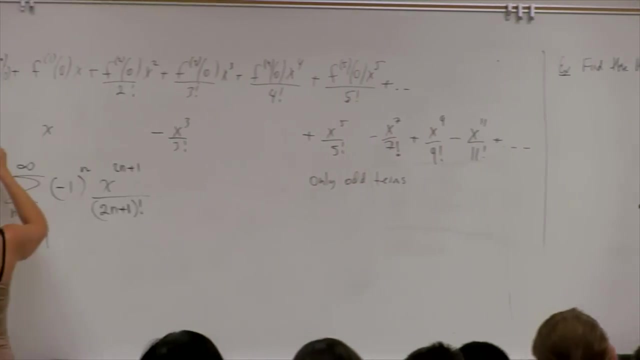 OK, So when we do it for cosine, we could do the same, But we don't do it, We do something that is easier. So the example: Find the Maclaurin series For f of x equals cos x. So what I'm going to do, I'm going to take this representation of sine. 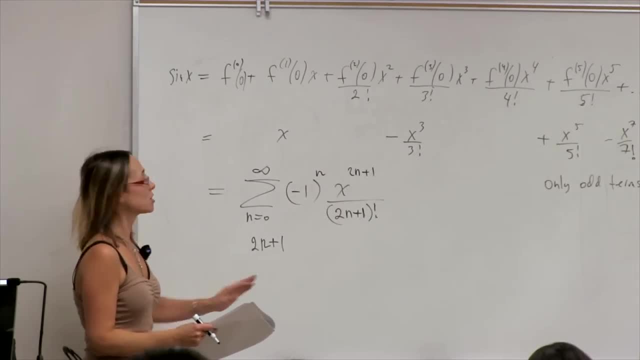 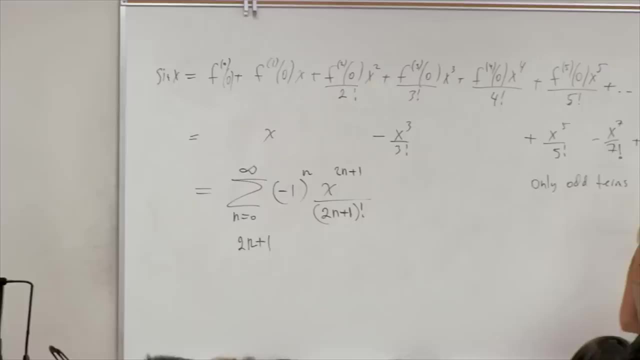 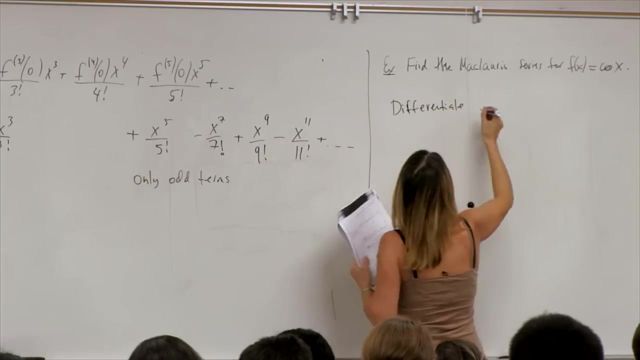 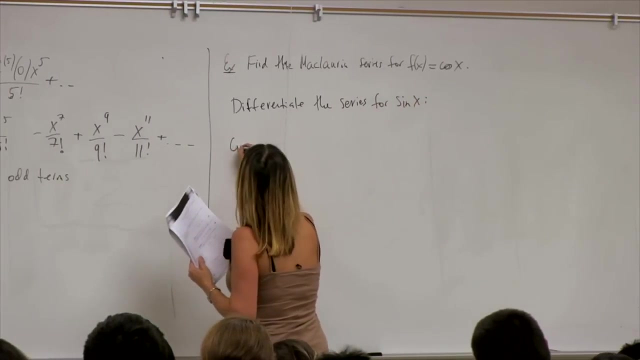 And, as you remember, we can actually differentiate power series. So by differentiating the left hand side, I get cosine. And these are power series, right? They are very easy to differentiate. So differentiate The series for sine x. So on the left, I get cosine x. 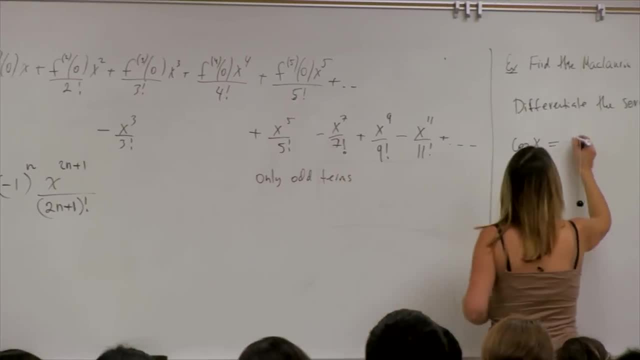 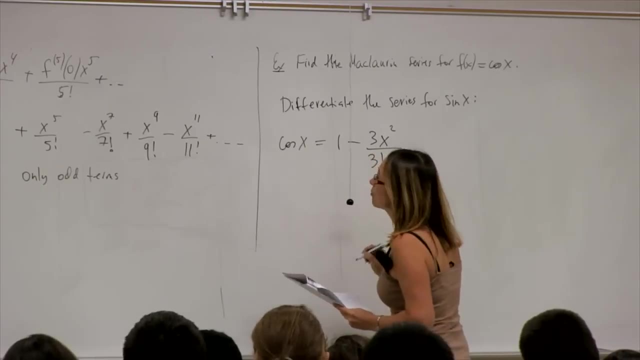 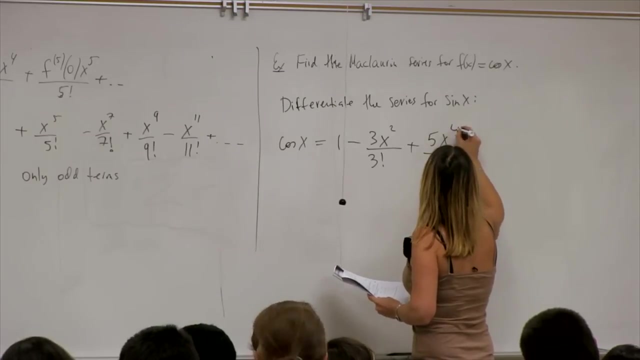 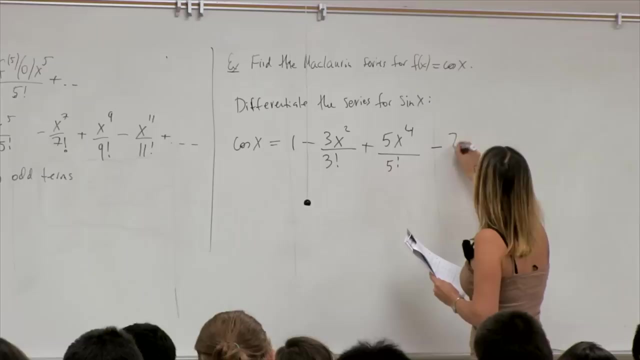 On the right, I have 1.. OK, Minus 3x, squared 3 factorial. Plus 5x. fourth over 5 factorial. I'm differentiating these terms, OK, Explicitly, without the sigma thing: Minus 7x to the sixth. 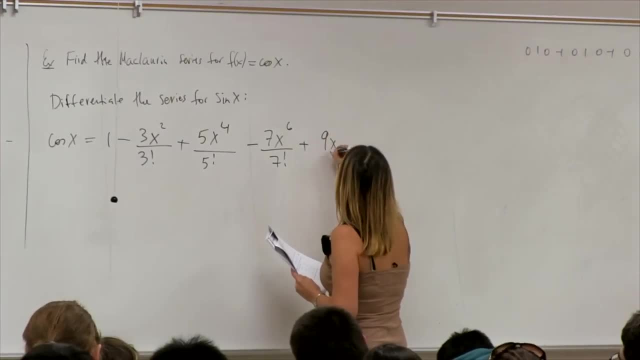 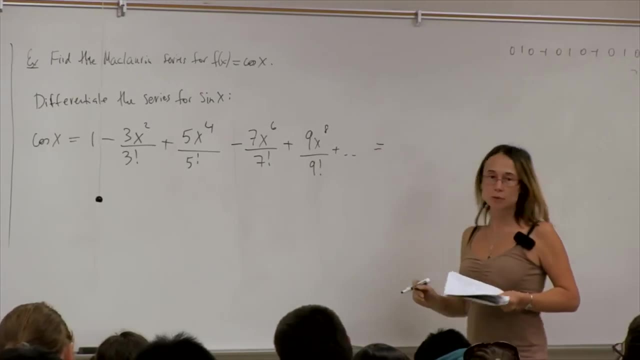 7 factorial, Plus 9x to the eighth, 9 factorial. That's enough, OK, So, and you can see that we have a nice cancellation. You have 3 factorial divided by 3.. 5 factorial divided by 5.. 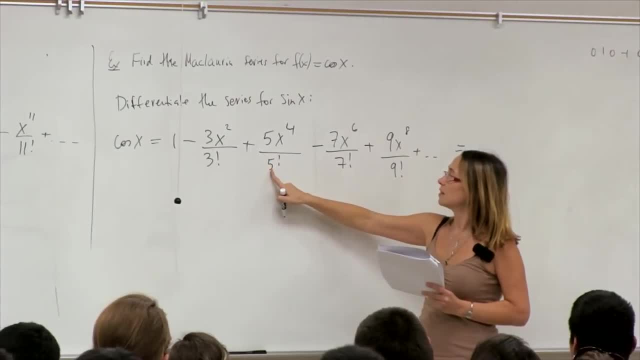 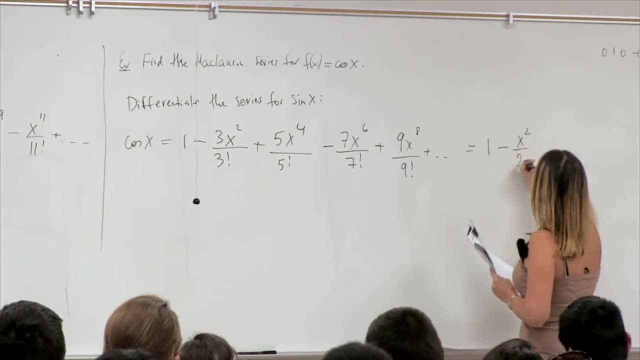 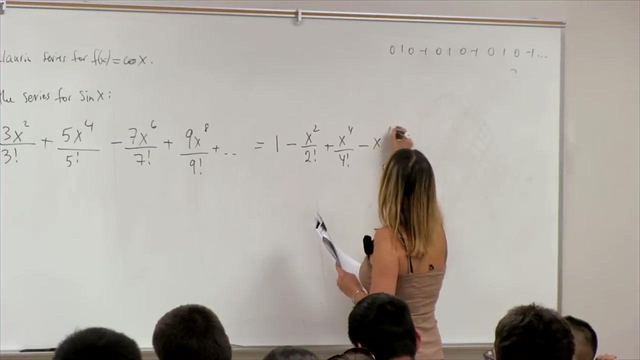 So What can I replace it with? This is just what? 4 factorial right. So I have 1 minus x squared over 2 factorial. Plus x to the fourth, 4 factorial, Minus x to the sixth, 6 factorial. 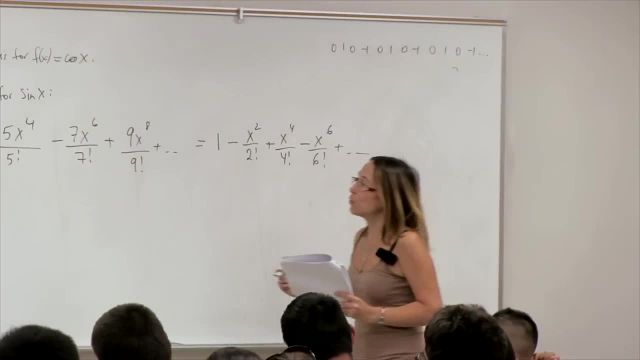 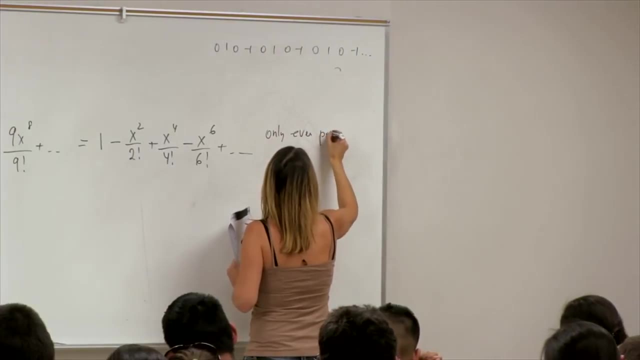 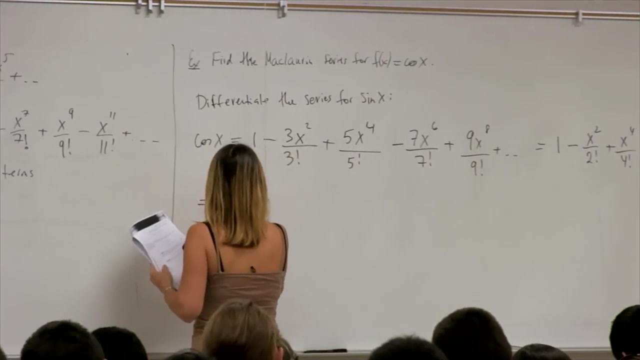 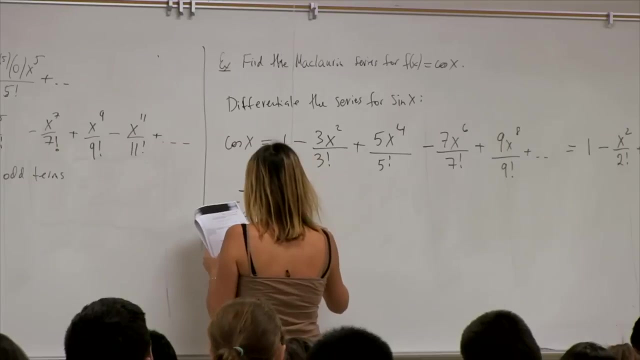 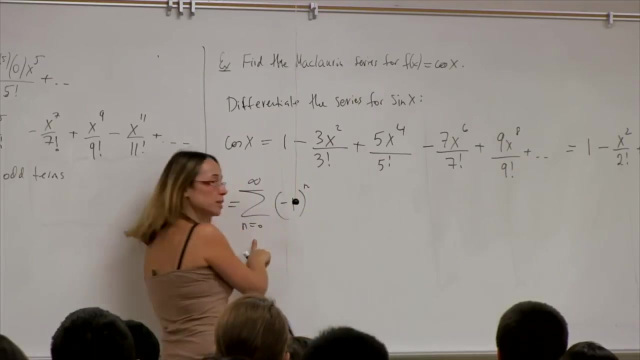 And so on. OK, So now we only have only even powers. So I'm going to write it down as the sigma notation. I have the alternating sign, But I don't want all the n's, I only want even n's. 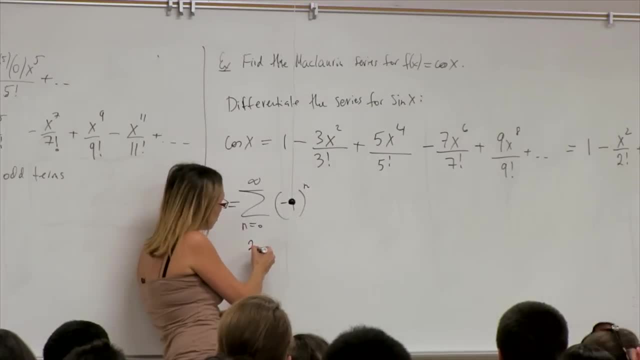 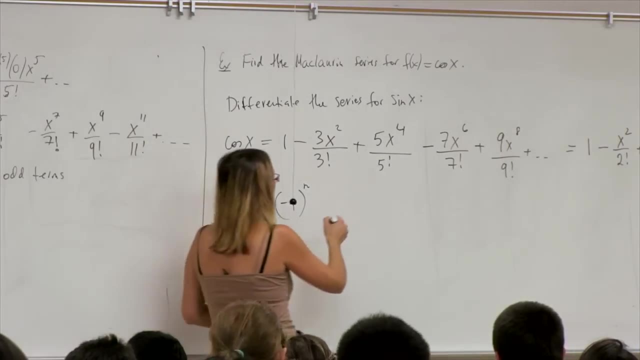 So, as n goes 0,, 1,, 2,, 3,, 4,, 5.. 2n Goes 0,, 2,, 4,, 6,, 8. 10. Right, So this is what I want. 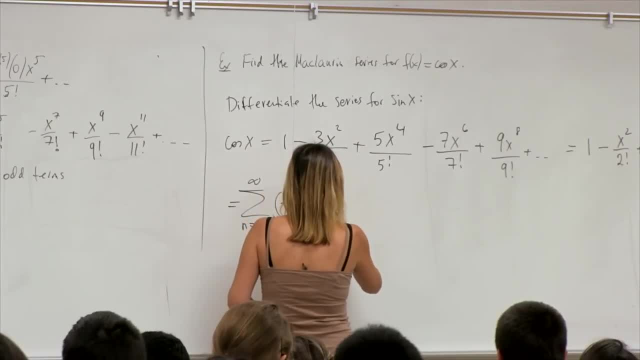 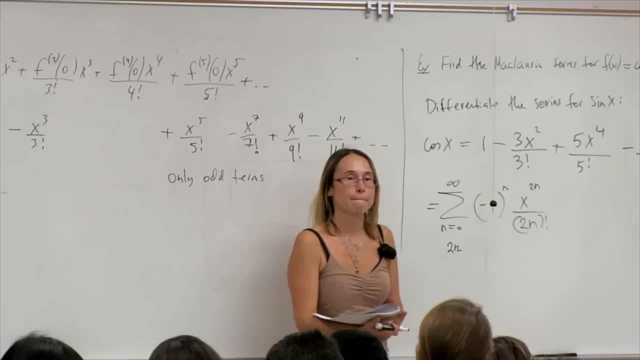 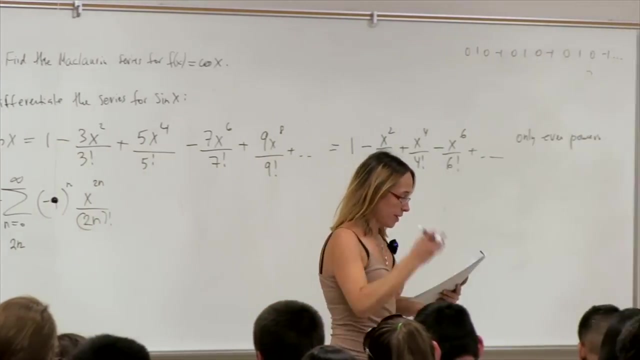 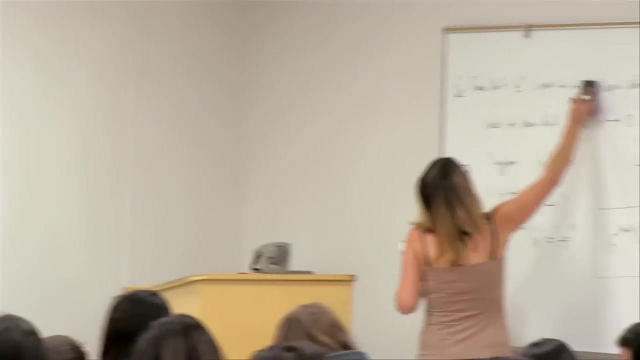 So I have x to the power of 2n Divided by 2n factorial. That only picks out the even terms Questions. Very good, Fine. Another important series Which will do the usual method. By usual I mean that we're going to write down all the derivatives. 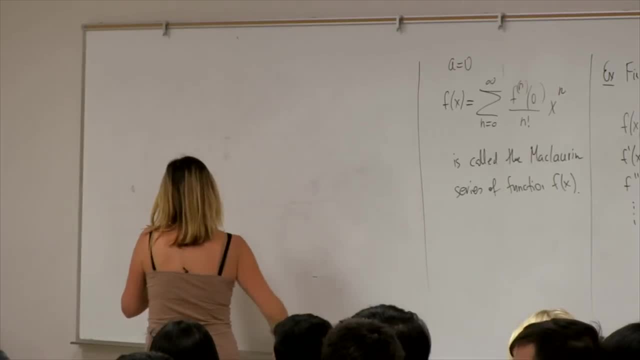 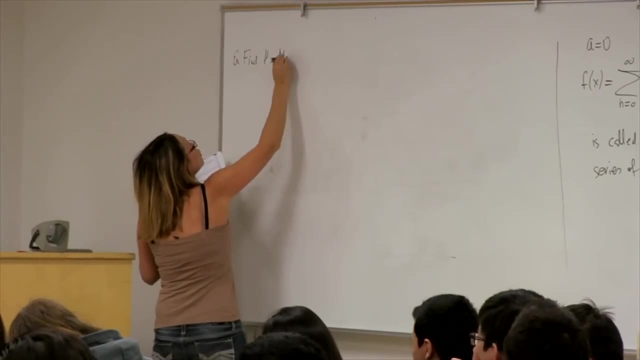 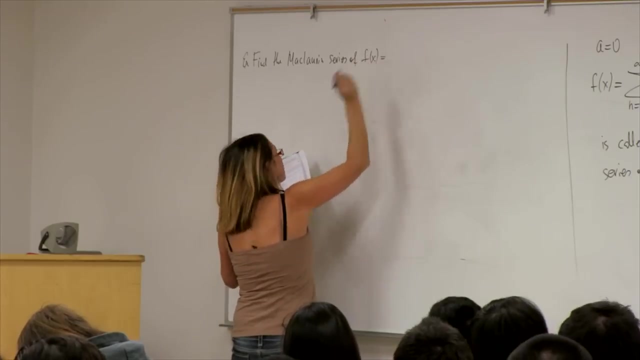 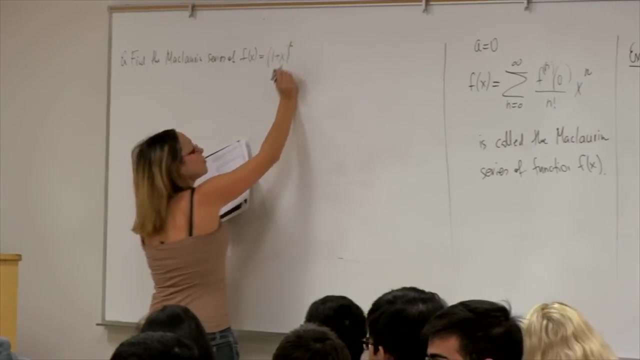 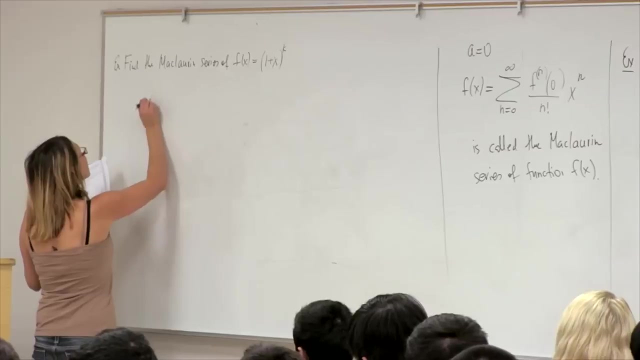 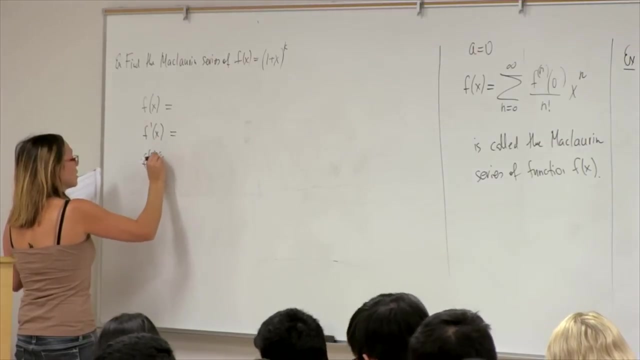 And evaluate them at the center. So find the Maclaurin series of the function f of x, Given by 1 plus x to the k, Some power of k. Okay, So I'm going to need f of x. 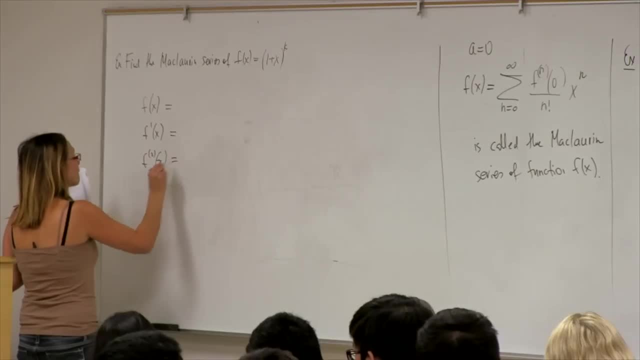 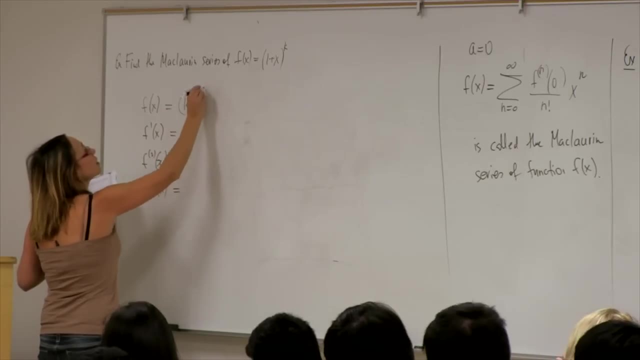 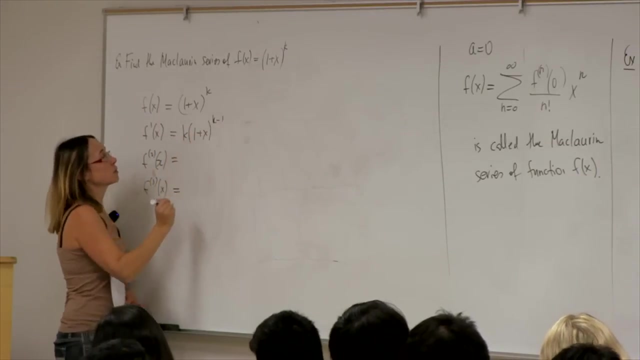 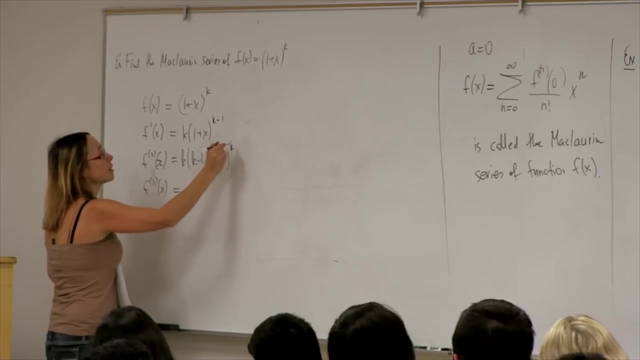 All of these, So 1 plus x to the k. This is my given function. The first derivative is k 1 plus x- k minus 1.. The next one is k- k minus 1.. 1 plus k. 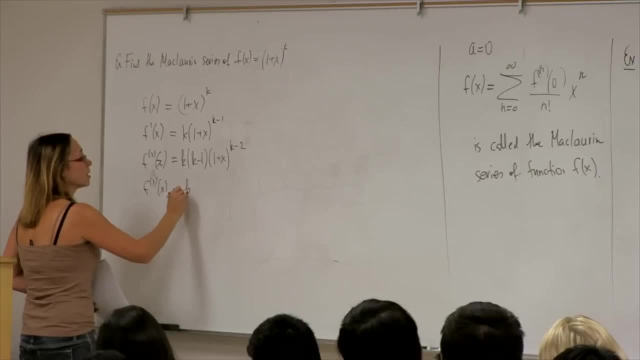 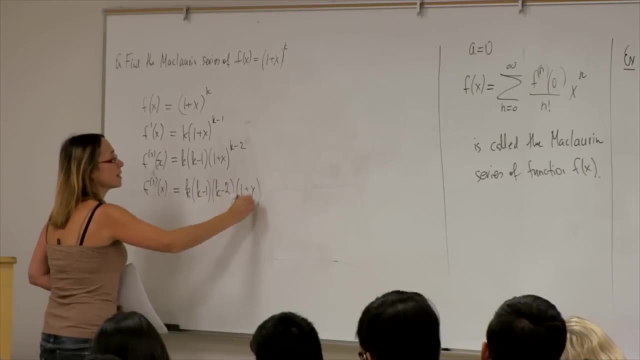 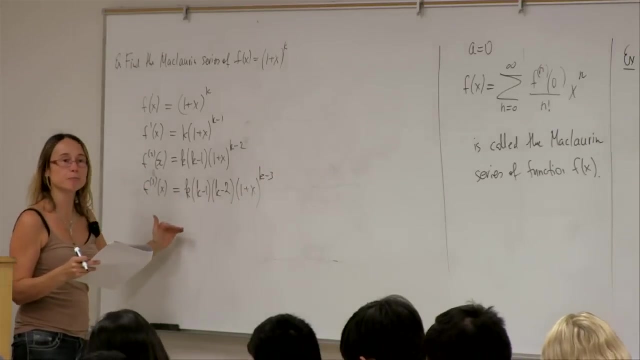 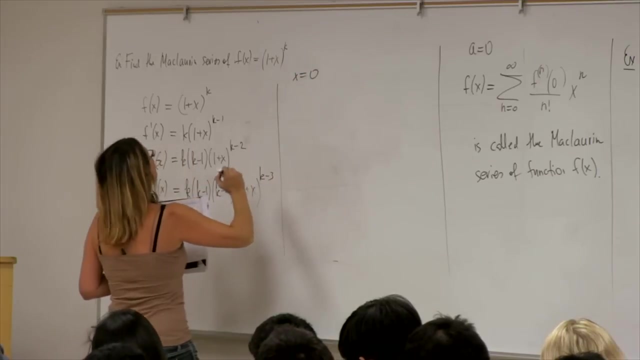 k minus 2.. k? k minus 1.. k minus 2.. 1 plus x, k minus 3.. So I think we can see the pattern here Right, And it's especially transparent when we evaluate everything at x equals 0.. 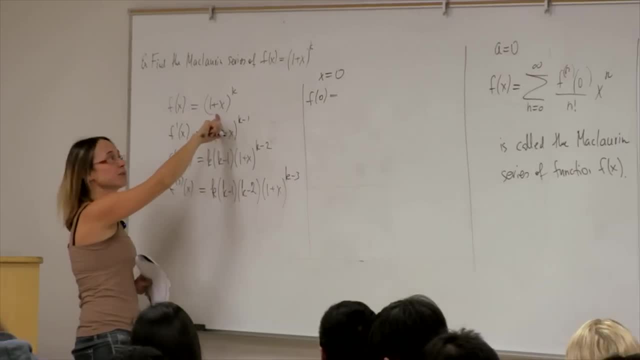 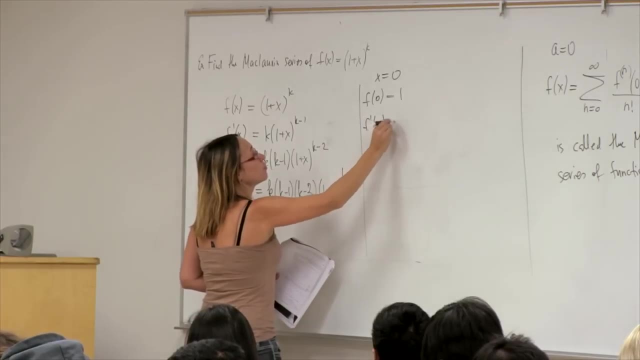 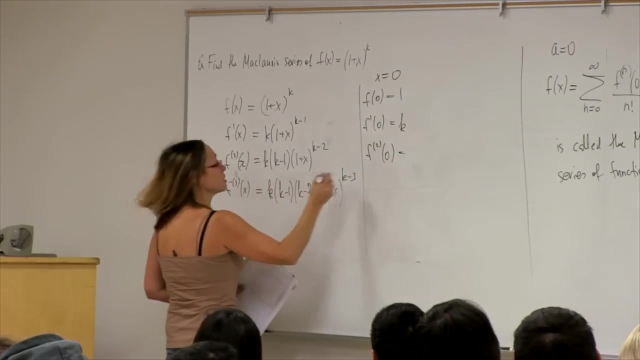 So what is f of 0?? You can see that this is 1.. Right, When x is 0, this is 1 to the k is 1.. f prime of 0 is given by k. The second derivative is k. 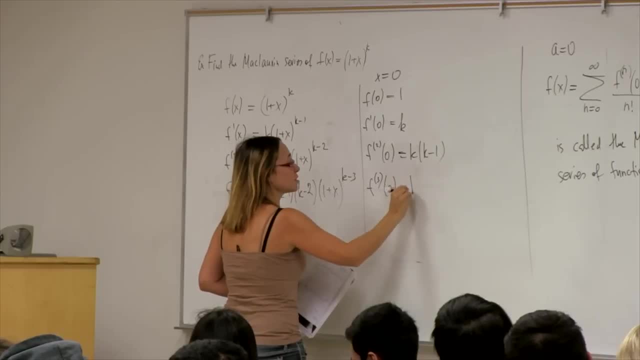 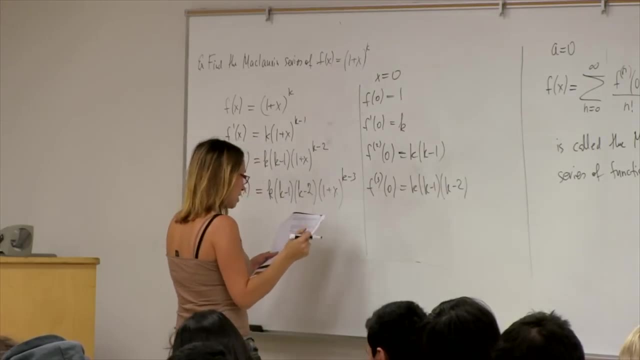 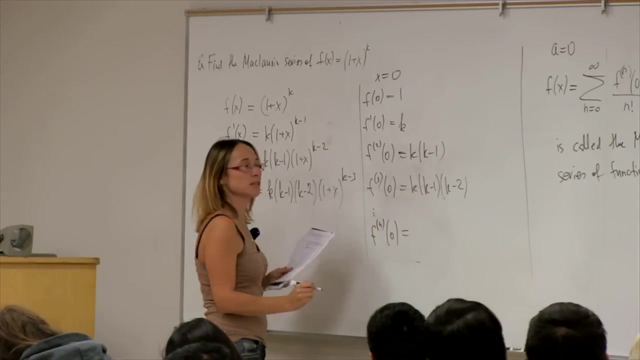 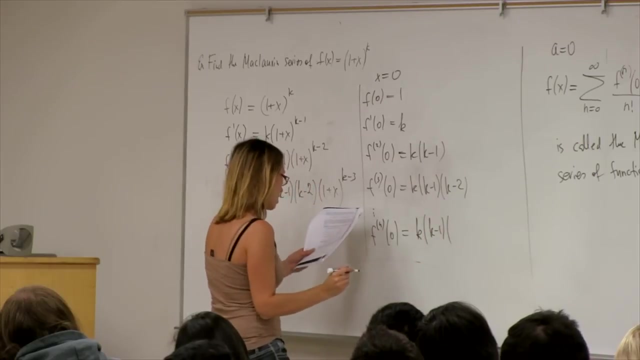 k minus 1.. The third derivative is k k minus 1.. k minus 2.. And so on Right. What's the nth derivative? What's the nth derivative? We're going to have? k k minus 1.. 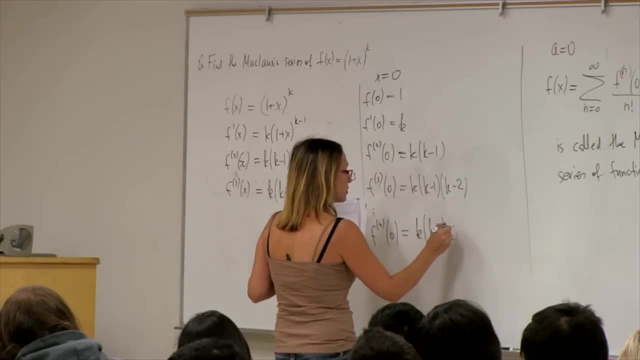 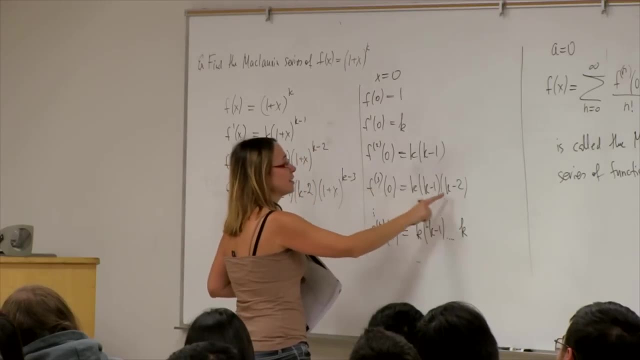 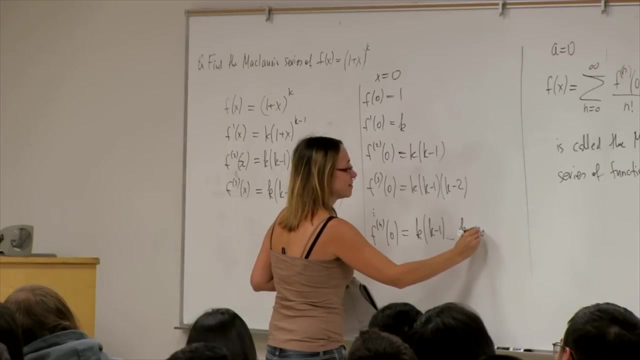 And so on, All the terms. What's the last term? k minus 1.. Are you sure This is f3.? The last term is k minus 2.. k minus 1. Plus 1.. Yes, Okay, Like this. 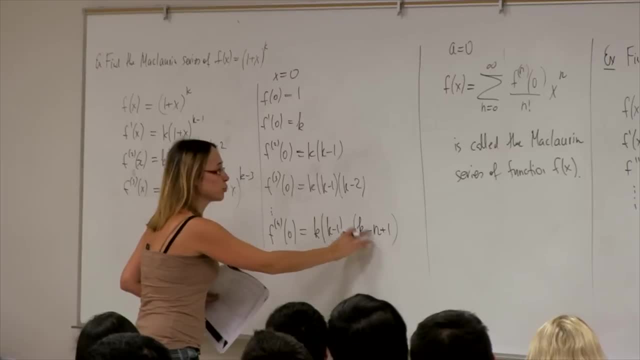 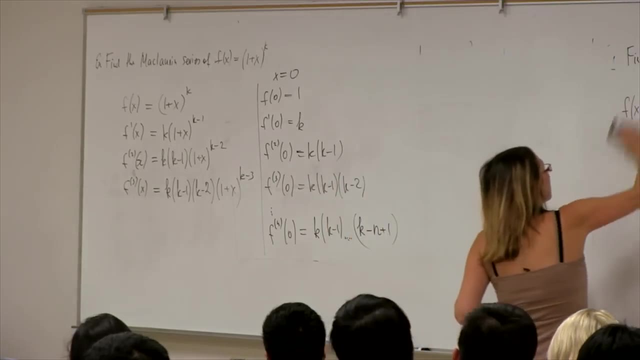 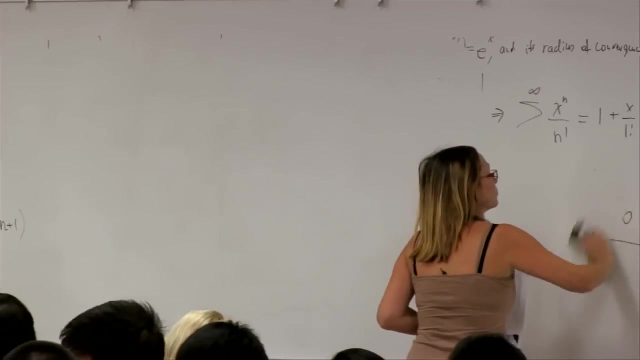 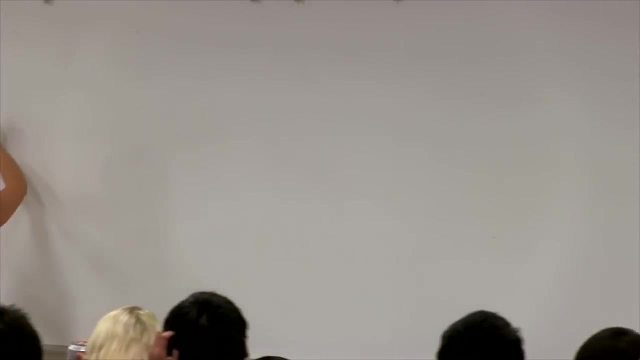 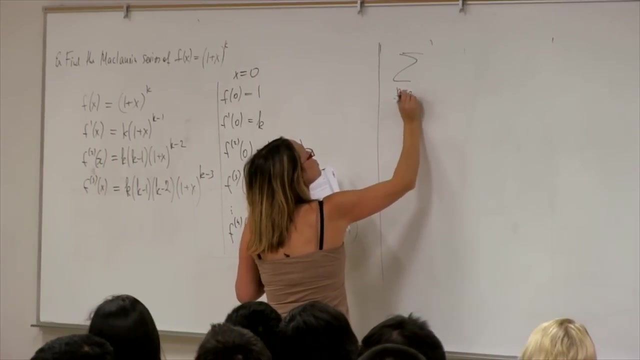 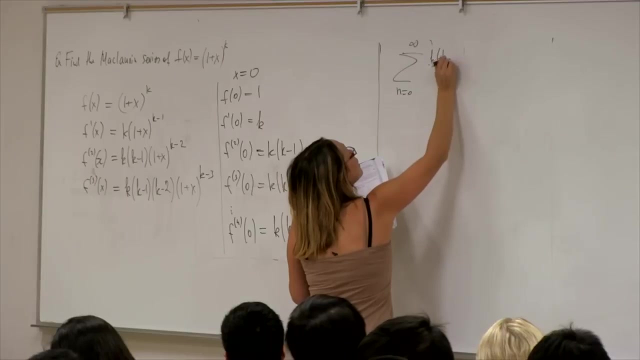 So Because subtracting n would subtract too much, So I need to put one back. Fine, So we can write down the series Starting from 0.. The general term is k- k minus 1.. k minus n plus 1.. 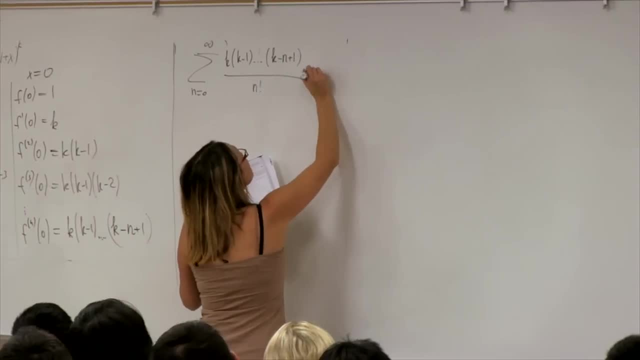 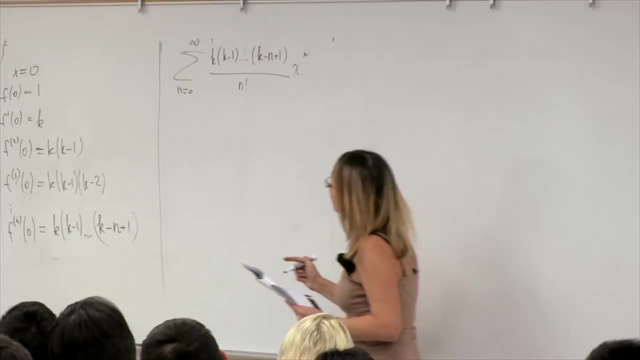 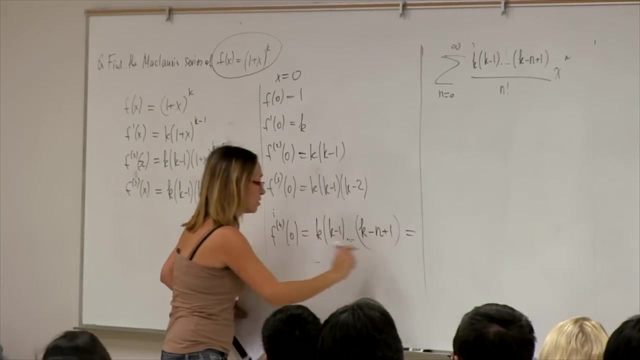 Dividing by n factorial x to the n. This is the general expansion, The Maclaurin expansion, of this function. So I want to give you a better way to write this. Okay, You can see that what you do here is you multiply all the numbers. 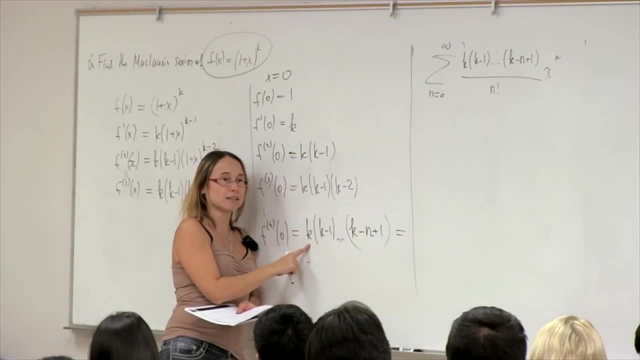 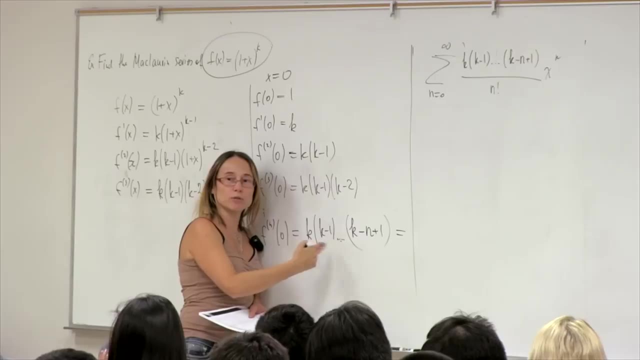 Starting from k and going down. So, for instance, if k was equal to 10,, you'd have 10,, 9,, 8, and you stop at some point, Right. So there's a much better way of writing this. 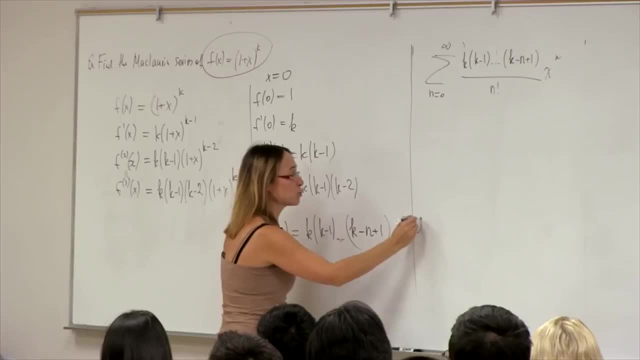 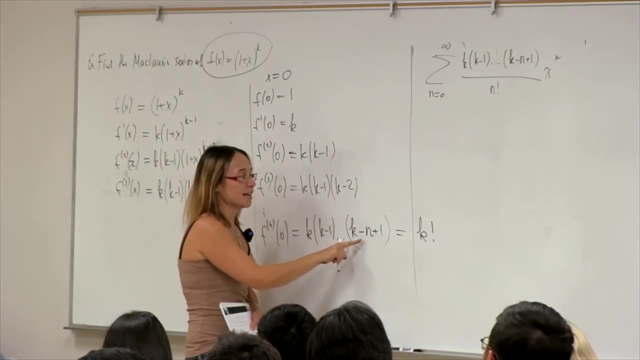 So if I went all the way down to 1, this would be equal to k factorial Right If I went all the way down to 1.. However, I stop. And starting from k minus n. starting from k minus n- I don't have these terms here. 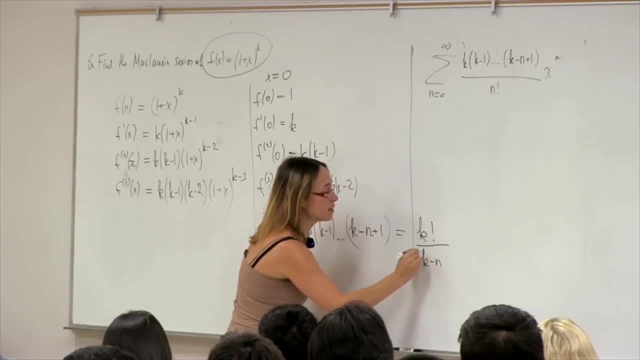 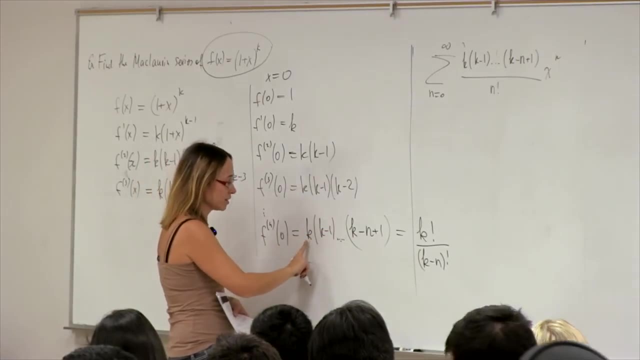 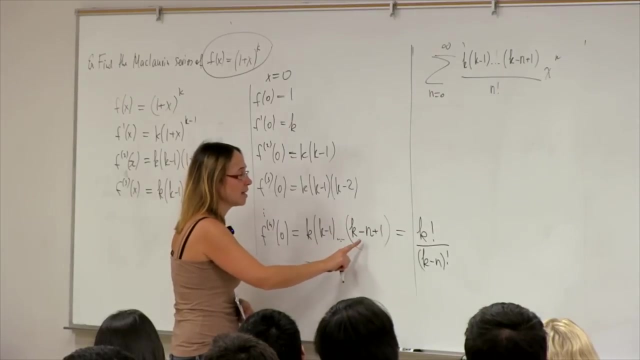 So if I put in the denominator k minus n factorial, that's what this is Right. So I have all the biggest multipliers And I multiply them together: 10,, 9,, 8.. And then I have to stop. 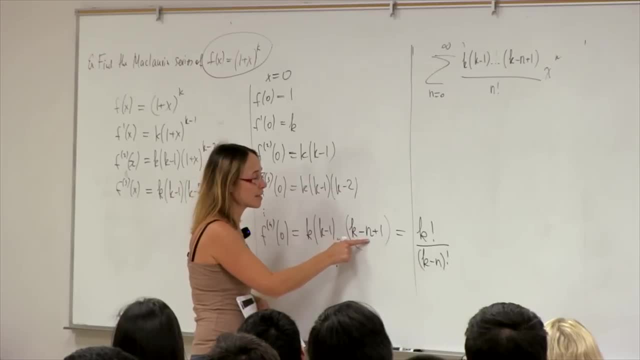 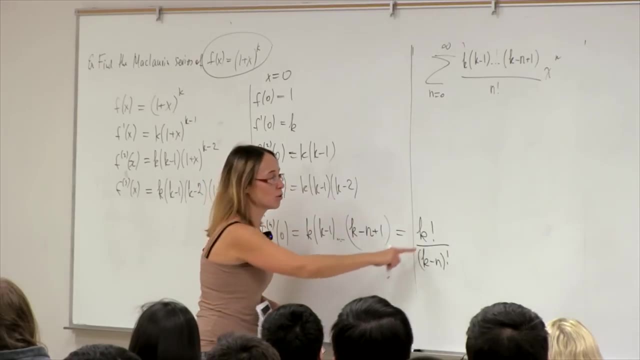 Where do I stop? The last term I include is k minus n plus 1.. The first term that I exclude is k minus n And everything down below from that. So this gives me the equivalent representation in terms of factorials. Okay, 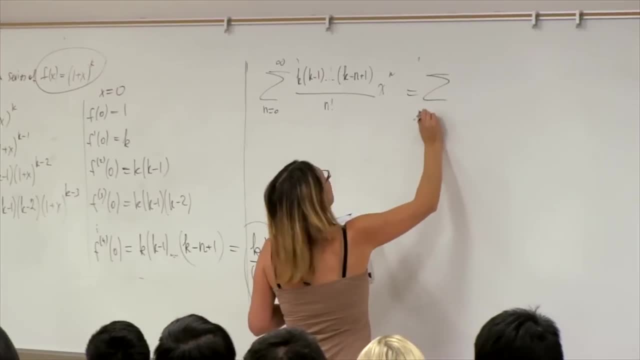 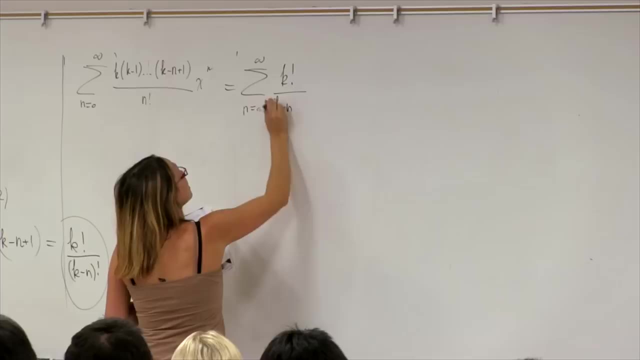 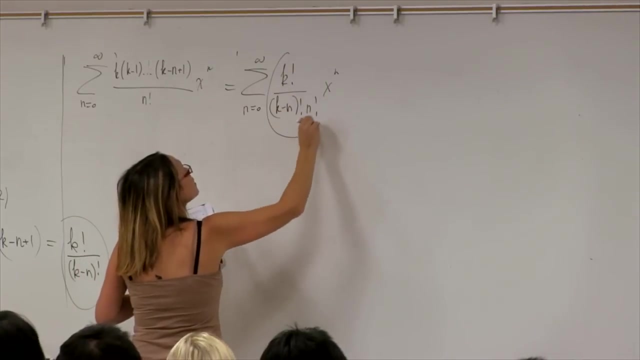 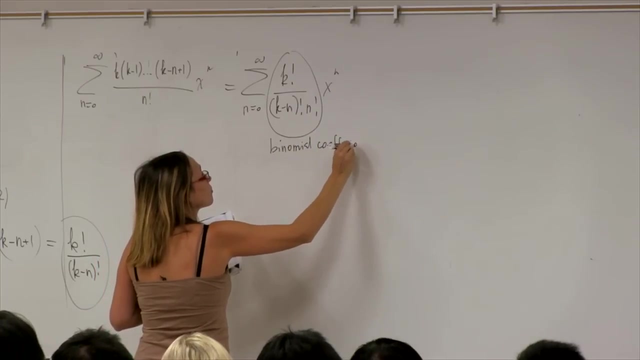 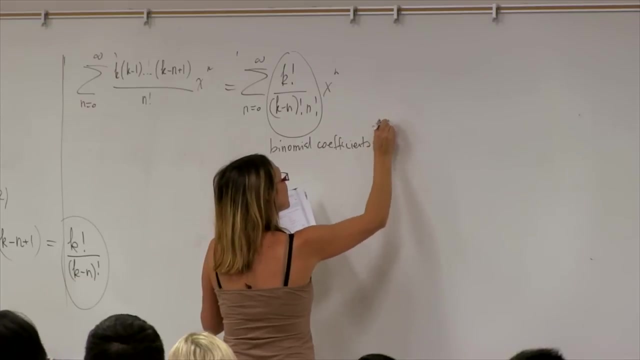 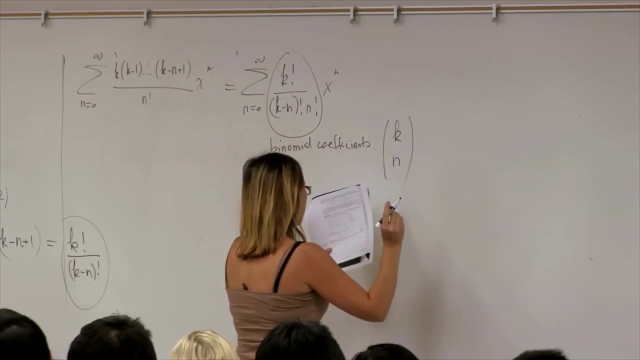 So this allows for a nicer representation here. So I have k factorial k minus n factorial n. factorial x to the n, And these things are called binomial coefficients And there is a notation for them. It's called k choose n. 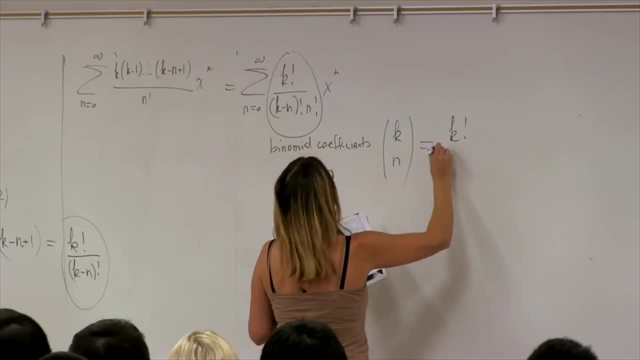 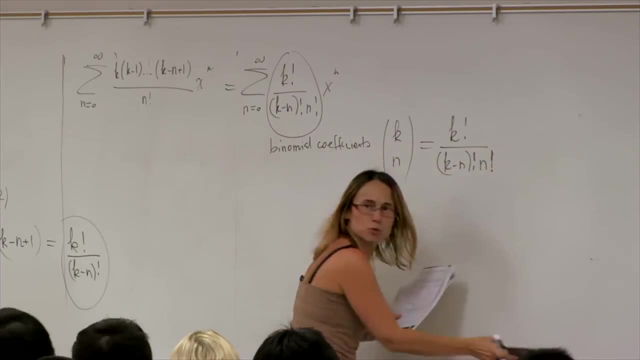 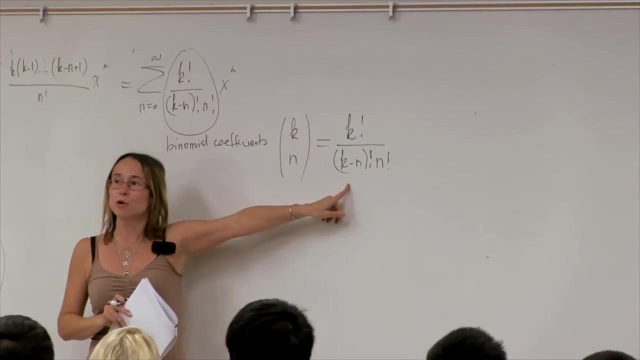 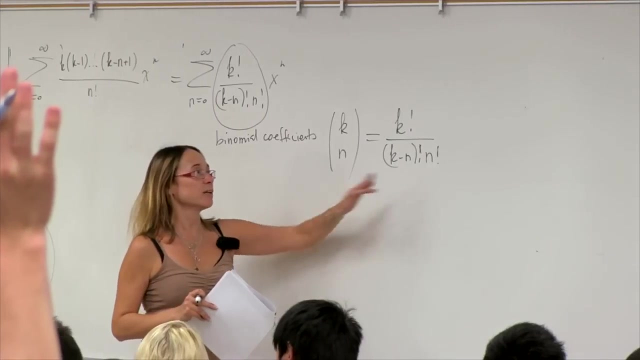 Okay, So this is a notation that means exactly this. What's this music? Okay, If you're familiar a little bit with combinatorics, that tells you how many ways you can pick. If we have k students in the class and I want to pick a group of n, this is how many. 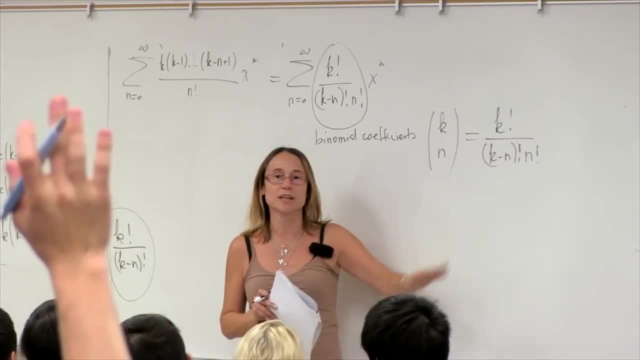 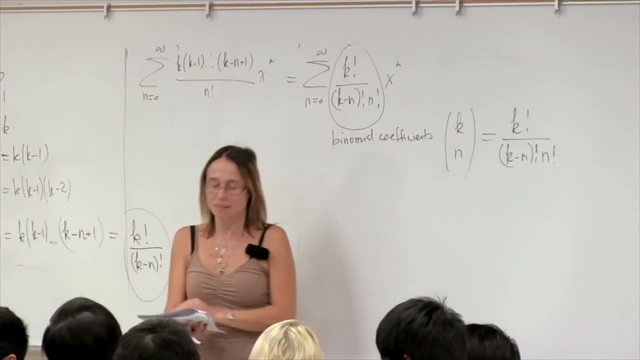 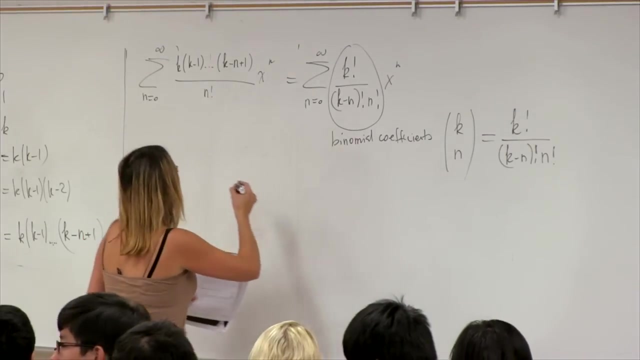 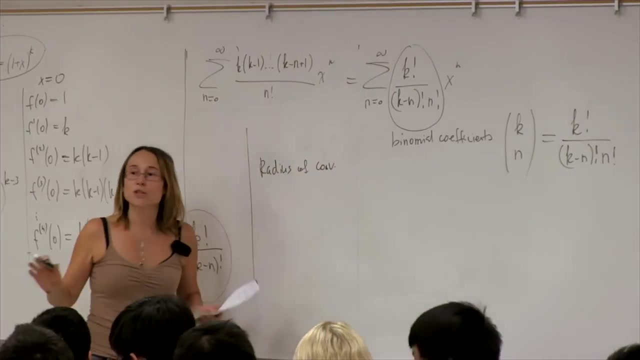 different ways I can pick n students out of k Question. It almost doesn't make sense because we have two minutes left. Yeah, Okay, So the last. let's talk about the radius of convergence really quickly. Question to you: How do I evaluate the radius of convergence of any power series, including the chlorine? 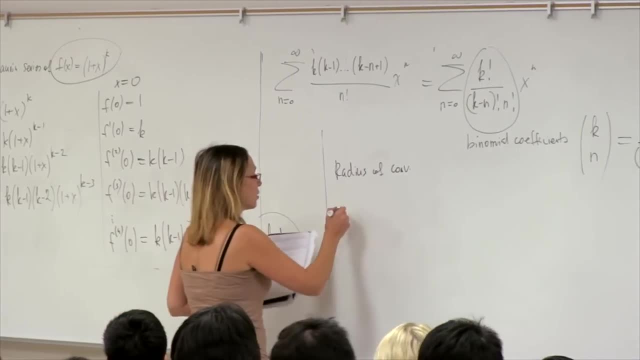 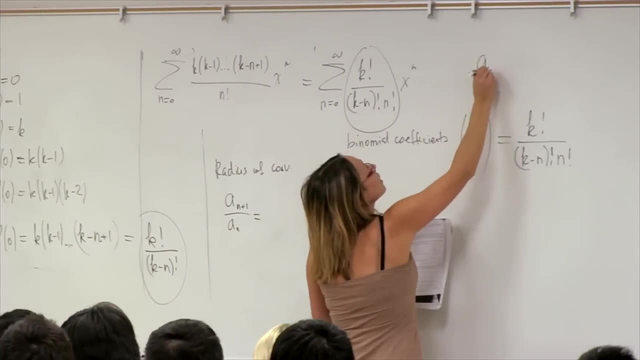 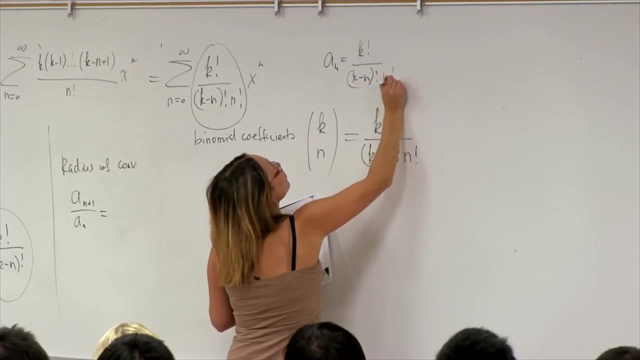 series. What do I do? What is the method? Ratio test. Okay, So a n plus 1 over a n I take. so what is a? n? A n is k factorial over k minus n factorial n factorial x to the n. 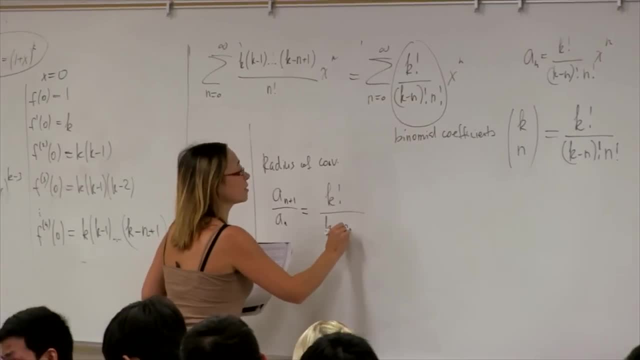 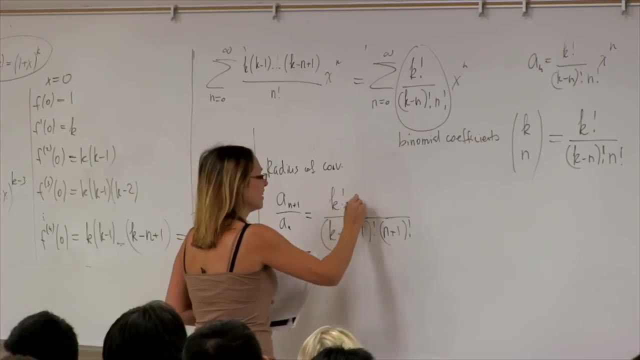 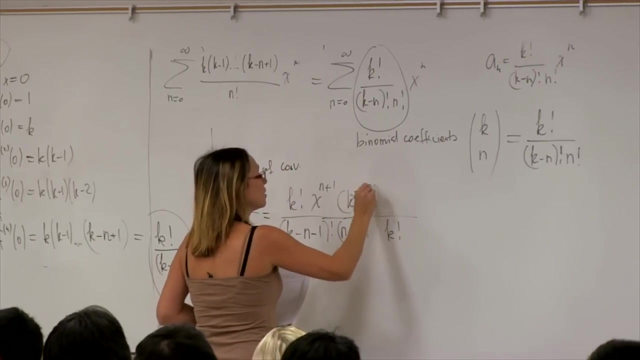 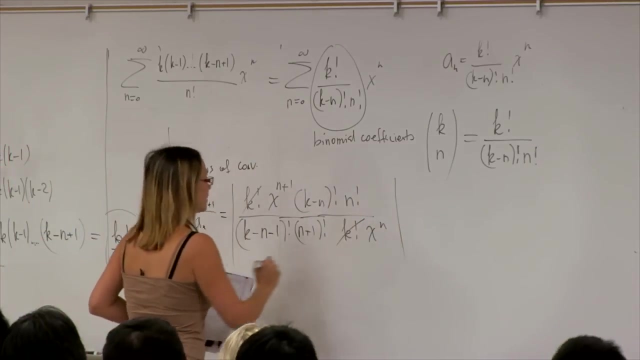 k. factorial k minus n minus 1. factorial n plus 1.. Is it getting louder? Divided by k. factorial k minus n. factorial factorial n. factorial x to the n. So look, we have lots of cancellations. x remains only here. 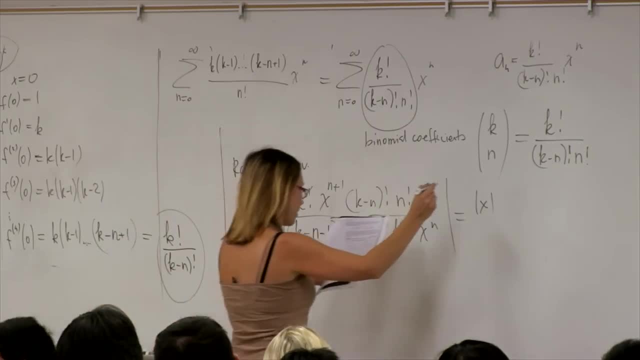 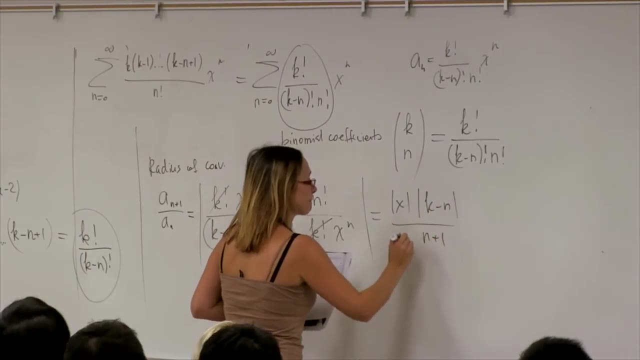 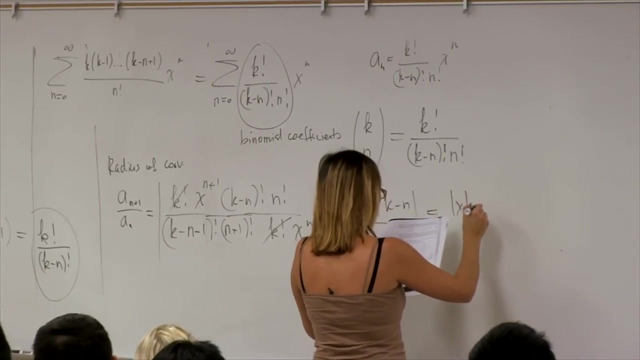 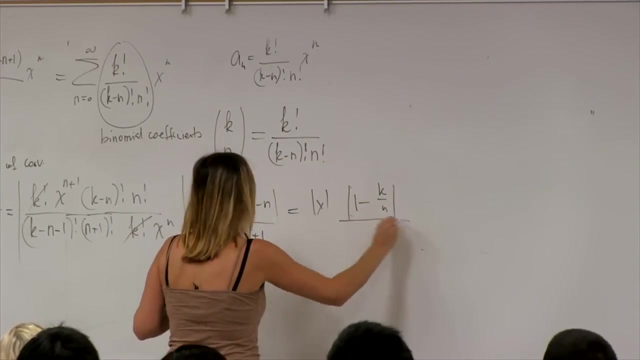 k minus n. factorial k minus n minus 1.. So I have k minus n And I have n plus 1.. Okay, So I can write it once more like this: 1 minus k over n, divided by 1 plus 1 over n. 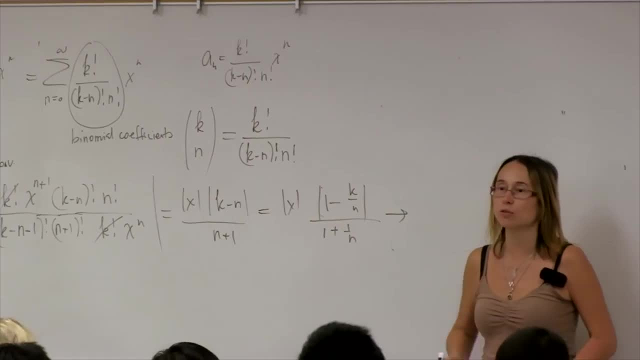 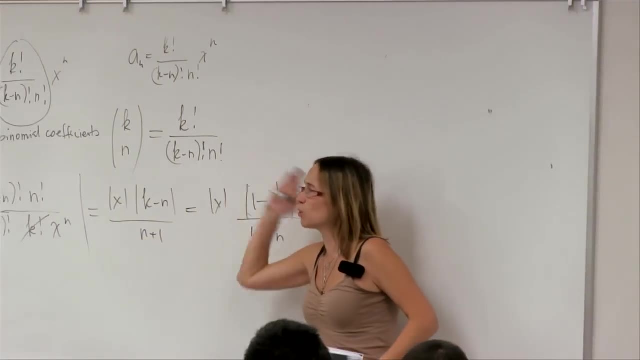 Okay. So what is the limit of this, as n goes to infinity? So before, when we did it for exponents, we had x divided by n, factorial, And that always went to 0. This one, as you can see, doesn't go to 0. 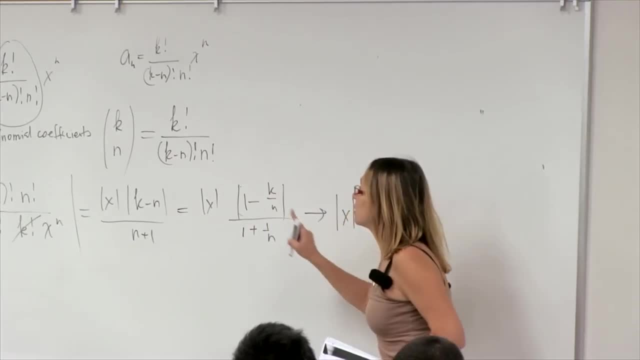 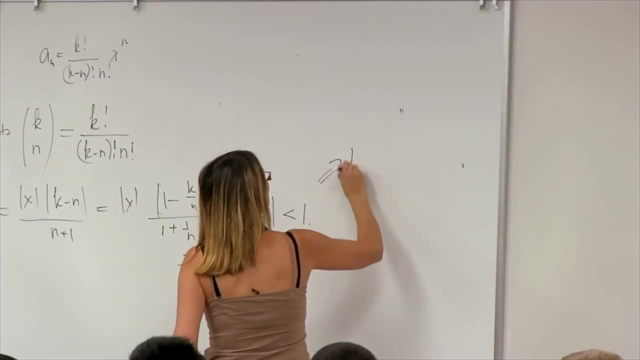 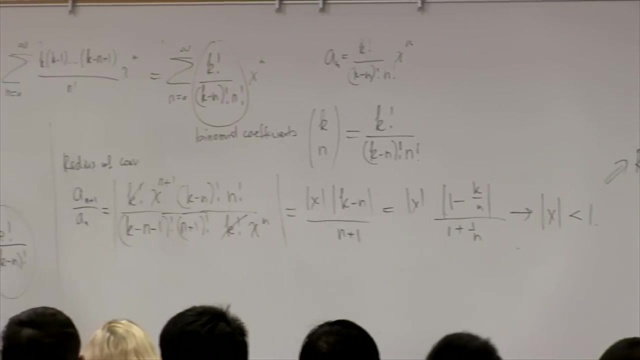 But it goes to x factorial. So the ratio test tells us that the series converge only when this guy is less than 1.. So the radius of convergence for Maclaurin series is 1.. So we have this nice representation of this function for the values of x, between minus 1 and 1 only. 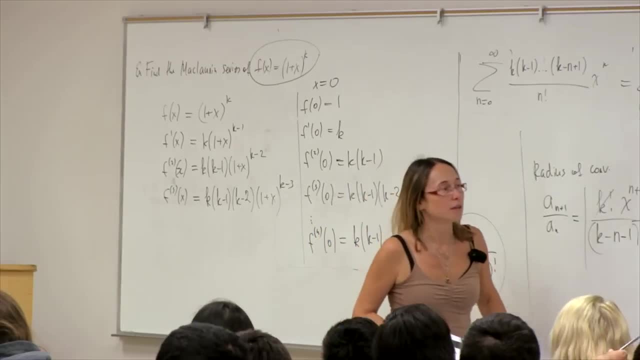 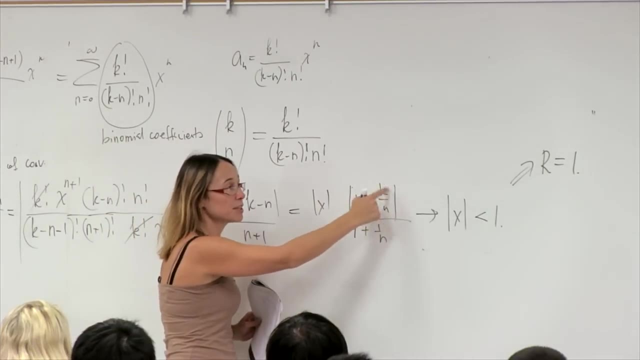 Questions. So 1 minus k over n, You have to find the limit of that right. So, yes, n goes to infinity. So this guy goes to 0.. So I have 1.. This goes to 0.. So I have 1. And x remains. Thank you. 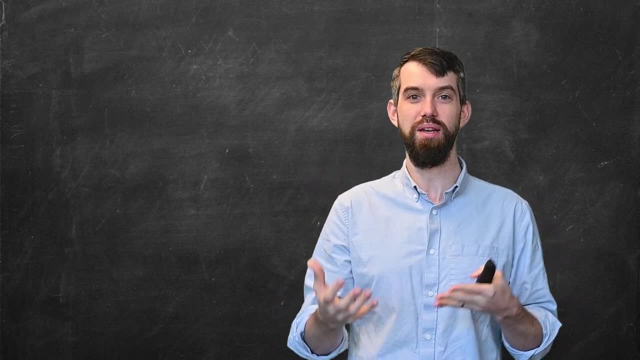 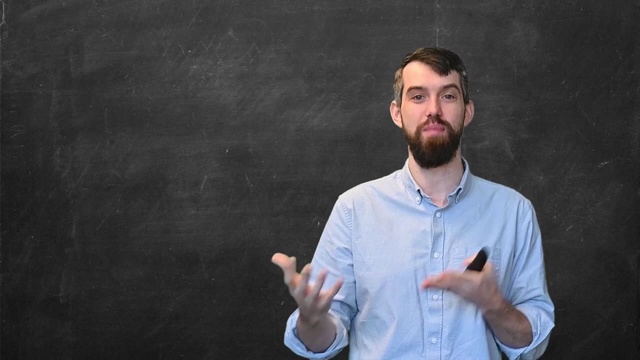 Welcome to my new series on the Laplace Transform. In this video and the videos going forward, we're going to study some of the reasons why the Laplace Transform is an incredible, powerful piece of mathematics. In this first video, we're going to define the Laplace Transform and we're going to 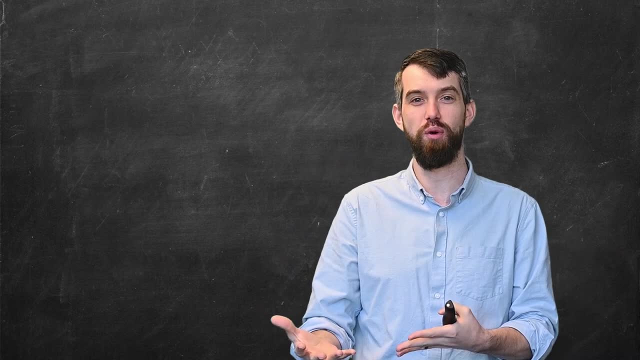 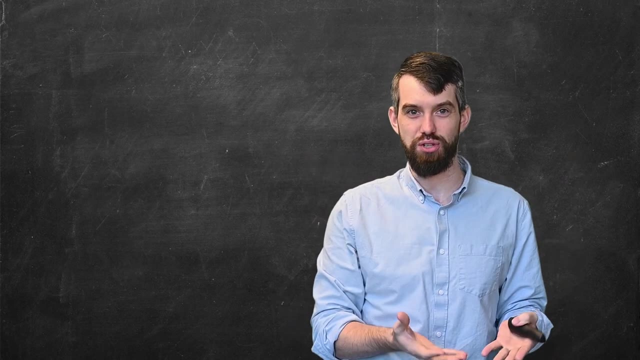 see a couple different examples where we're going to compute the Laplace Transform. But why might we be interested in something called a Laplace Transform in the first point? One reason why I really like the Laplace Transform is it's useful for solving differential equations like this one.